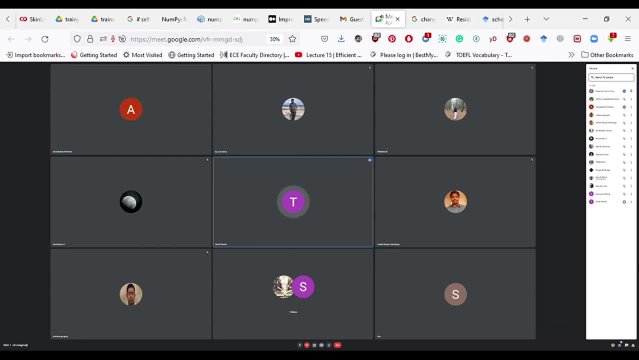 So thank you all for showing interest in today's talk And, on behalf of the IEEE Signal Processing Society student branch IIT Kharagpur, I welcome our guest for today's session. So let me introduce today's speaker, Dr Akanksha Pathak. 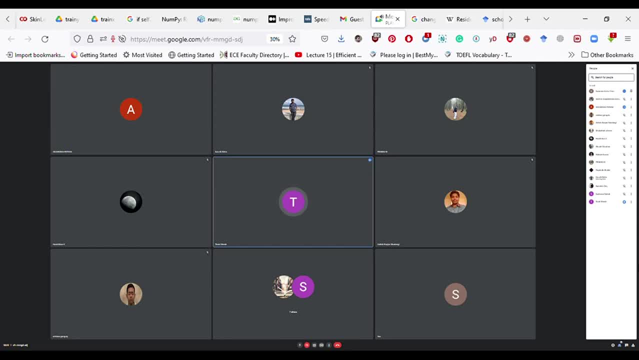 She has been working recently as the principal engineer at US-based semiconductor manufacturing company, Global Foundries. She has completed her guidance. She has completed her PhD from IIT Kharagpur itself under the guidance of Professor Gautam Shah from ECA department. 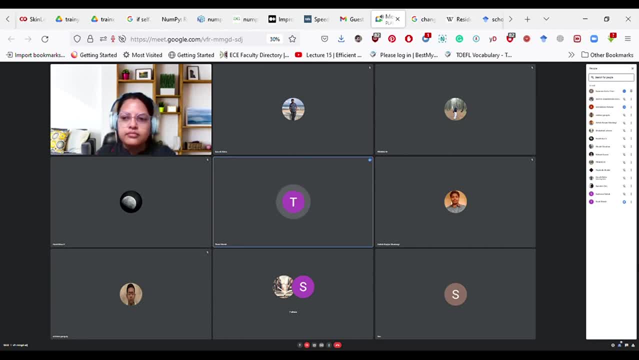 She has completed her MTech in Robotic Specialization from IIT Allahabad and her BTech from Uttar Pradesh Technical University in Electronics and Instrumentation domain. So her principal research interest lies in applied machine learning, deep learning in biomedical signal and image processing. 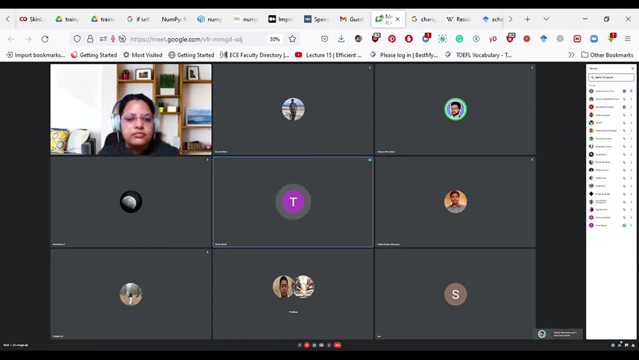 So, without further delay, I just want ma'am to begin with her session on the different methods for biomedical signal and signal processing using machine learning, methods for cardiac disease detection using the heart sounds. So I just request everyone to please kindly mute themselves and at the end please ask any question you have in mind. 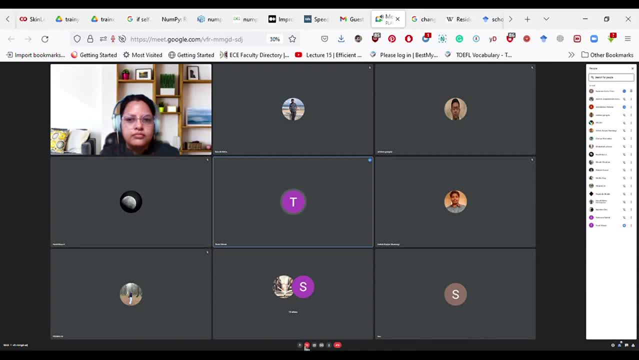 Ma'am is going to definitely answer the questions And please fill up your name in the attendance sheet. that would be provided in the chat box. So welcome, ma'am. Please continue with the session. Thank you, Tiyash and the entire IEEE SPS society. 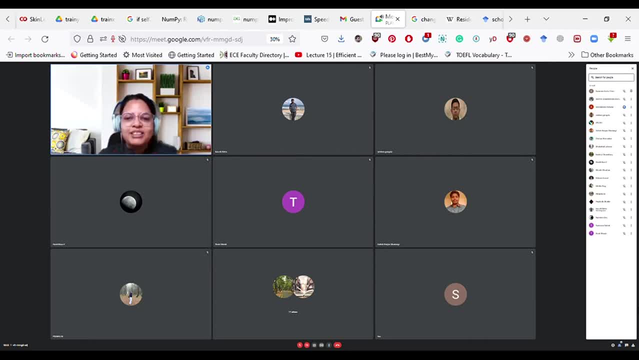 It is indeed a pleasure to be here as a speaker when I myself was a part of this organizing committee. So yeah, it's all together a new experience, So let's start with it. So is it full screen available? Yes, it is. 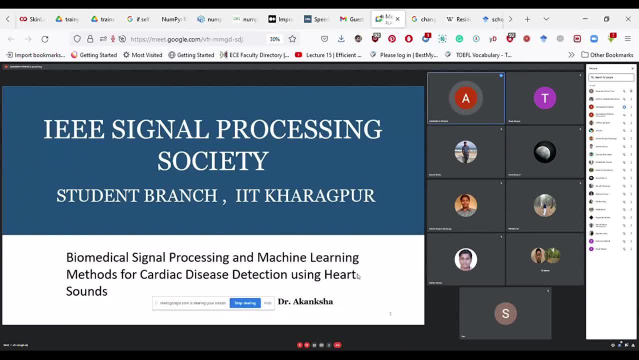 Okay, So good evening everyone. My name is Akamsha and I'll be presenting today's the SPS Signal Processing Society student branch talk. So the topic of this talk is basically biomedical signal. So the topic of this talk is basically biomedical signal processing and machine learning methods for cardiac disease detection using heart sounds. 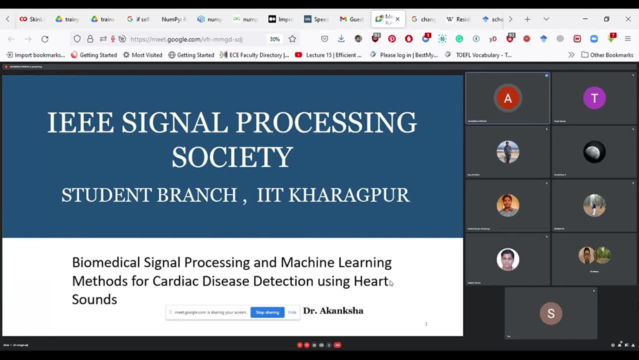 This work, or the talk, is basically based on my PhD work undertaken during my IIT Kharagpur tenure. So, though I have tried to make it like more based on intuition sense on how to deal with a biosignal based problem, but still like more the methods will be. 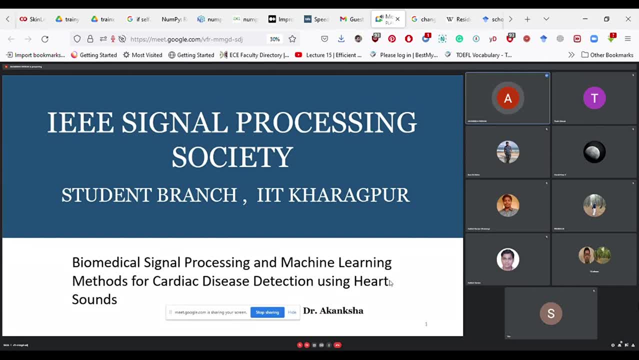 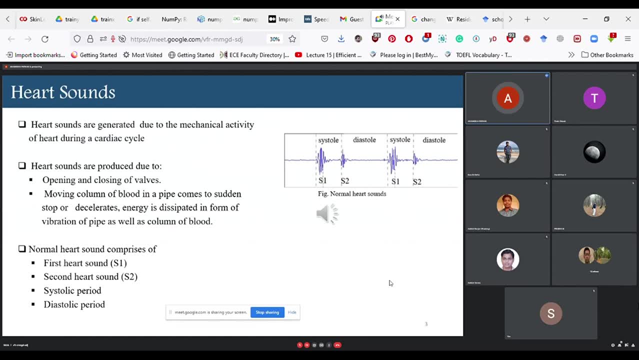 Truly like sometimes confined to other special disease which I will be dealing with here. So first is heart sounds. so what are heart sounds? I think we must have heard about the heart sounds either in a biobooks or through some Bollywood movies. 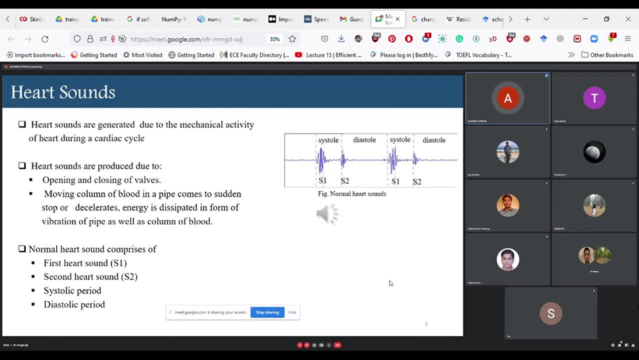 What do they appear like and how do we hear them? They are mostly like love dove, a sequence of loved over. um, let me play if it is good. okay, so hard sounds are basically generated due to the mechanical activity of the heart. mechanical activity basically means the 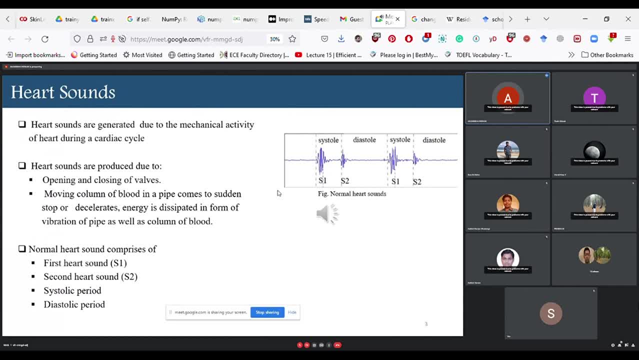 regular relaxation and compression and compression phase of this heart. basically, hard sounds are produced due to, if you can say, due to opening and closing of the walls, the four walls, if we remember the aortic mitral and the tricuspid and the pulmonary. another analogy which we can understand, that how hard sounds are produced is like suppose: uh, if you. 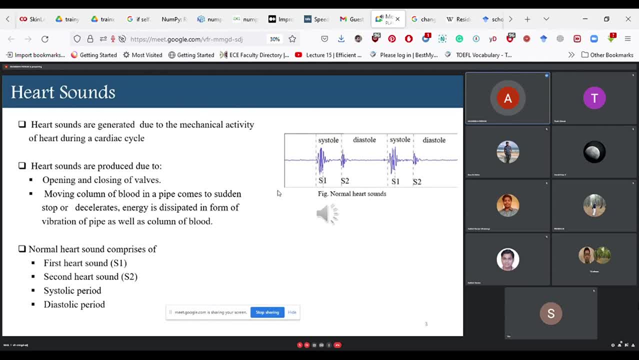 remember the, the water pipe through which we usually water our plants. if that pipe is stenosed or constricted or obstructed at some point, then you might hear some sounds of sound or you might feel the vibration in the pipe due to that constriction, if the pressure is too too much in the water pipe. so similar is the case. 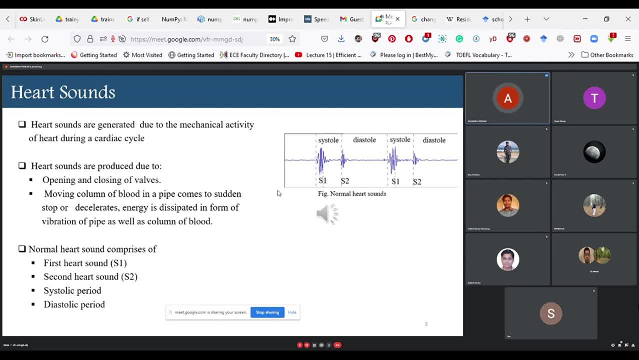 with the heart sounds. whenever the blood offers or obstruct is obstructed in the vessels in any form, due to stenosis or other obstruction, then what happens is the energy is dissipated, either in form of vibrations. vibration is something which is not audible, and when it is an audible frequency, 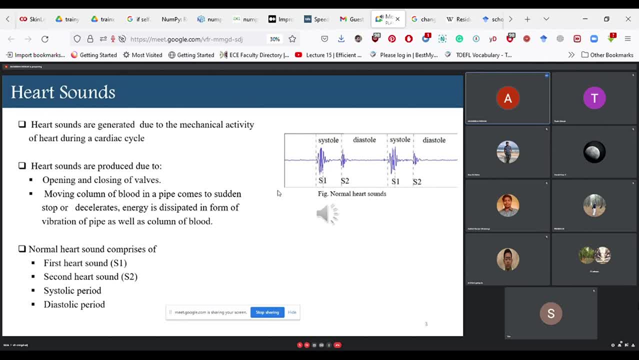 it is heard as a sound or a murmur, whatever we term it as unwanted noises or the abnormalities are termed as murmurs and healthy sounds. healthy activity is termed as sounds, heart sounds, and if it is not at all audible, we term it as just vibrations, so normal. 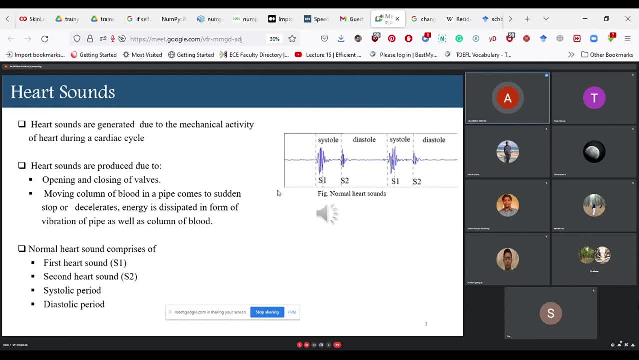 heart sound basically comprises of four main phases. first is the s1 sound, the this sinusoidal wave. then next is the silent phase, systole. next is the s2 sound, uh, the dub sound, which we say and then are comparatively longer, but again a little bit silent with diastole. so this is a repetitive. 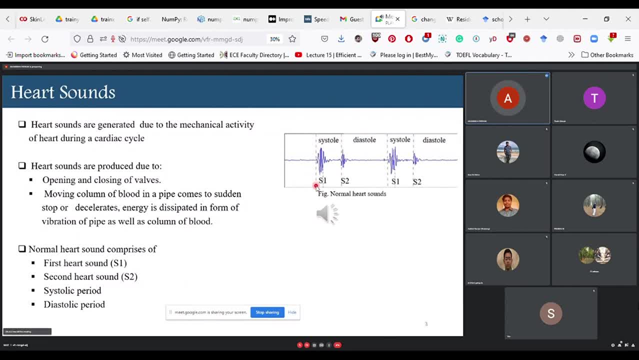 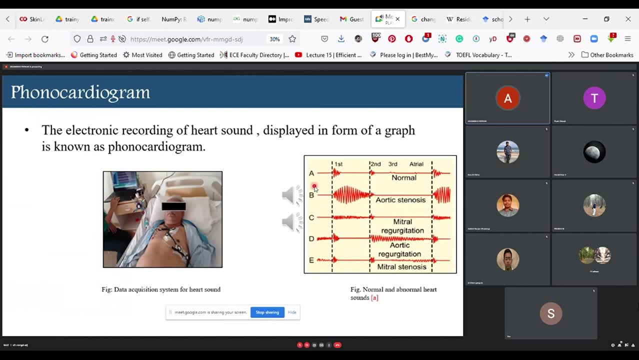 cycle. now, what is phonocardiogram? so you are using? you are using the terms as heart sound and we can only listen them using set of scopes. but how do we use those sounds to process it at our end? so the electronic recording of these heart sounds, which is displayed in form of a 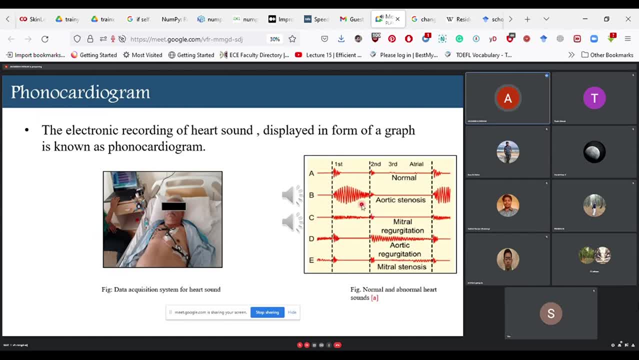 graphical pattern, as shown in this figure, is known as a phonocardiogram. so, as we can see this figure, this figure is taken from our own data equation system, which i use in this study. so, basically, what we do is we attach some sort of transducer in the stethoscope to convert this sound into an, a digital. 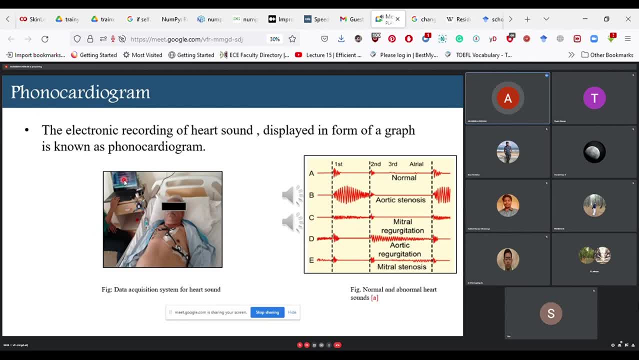 record and then it can be saved using some- uh, daily used softwares to record the heart sounds in form of and whatever file format you want, so that you can hear it as well as access it. so, as we heard a normal song, what would be a abnormal sound be like? so an abnormal sound would? 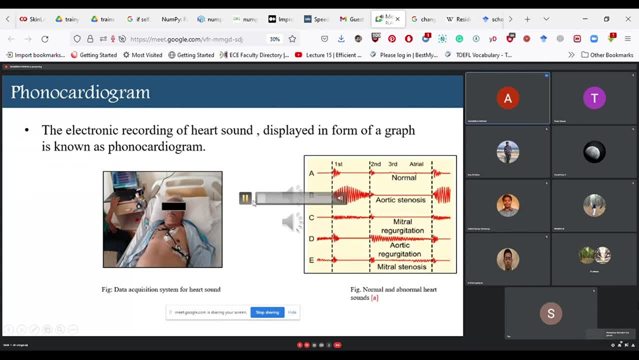 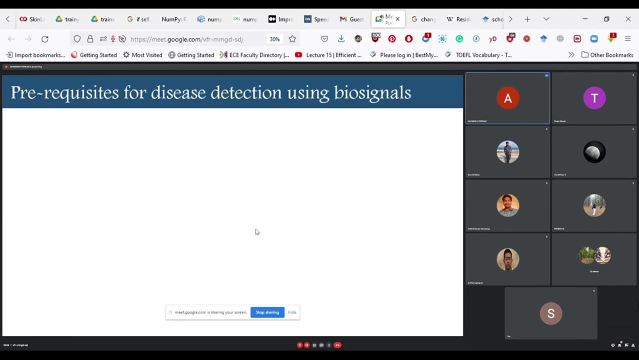 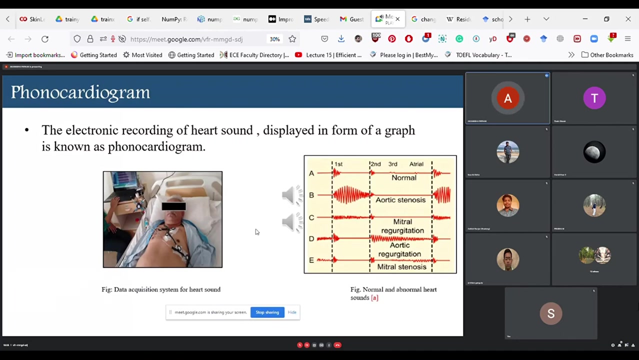 be like if you, i hope it is audible and this is for another abnormality, okay, so, um, just a quick go through. stenosis, basically something when the blood is unable to move in a forward direction due to the constriction, and resurgitation is something when the blood flows backward due to the improper closing of the wall. so stenosis is due to. 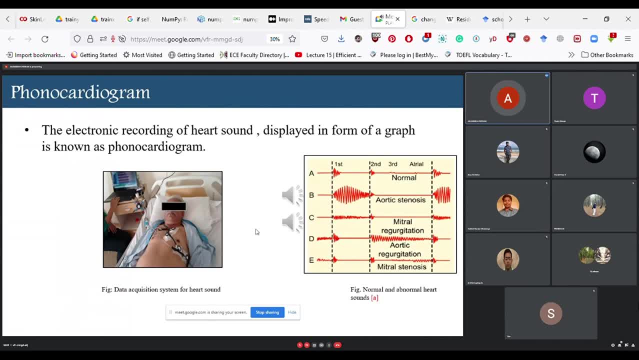 an improper opening of the valve and regurgitation is due to improper closing of the valve. valve can be considered as a sort of two phase door, which is unable to open and close which is able, which is whose opening and closing basically regulates the blood flow. what are the prerequisites? 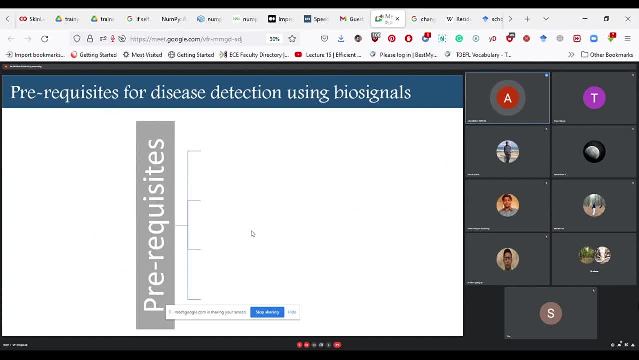 for disease detection using any biosignals. so this is like, i think, a mandatory check which you should, which one should go through before starting with any biosignal for any sort of disease detection. so first is understanding of the disease. you need to understand what is the basic disease, how is it affecting that organ, what is it like, how is it caused? what 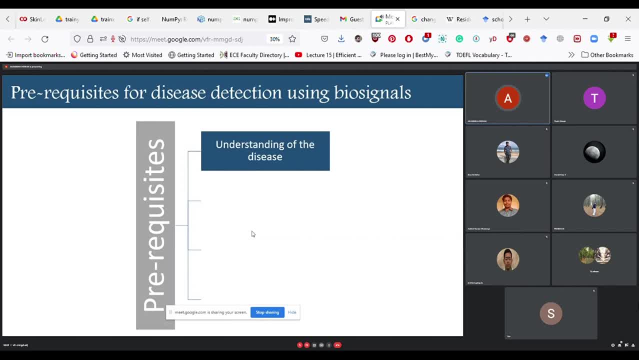 are the repercussions of it and so on, the statistics, how it is causing the mortality rates and all like you need to be aware of it. next is: how is the disease manifested in the biosignal so you are using? you are going to use a biosignal of your interest for diagnosing the disease. 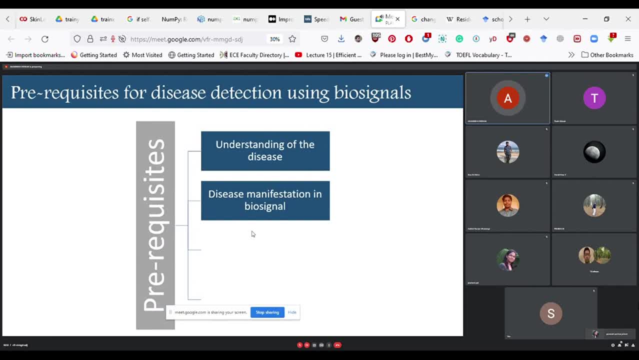 so, in order to go with your entire signal processing paradigm, you need to understand how is that disease manifested in that biosignal itself, starting from data acquisition, how is the signal going to be until you acquire, and how is that disease overall manifested in it. you need to know, then, what is the anatomy and physiology. 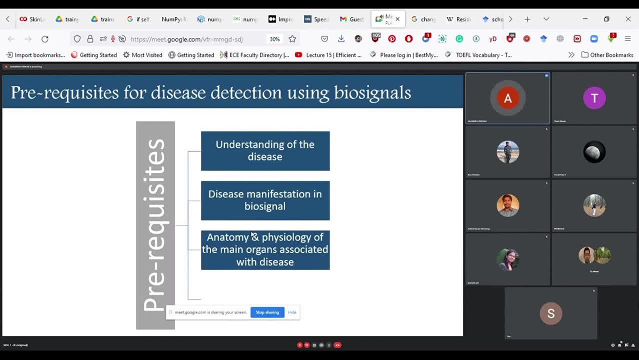 of the main organ assoated with the disease. so suppose you are. in this case i am dealing with heart, so i need to be aware what is the basic physiology of the heart then, how does it behaves after the disease, so that i can relate during my signal processing and i can. 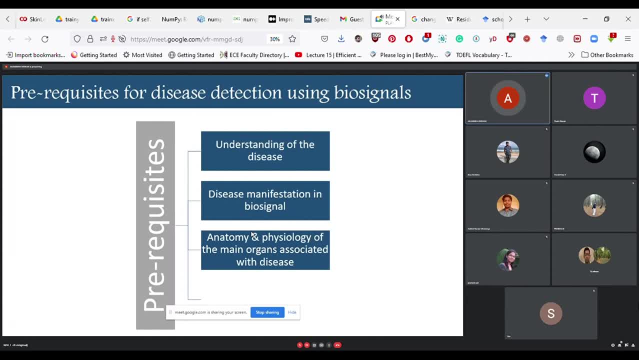 get an intuition. ok, so if i am thinking over this process, he is inspired because of this process in the anatomy and the physiology of heart. next and the last part, but not not vizot, credit to my sexual history, which had aaj locating the message at the bottom. so 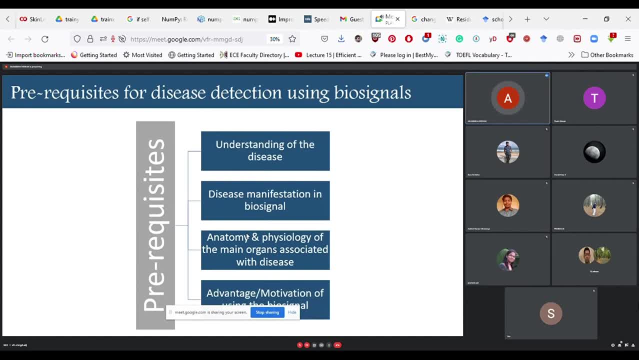 if you remember it says: pardon, i will be 음악 reader. maybe what you can pay with the info, because the performance of a manolary is inferred at key for every development. to figure outstreak the least is the: what is your advantage or motivation of using the biosignal? see, obviously. 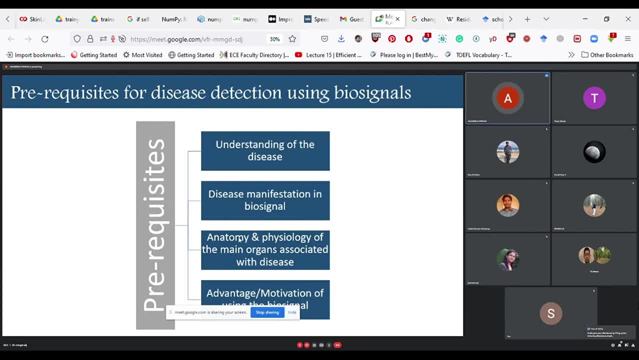 biosignals are not practically, or we can say commercially, used to a great extent because of the advanced techniques obviously, and one would obviously favor the advanced methods of disease detection rather than using the biosignal, because they are a little bit weak. but there should be some good motivation or advantage which you can portray in order to 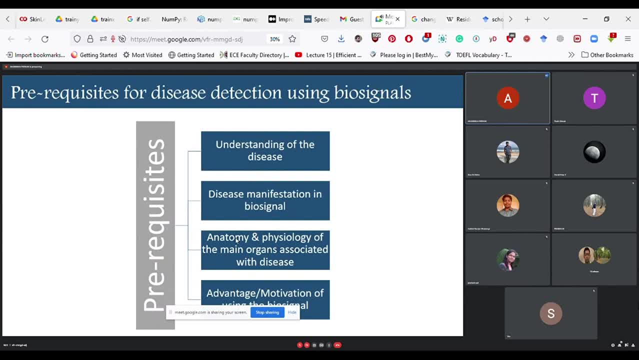 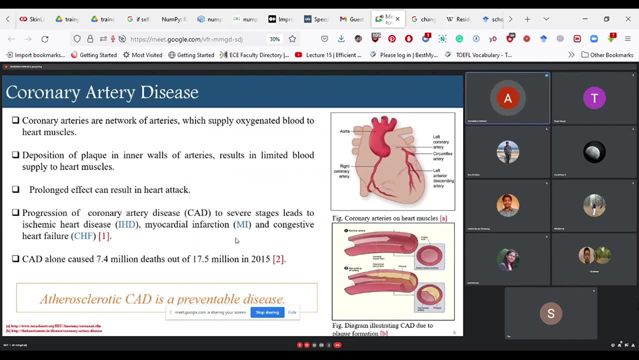 convince the society or the research group that okay. this is the main reason why i want to go with the signal. so just quick, go through here. in this talk today we will be dealing with coronary artery disease. so this disease, in layman terms you can refer to it as a sort of a heart attack disease. 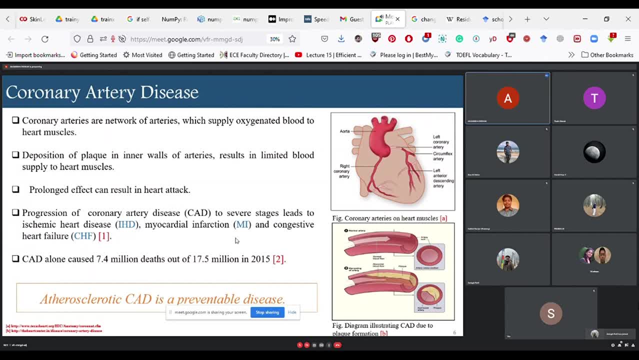 which we commonly know, and that the cholesterol buildup in these arteries, the coronary arteries, basically reduces the blood supply or the blood supply of the blood supply, of the blood supply, oxygenated blood supply to the heart muscles. so this is, as shown in this figure, this artery is not a single artery coronary artery, this is like a. 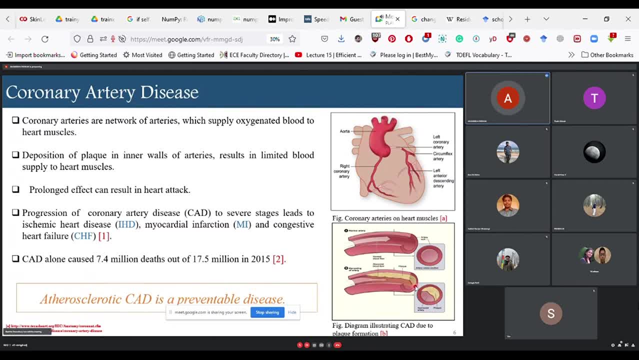 network of artery. okay, so, uh, as shown in this figure there, whenever there is a buildup of cholesterol- or, in technical terms, applied- and the inner walls of this artery, what happens is it limits the oxidative blood supply, so the blood supply is reduced to these heart muscles, which are 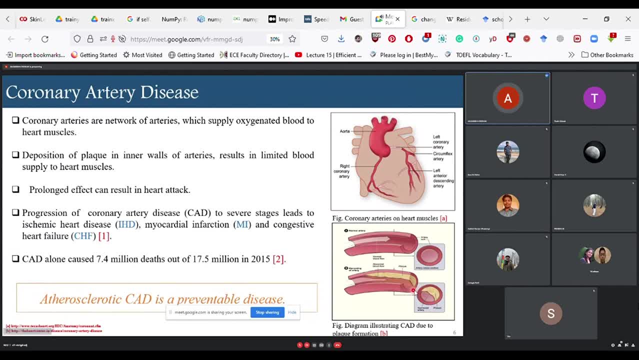 the heart muscles, which will gradually lead to the decay of the tissues of the heart muscles and hence the heart will lose its ability to contract and relax. so the disease is obviously very fatal, but it has a positive aspect that if it is identified it is at a good initial stage. it can be 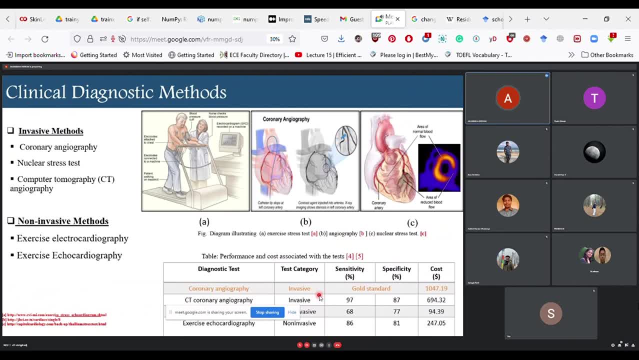 prevented to turn into more fatal. so there are some existing diagnostic methods which are like in the test, which in which the testing methods get intruded into your body and the ones which are not intruded are like non-invasive. so we have ct scans and some. 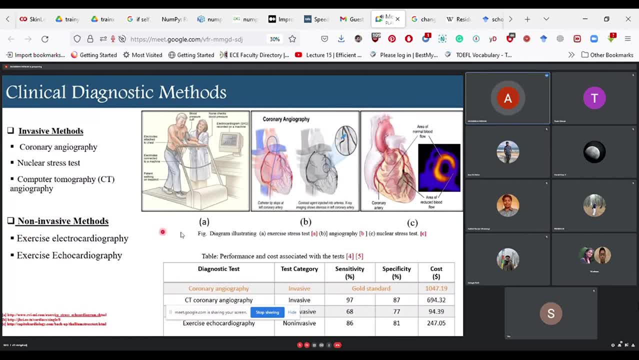 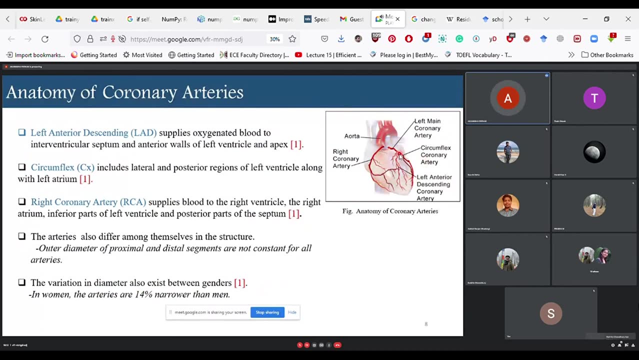 non-invasive methods like treadmill based ecg electrocardiography. so obviously, uh, we see like the gold standard is the angiography method. now a quick go through the anatomy. so anatomy is like it is not just a single artery but a network of artery, but so we have right divisions. 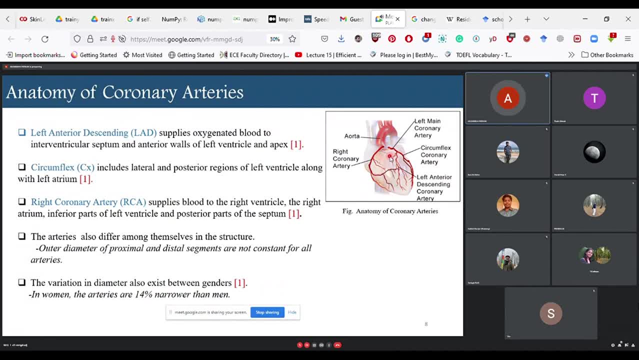 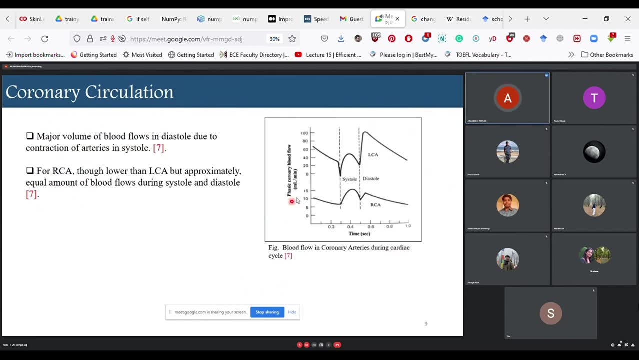 left division and then some common subdivisions of the left artery as well. now the arteries have. these arteries have different diameters among themselves also. moreover, the blood flow is also not like constant through all these arteries in both the phases. so, like you see, in one of the arteries, like left one, left coronary artery- blood flow is more in the 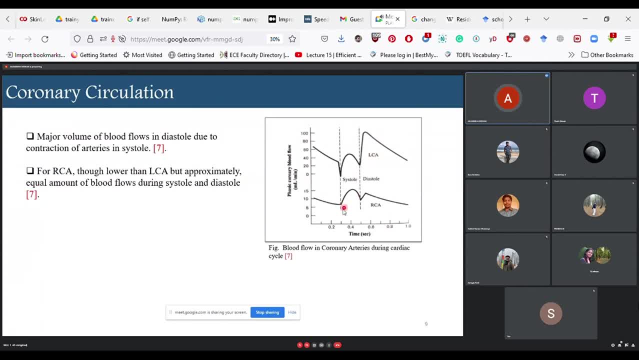 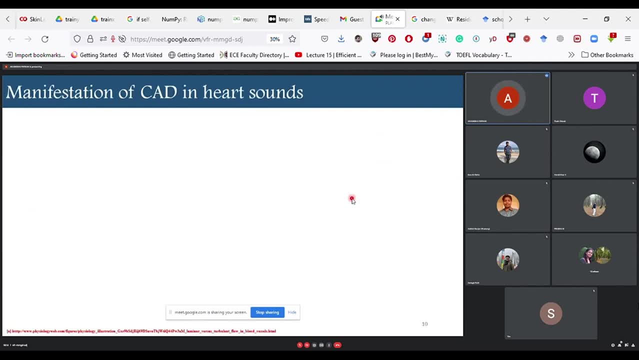 diastolic phase and less in the systolic phase and in the other artery approximately same blood flows in both the phases. now main thing is like how is the disease going to be manifested in the heart sounds. so this is like the main basic building block to understand how is your disease? 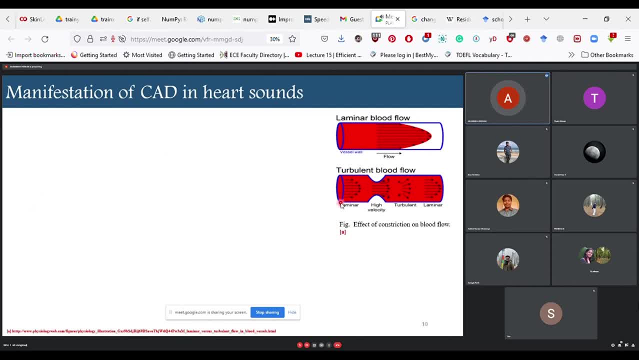 getting manifested so that you can think of in your case also, how is, how are you going to apply these methods? so whenever blood flows in a healthy vessel or a normal blood vessel, it follows a parabolic path. parabolic path means the particles at the center are moving in a more higher speed. 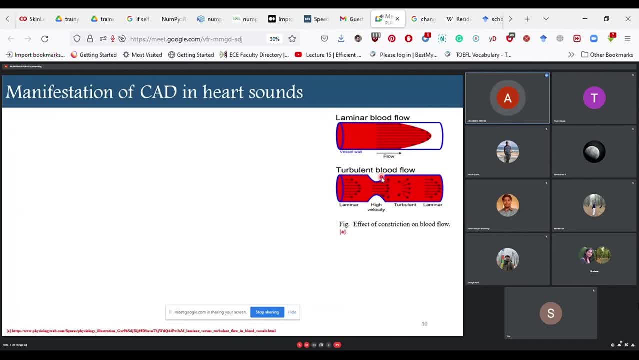 compared to those at the edges. but whenever there is a constriction or obstruction offered by appeared in the appears in the blood vessel, what happens is the particles of the blood start moving in some random direction. so this random direction is produced, produces abnormal sounds which are known as murmurs. again the same thing if they are audible. 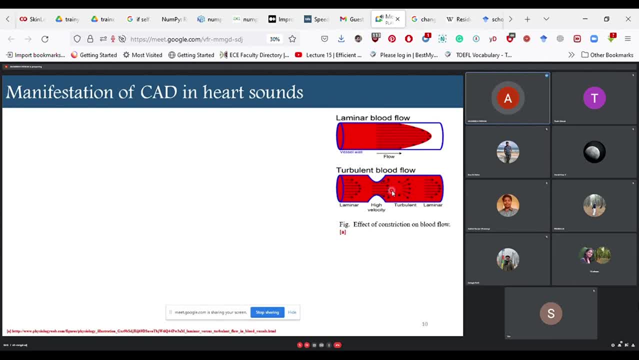 they will be some murmurs, but if they are not audible they will be termed as vibrations. but the streamline flow or the laminar flow does not produces any sound. it is like very calm and complex. so in this case we say that the heart sounds. uh, since they are generated due to the same 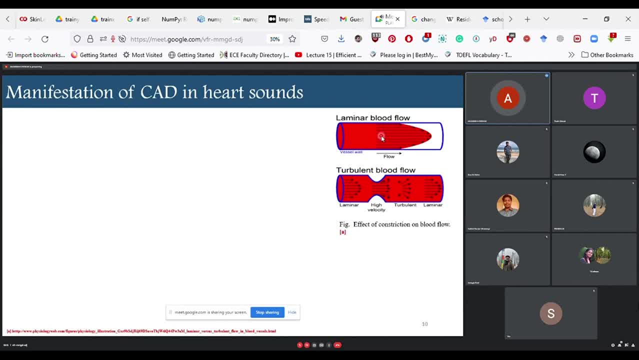 activity, as i discussed before. so these vibrations and murmurs, if any, are added to this original heart sound itself. so in this way we can say that, okay, my heart sound signal is getting added with extra other vibrations and sounds which are generated due to obstruction or in the blood. 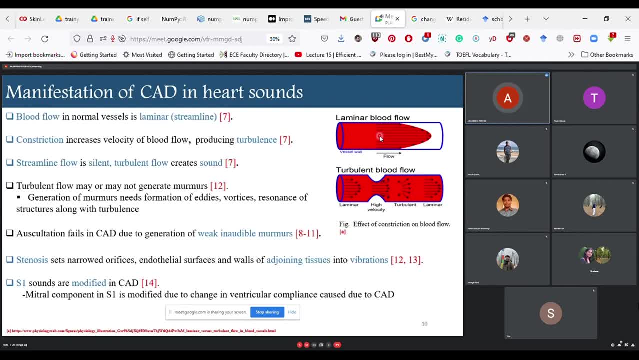 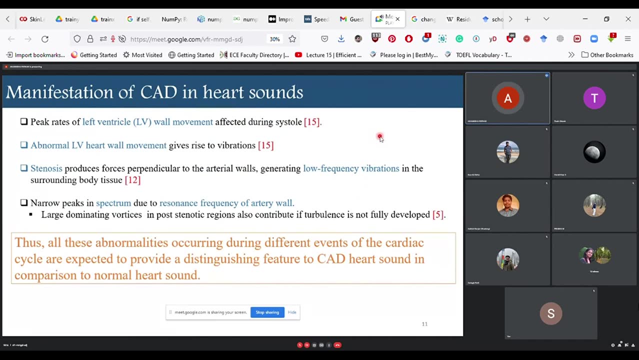 vessels. okay, so, um, yeah, this is just some detailed discussion, like which some, some special phases are being affected, or the entire signal is getting affected. so so we expect, or there's an intuition, that, okay, all these abnormalities which are added at different phases of the cardiac cycle, they are expected to provide some distinguishing feature to the 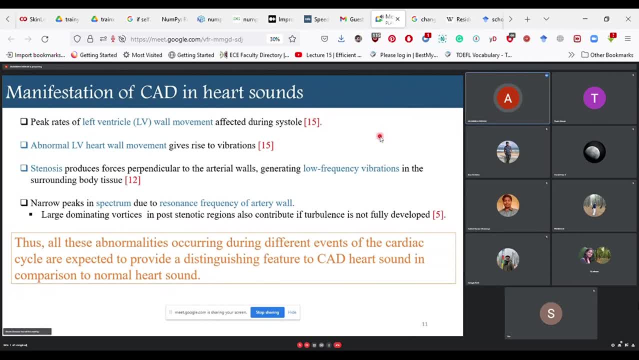 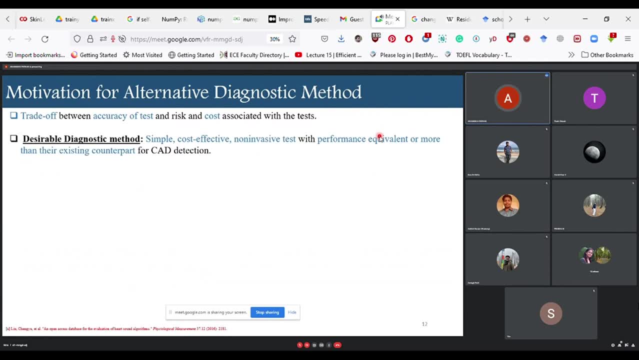 cad heart sounds compared to the normal heart sounds okay. and last but not the least, what is the motivation? see, currently we saw that the gold standard method is testing with such gold standard tests because obviously the cost and the pain they suffer during this testing as well. so in such a case, if at a primary of uh care or 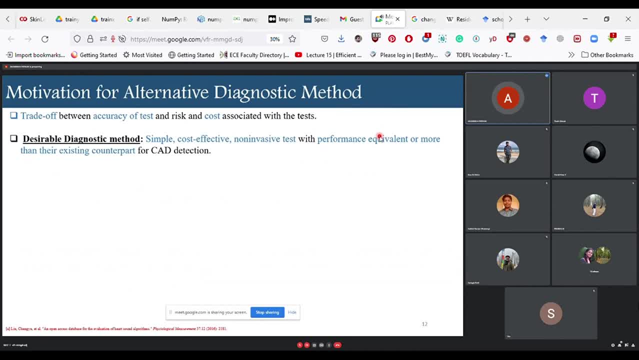 level if we are using some non-invasive and some low cost method. that would be obviously like good, since people will approach more for testing. so this is like one of the major advantage with heart sounds. they are now invasive, they are low cost. we just need a simple stethoscope. 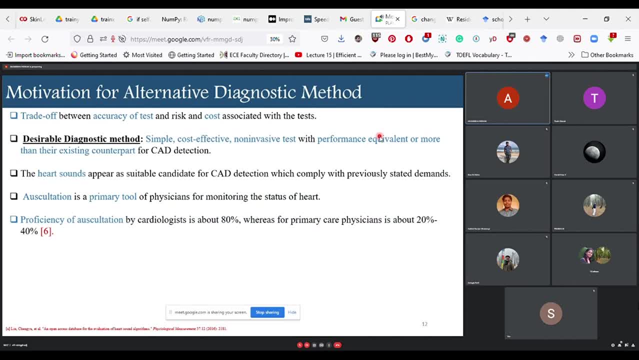 and a system for diagnosing it. major, important. but a point of using this entire signal processing and computer rated diagnosis is that auscultation is like. the proficiency of auscultation is very low among the physicians. as I played those two sounds for the disease case you. 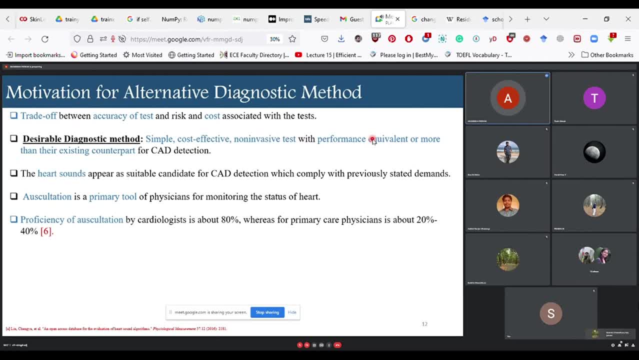 need to be trained properly to identify which sound corresponds to which abnormality. now, this is a like very practiced, even for senior cardiologists. this proficiency is like not 100 percent, it is about 80 percent. so you need to have rigorous training to identify the sounds as per the disease, which is not possible for 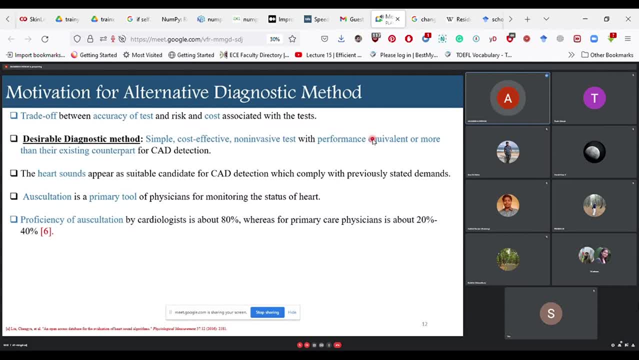 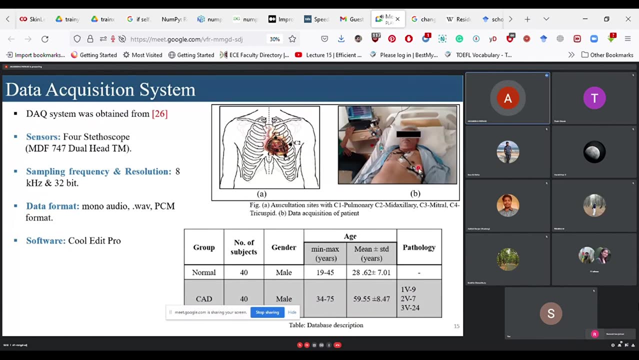 a human listening and it limits our auscultation ability. so in this context, we can say that a computer-aided method finds its way. okay now, as I already discussed how the data is acquired, this is just like how the data was used in our study, so main. key point is that we need to be able to identify the sounds as per the disease. so we need to be able to identify the sounds as per the disease. so we need to be able to identify the sounds in which way that refers to the signal processing. so one of the key points of the data, or the 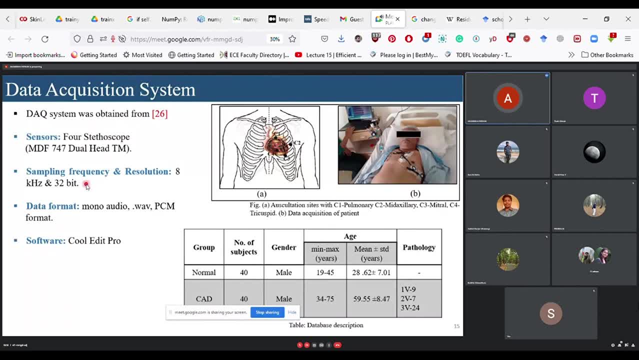 phono cardiogram being recorded is like the sampling frequency which you should use. so that should be a general knowledge from the prior knowledge, from the literature. what is the range of the frequency of the signal? and obviously by nyquist rate of idea you can go for twice the highest frequency content. so to be on a safer side, we took like more 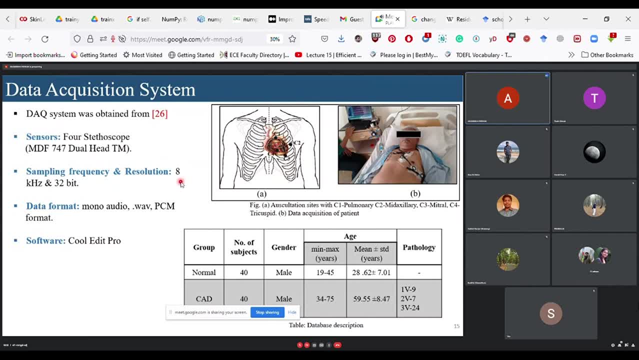 than the nyquist rate to have any prior experience. okay, like in general, we have seen it is possible to measure the sound level per second. so it was possible to measure the sound level per second because of theTechnology. we checked the data which was shown and the frequency of the anode: high state. 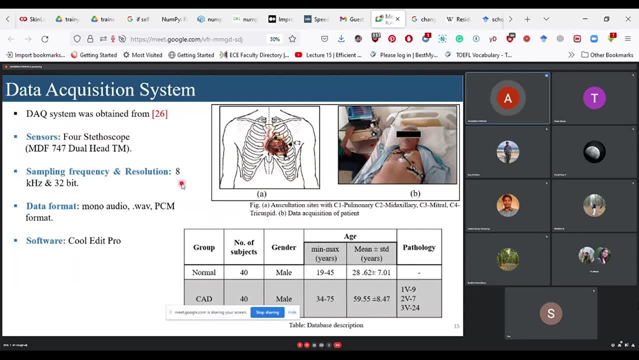 what, in case, the we can, we can have a higher range of frequency, just for being on a safer side. we took 8 kilohertz and the sensors obviously depends on you, so you can go for. the better the sensors are, the better is the credibility of. 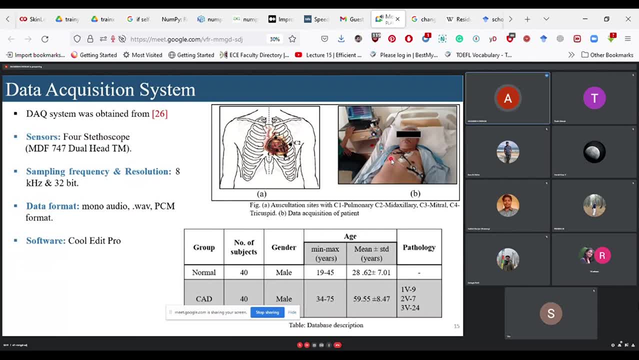 your data, obviously, so you can use this in our case, like we have used four sensors or four stethoscopes at, and we are using them to record the data simultaneously from four different sites on the chest. so, like at a go, data from all these four locations as we is being recorded simultaneously in the form of. 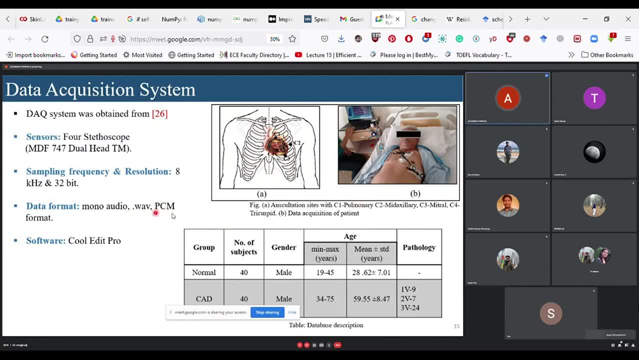 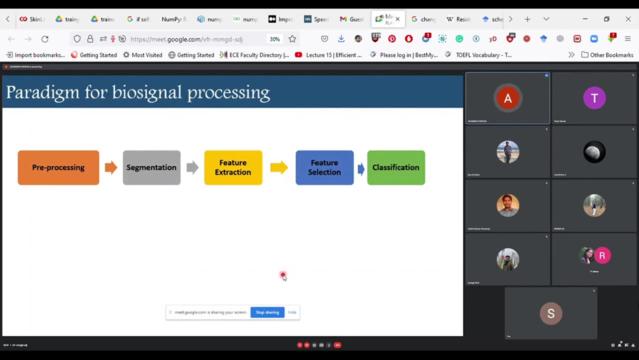 and being stored in form of PCM dot wave format. so here we are used like data: 40 care and 40 normal male subjects. yeah, how comes the paradigm for value signal processing? so basic paradigm as shown is pre-processing, then segmentation, each extraction, selection and in classification. so what is pre-processing? so the pre-processing is: 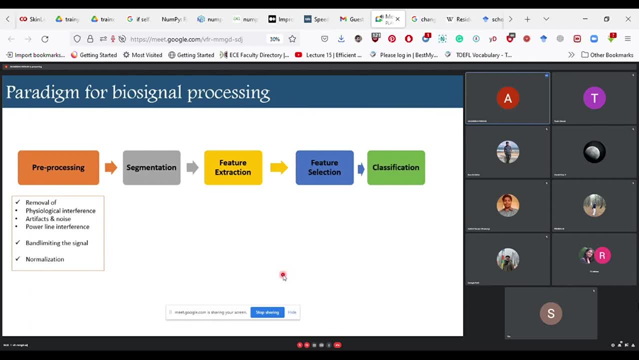 like removal of just nourishing your signal to get the most of out of it. this is a very crucial stage. if you don't after data, if you don't pre-process a signal, if you start dealing with noises also along with a signal, then you might lose important information and might be. 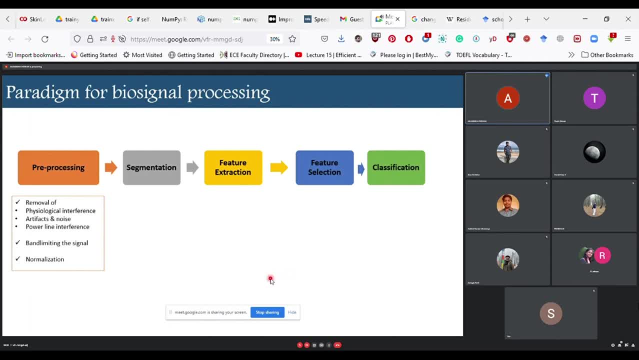 dealing with some irrelevant content. so pre-processing is basically like removal of artifacts and noise, some power line interference, some physiological interference, for example physiological and necklace. what is physiological interference? physiological into this is something which automatically gets added to your signal and you can't help about it, removing it at the acquisition. 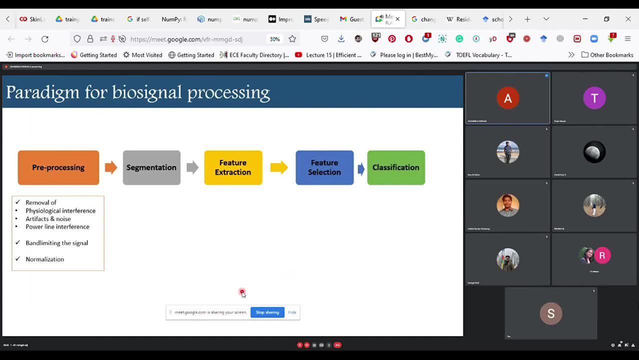 states, at least in. for example, in case of hard sound, if you have some bowel sounds in the stomach, so they get automatically added to the signal during acquisition. so you need some sort of signal processing to remove those sounds if you can identify them by listening or by some visual. 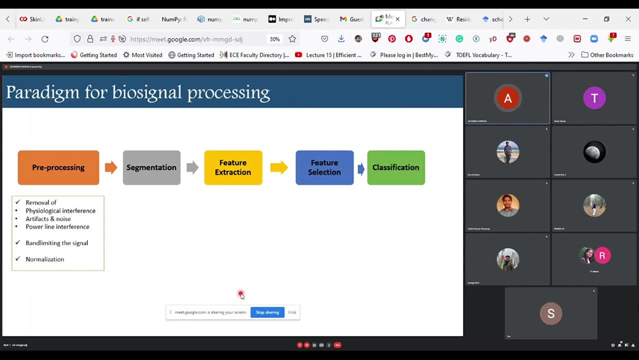 visual display or the respiratory sounds- uh. if you uh, which automatically get added to the signal while acquiring the heart sound, or vice versa. for example, you are acquiring the respiratory sounds, your motive is to acquire respiratory sound, then heart sound will automatically be added in that signal. you can hear it very nicely. another could be like a mother with a fetus, with a fetus in a 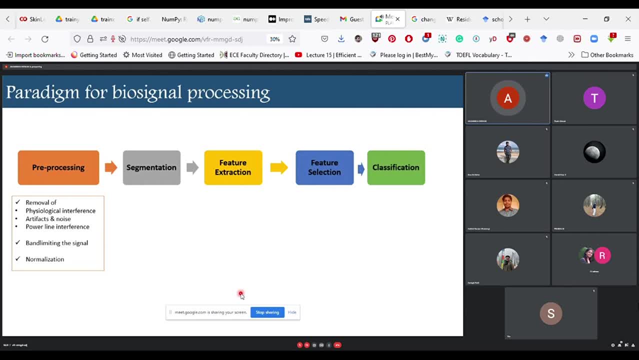 womb, so the fetus sounds automatically get get added to those of mothers. so these are some like those interferences. you cannot unavoidable interferences. they get added. either you change your data acquisition methodology according accordingly, or use some signal processing methods to remove these interferences. next is artifacts and noise. artifacts are not physically refers to uh. 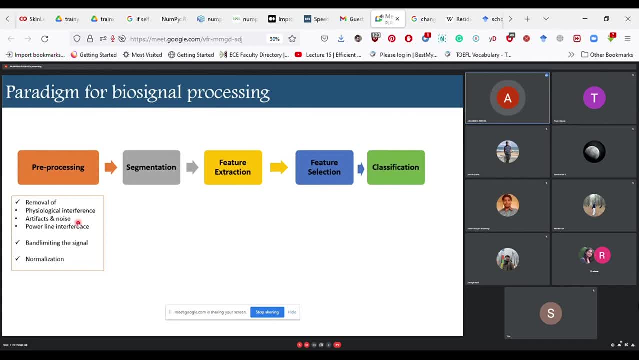 environmental noises, uh, for example, the environment where you are acquiring in a hospital. you might hear voices of people or the machine related sounds. they might get added to the server next, and those are just differences like height and noise in external employees. so, for example, if a robot isわかing the signal through his or her mem포logy, 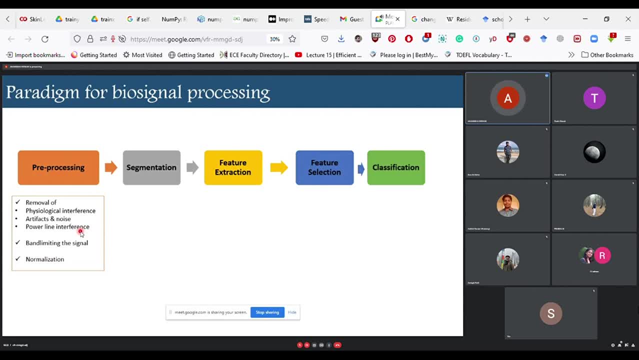 then you have between 600 max php. the signal quality code, especially if the sd Stefan uh is not being Aaa, can be disinformation if you're introducing more than 2000 sHello – um, imagine if I were to make a robot that still has a pipe, thisophone material, straw plus. 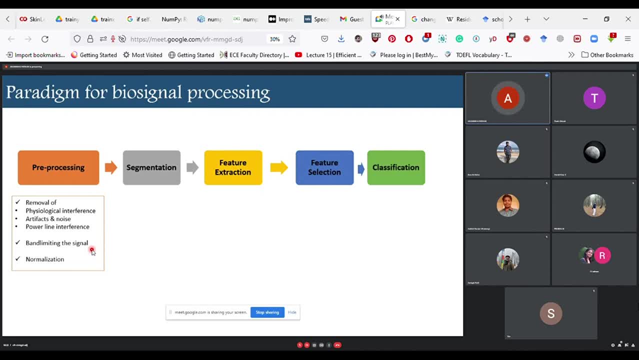 smooth sound from fx culture device planning chips or uh wire, Big Big Pop stickers and vgas Gabe devices and uh vibrate, uh continuously as per needs. so power supply, which usually gets added to the signal filtering or high pass filtering, whatever is required as per the usage. and next last, 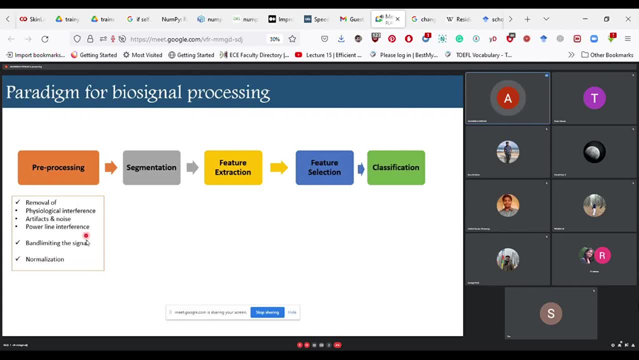 but not the least is normalization. so after doing all these processes, obviously you are using some signal processing, so the values of the signal might change a lot, so you need to scale them at a definite range. so either use a z normalization or a min max scalar, whatever suits your need. next process is segmentation. segmentation is what segmentation is like. 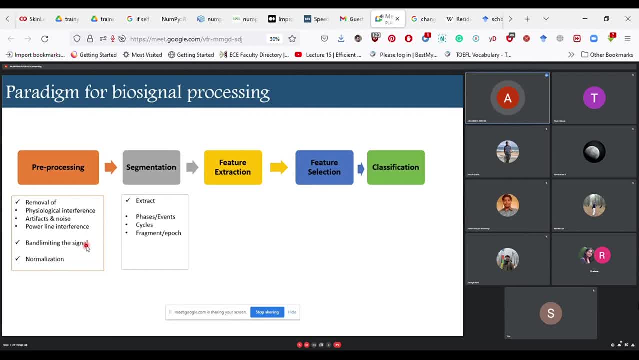 identifying the main phase or the event or the cycle or the fragment, like: what do you need for dealing with the signal? do you need some specific phases? for example, in our case, do i need only systole or diastole or s1 or s2. so what do i need? 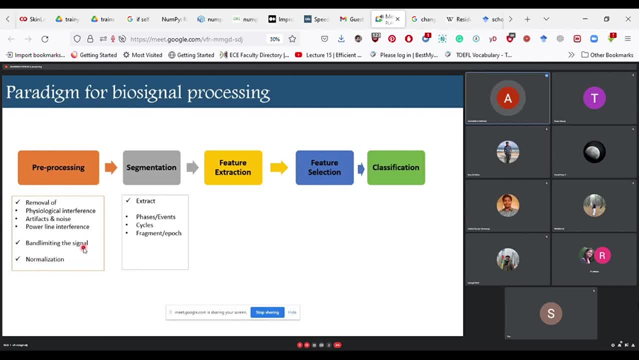 among all those phrases, or is it like: do i need the entire cycle for my feature extraction purpose, or do i need a longer fragment, like multiple cycles at once or so? this is like people. so what do you need? you need to, uh, identify it, either using literature or using. 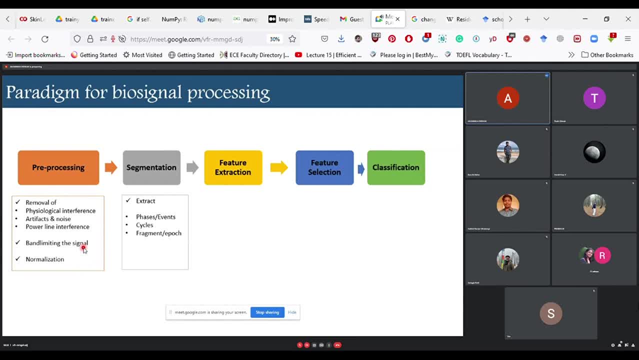 some statistical methods which convince you that, okay, you should go for this. next is feature extraction. so feature extraction could be handcrafted, or representation learning base handcrafted. i've just listed four. you can say some sort of broad categories, but it can be more than that, excuse me. so handcrafted is like time domain, since we are dealing with. 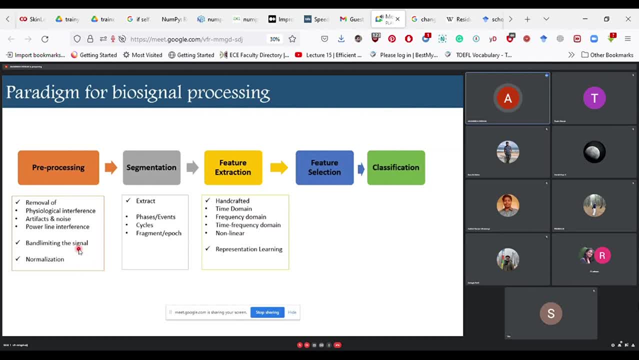 a signal, one dimension similar, we can say time domain, frequency domain, time frequency domain or even non-linear domain. so all this is a part of biomedical signal processing and feature selection, classification, which is a feature selection, classifying feature selection, and these are all things that are still attributed towards the machine learning. 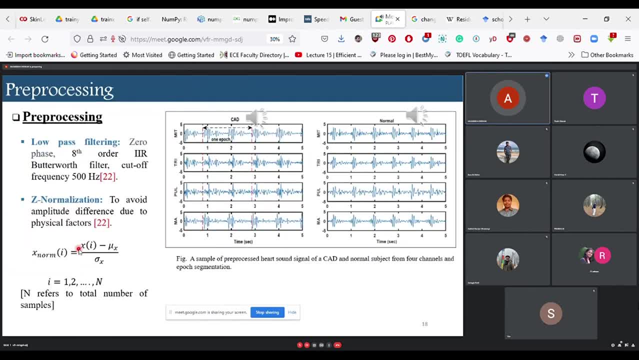 in this case. basically we are dealing with. in our case, we took pre-processing as just low pass filter, limiting it to 500 hertz. since our signal was by audio investigation, we found that there were not much noises. moreover, the data in our case was also recorded in a breath. 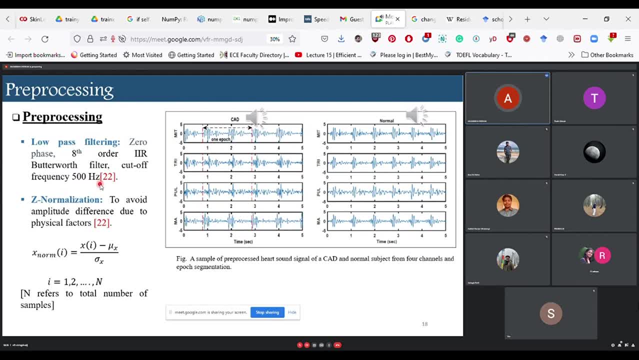 hold state so automatically. we eliminated the respiratory sounds, so this was like one technique. but obviously if you are taking a, the sound recording, the sound in the breath holds it. it limits the duration of the data. one cannot stop the breath for one minute. it is. it can be holded for a few seconds. so there comes a trade-off. 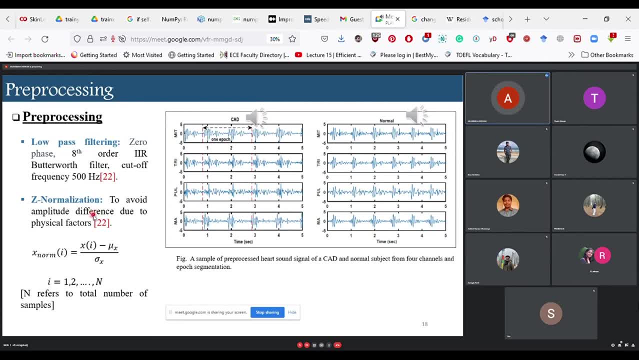 and next is like: normalize the signal using z normalization so you can see like this is a visual display of the CAD and normal heart sounds and the labels on the right. this MIT right, well then I mean- basically refers to the four auscultation sites on the chest: mitral, tricuspid, pulmonary and 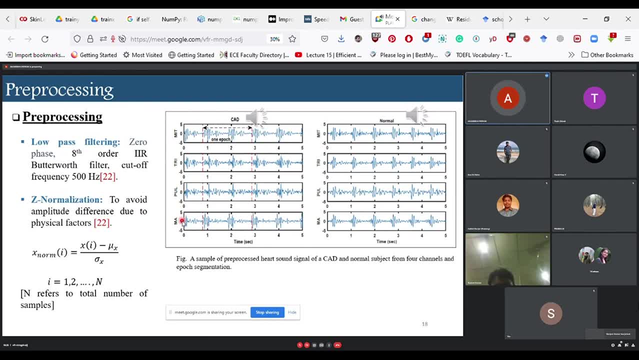 mid axillary and so on. so I think, visually, if, if you are able, if you see you cannot identify very distinguishing patterns here, and audio wise also, it is not very prominent to identify, okay, unlike the stenosis and regurgitation sound which I told, which I have displayed before, the, the visual even. 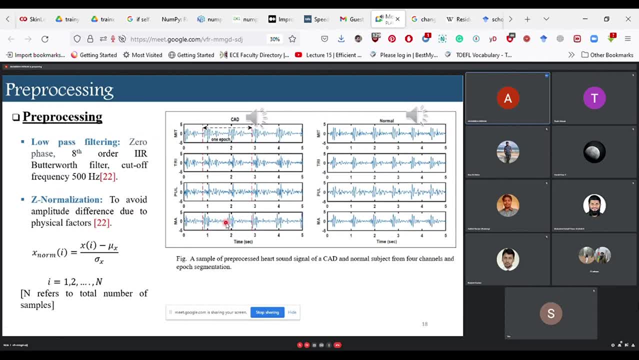 the audio characteristics are not also very differentiable. so this is like a very uh hard problem because, unlike the previous cases where I showed the regurgitation stenosis of the walls, they are very evident. the visuals are evident, the audio is evident. okay, there is an anomaly, but in 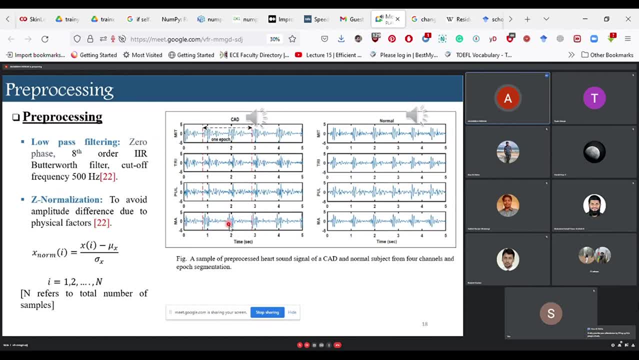 case of CAD. uh, this is very difficult, basically because the murmurs on the generated are very weak since they are on the muscles, so it is very weak. they are very weak to get added to your sound in a very strong manner. so we can only expect. our intuition is that there are vibrations which are being added to the signal, and we hope we have. 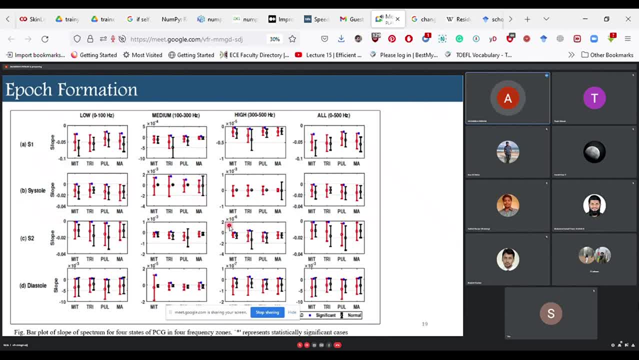 some patterns accordingly. so now in our case, like, how do we go for that segmentation process? so, um, we use some sort of status testing in order to identify. do I need to go with any specific phase? for example, in this literature survey, we have a dominant literature saying that only diastoles are the ones which should be used. 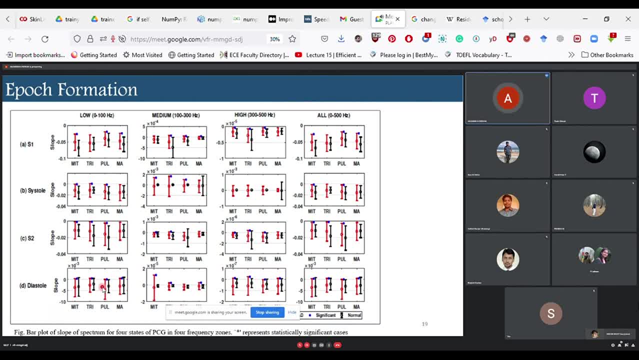 for investigation, because diastole is the phase where maximum blood flow occurs in the coronary arteries. okay, so there's a lot of clinical evidence as well as technical evidence of using the diastole, but still one should not block his head with the prior literature. but I think 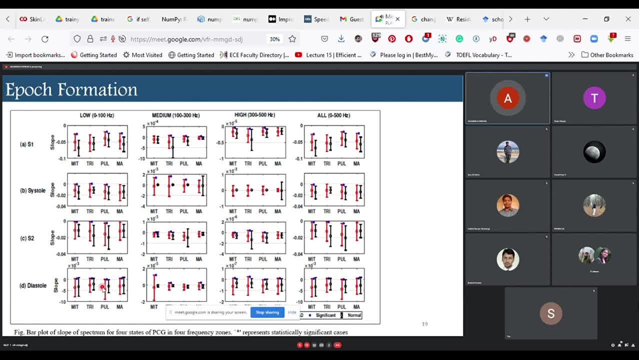 you should also proceed with like with his own intuition and understanding and a curiosity that let us go through some other ways also. so what I did was I just took four different frequency zones and segmented these phases- S1 phase, systolic, S2 and diastolic- using 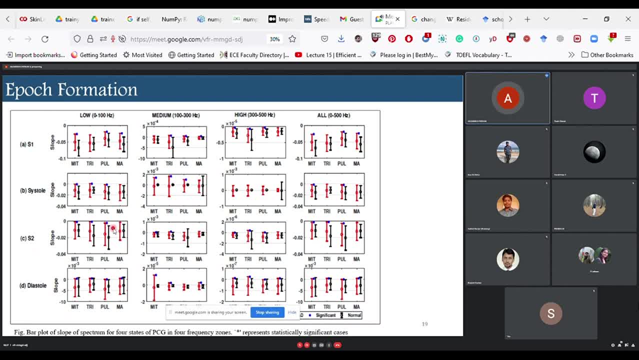 established segmentation algorithm in the domain and computed the slope of the spectrum of these phases in these four frequency zones, So the ones marked in blue, the blue asterisk or dot, if whatever you identify it as. so this is basically a bar plot. Bar plot basically means, like the inner circle shows the 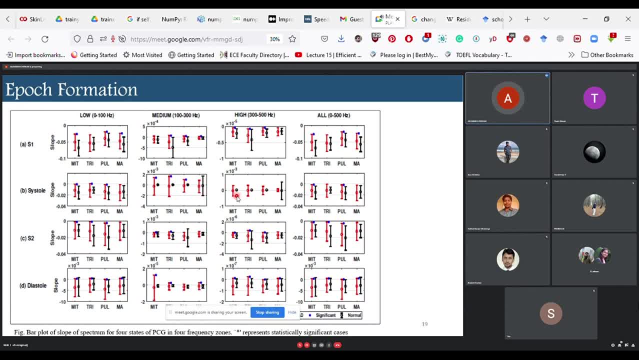 mean of the data and the whiskers show the variability or the standard deviation of the data. So red is for CAD and black is for black, bar is for normal and the ones highlighted with blue are like statistically significant. Statistically significant means okay, they are like differentiable. 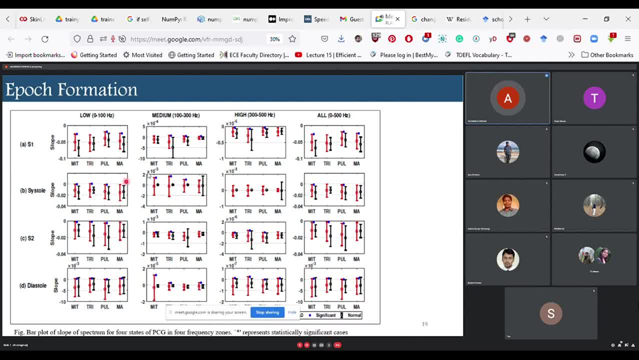 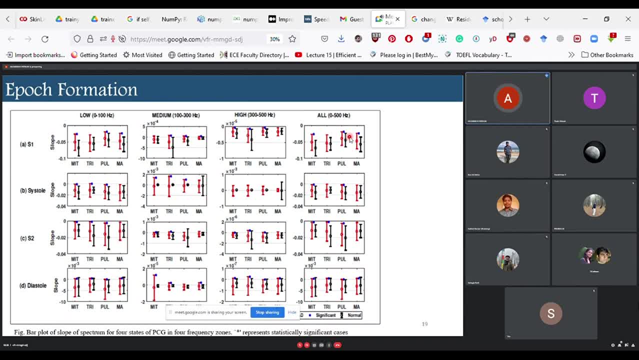 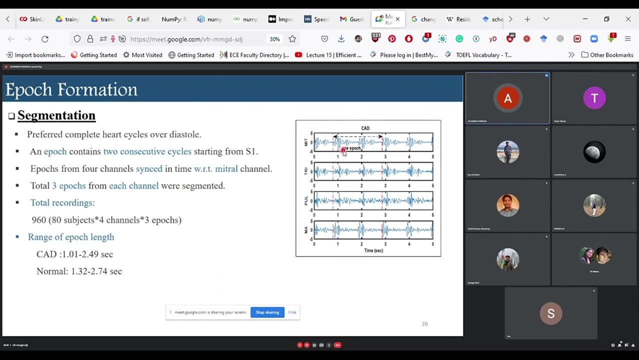 intermediate frequency zones or overall they are discriminative. So why should I only go for diastole? I will go for the entire cycle. So this is my intuition. So what we did is okay, I am taking entire cycle, but again, I am not just taking, going to take one single cycle, See the 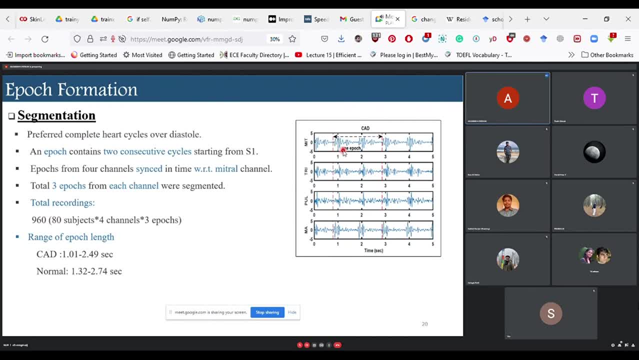 one single cycle duration is is maybe approximately, for example, one second or even less than that. So that length will not be sufficient for proper spectrum representation. See, the time is the frequency is inversely proportional to time. So the longer the length of time duration of the signal you will get, the better the resolution in the frequency. 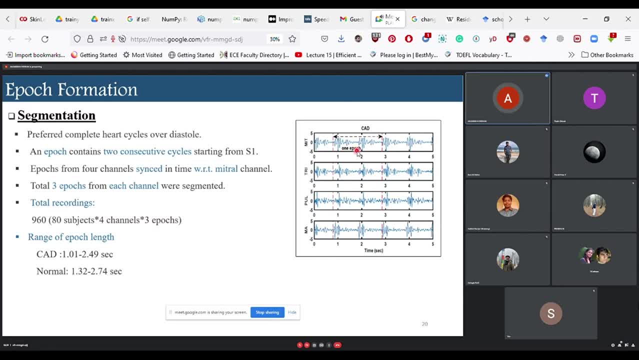 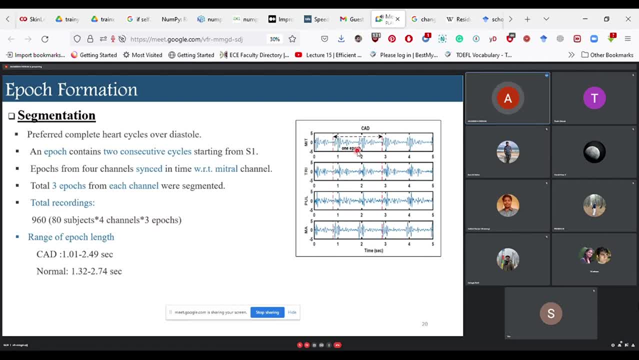 is like very important stage, because this is the stage where you are going to decide how good your model is going to be trained. So, for example, in my case we have an 85 subjects. So if I use the entire 10s data as a single epoch, I would be left only with 18 senses, and then with 18いました. 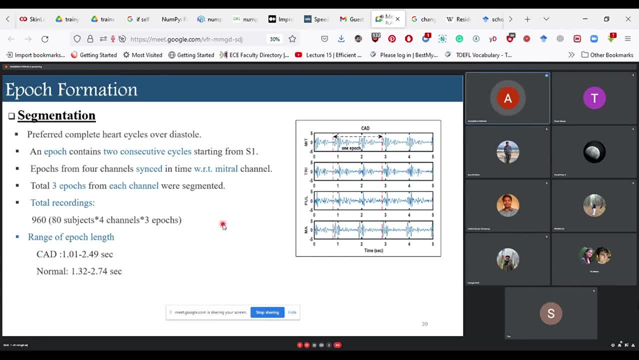 ENDS instances. I have to train the model, test the model, and if it is a neural network, I need a validation data. So I think this is a very simple path to go from here. you can enter 18 instances with the bare. 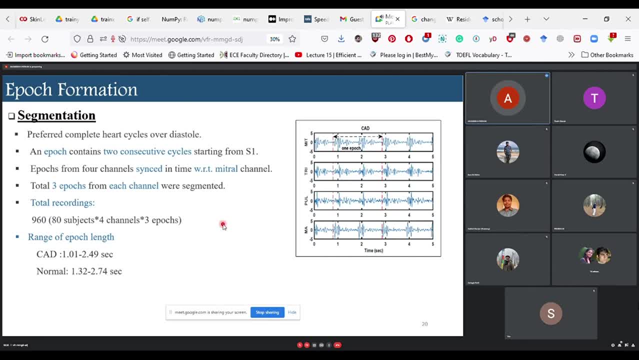 ims, buttonuli�� t, un stock have very less data compared to the image processing or other domains where we have the data in form of thousands. so this is the phase where you have the chance to increase the instances of your data. so what we do is like, okay, i'm take from the 10 second data. 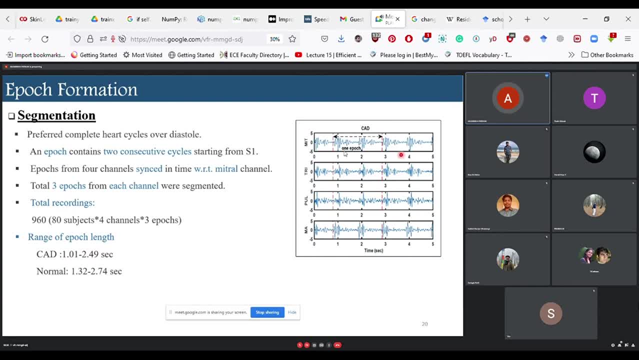 i am taking three epochs, i am forming three epochs. so in this case, in this way, i am increasing my epoch count to like 960: 80 subjects, four channels and then three epochs. i'm taking it like i raised it from 80 to 960. okay, so this is like i think everyone should focus. 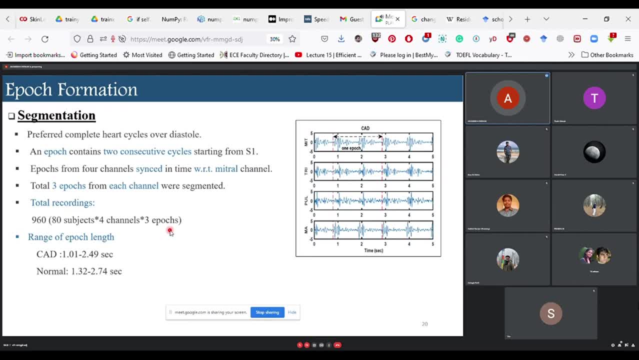 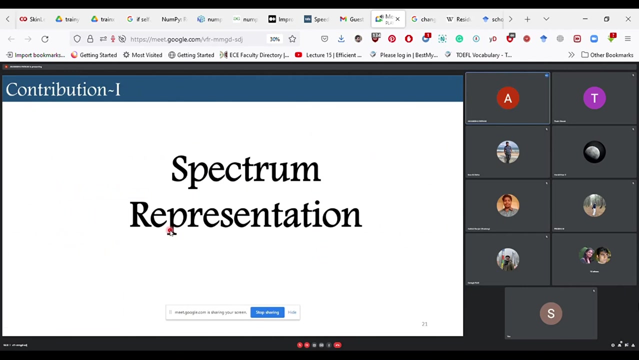 on this phase. how are you going to use your segments? because the segments, basically, are using the segment. knowledge is not only based on literature, but also it also lays the foundation on of a future machine learning training model. now we start with the first contribution, which is based on the spectrum representation. so before starting with it, i want to tell that we will 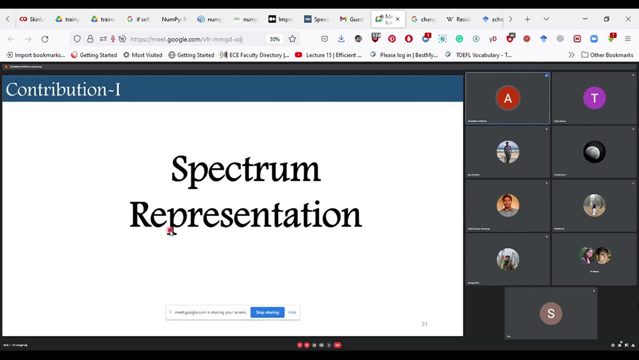 be dealing with a hierarchy of feature extraction methods. so the first and foremost hierarchy i am laid as spectrum representation. so spectrum, as you all know, basically tells us about what is the frequency range of the signal with the yeah. so how is like power distributed in the basic frequency range of the signal? so 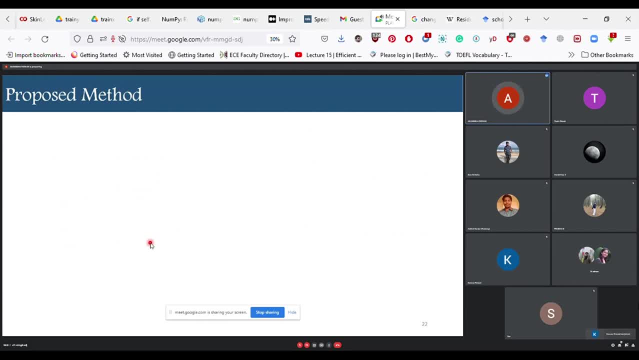 i am using hyper frequency to do theiu יח. i just want to, so i am like this is the load of ret каче. i am running like one hour after the signal is in good condition to be able to give us an above and under value. 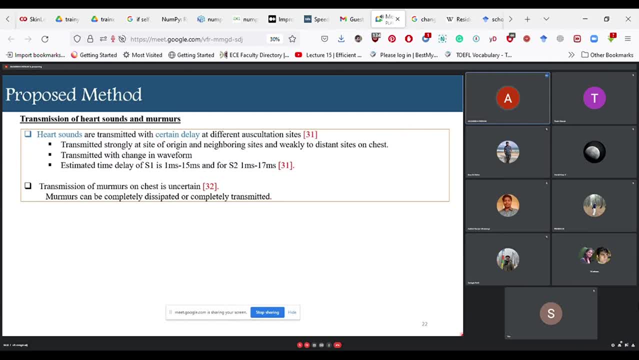 and ultimately- and then this is like a second set once again, and next is like a second set- physiology is that the sounds, or the higher sounds, basically they are transmitted at different auscultation sites, for example. so obviously you can hear the sound from different places, though they are generated at some point, but they are transmitted at different places. so 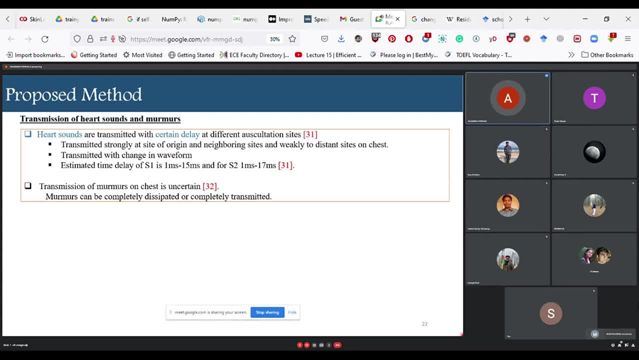 but the murmurs on the chest. they may or may not be completely transmitted. so, since we were acquiring the data from multiple sites, what we proposed is: i wanted to correlate the data of, or the heart sound of, two auscultation sites like: how is it correlated, but in frequency? 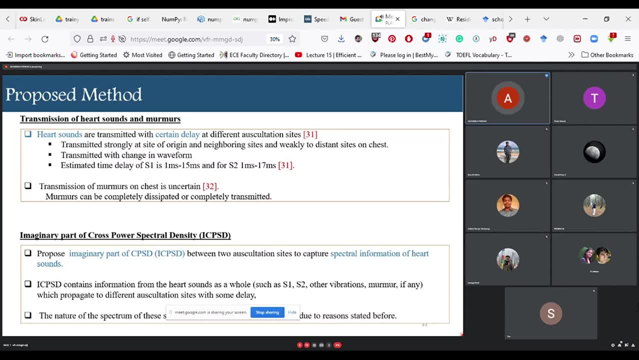 domain. so, as we have core cross correlation in time domain, we have the cross power spectral density in frequency domain. now the twist comes that instead of using the cross, the, usually what we would do is we would take the frequency domain and we would take the spectrum. so what we do is, when we have the spectrum, we use the absolute values of the. 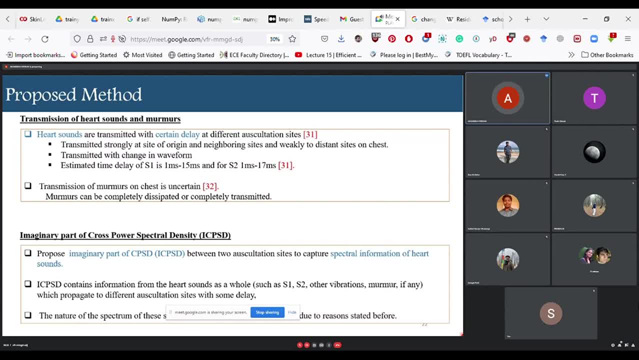 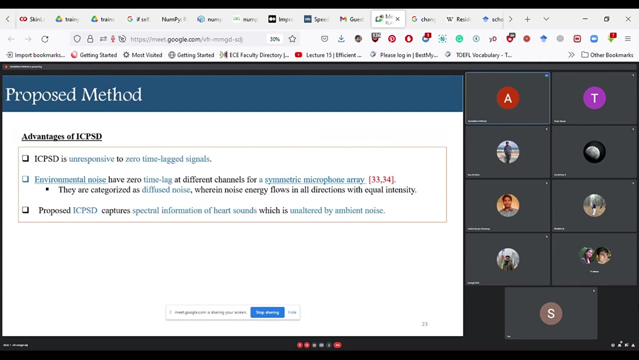 spectrum. but instead of using the absolute values of the spectrum, we, i propose to use the imaginary part of that spectrum. so what is the advantage of using the imaginary part? so imaginary part basically tells us that it is unresponsive to zero time, zero lag signals. let me give some sort of mathematical illustration. 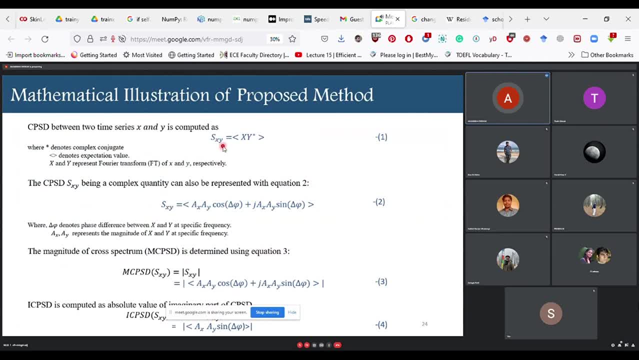 to this because suppose sxy is the spectrum, cross power, spectrum density of signal x and y and these operators, obviously our expectation operator, and i have written this in form of a complex number, rectangular paradigm fashion, so axe amplitudes, cos, delta phi and sign delta phi is obviously the phase difference and this is usually what we go, is when we take. the magnitude of the spectrum. we just take the magnitude of this cosine, cross delta phase x and y is the same. that goes for the classification. however, this b superb andarden mistake happens, then we know the Mickey's истории. eighteen, eight, no realization. f of nine can beこと. beautiful is you here? in biology that we have drunk. requires 2: 90. if we have both the quantity spirals or semantic, take it that our two. okay. if the amplitude itself it can be write to your точно, okay, and then we know later. k formula also does not not require any. 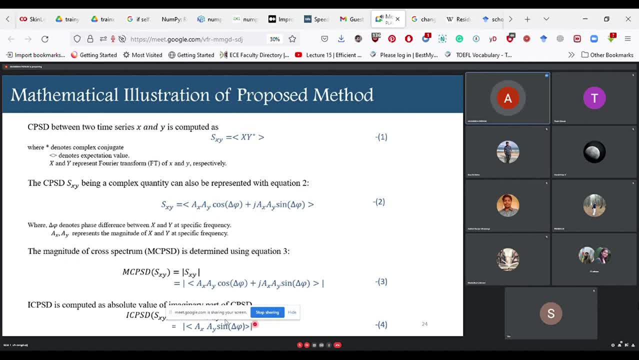 complex number, but imaginary component is restricted only to the sine phi function, the sine phi a, x, a, y, sine phi, sine delta, of sine of delta phi. now, if this phase is zero, what is what is? is it going to be? it is this imaginary part is going to be zero, but we'll still have the 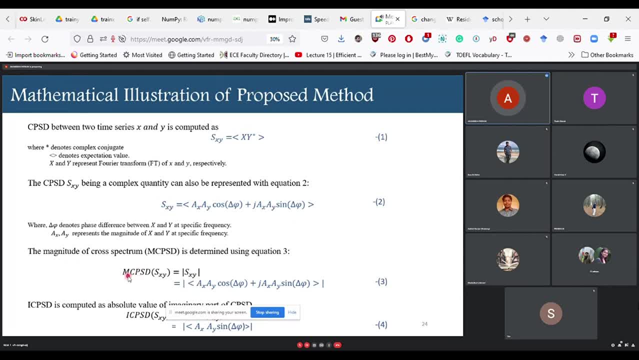 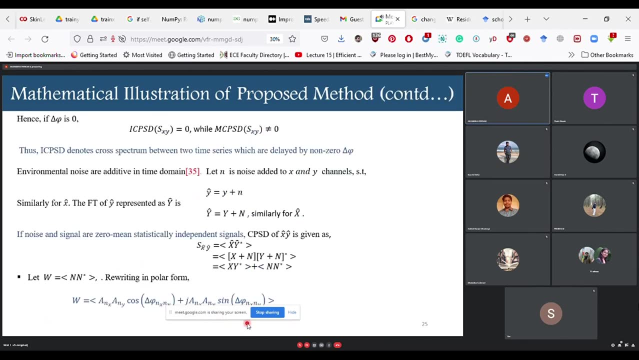 real part and that gets added, that is retained in the magnitude. so this imaginary component is basically retaining only those similarities which are delayed with some phase difference, with non-zero phase difference now. so what happens is whenever noise gets added to the signal, so the noises usually are, especially the environmental noises, they are usually additive. 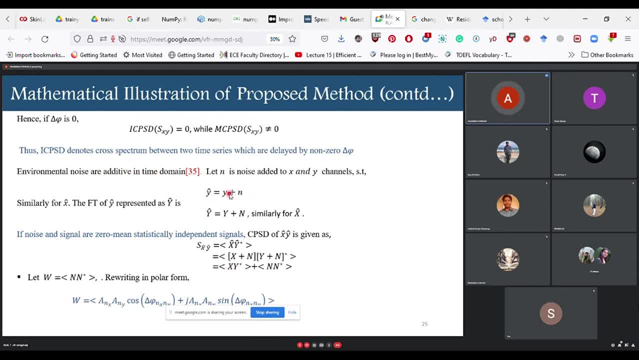 in time domain. so, for example, original signal was y and some noise gets added, it becomes y, hat in fourier transform by the linearity property. we can say it: the noise is also, the spectrum of noise is also added in the same way. now, if we take the cross power spectrum density of these noisy signals. 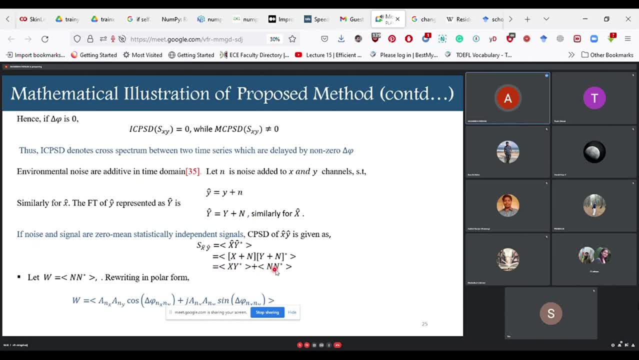 what we get is original signals, cross spectrum, plus noise cross spectrum. so what happens is: we get this is sine of delta, phi, nx and ny. now what happens is for environmental noise is that we get this is sine of delta, phi, nx and ny. now what happens is for environmental noise is that 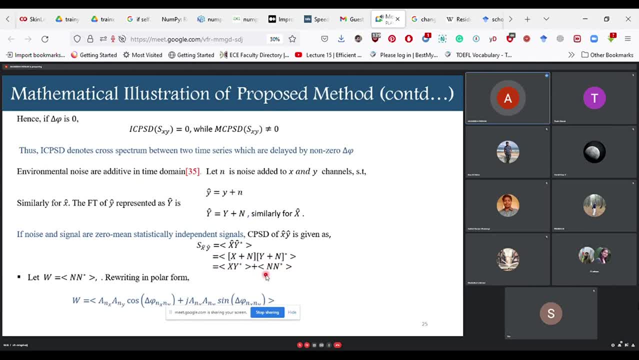 we consider them that they are appearing from a distant place. so whenever something is falling from a distant place, we say that it is appearing as parallel waves. same, for example, we have heard- we have must have dealt with it in our physics classes- that if something is coming from far, 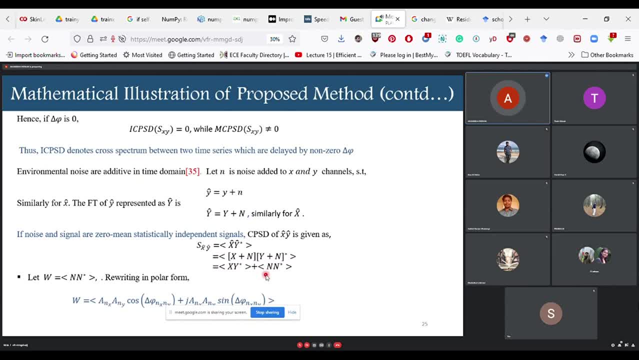 off place it is, and then it is received in form of parallel waves. so parallel waves means the there would be no phase lag and when we are capturing that noise of the spectrum we get much less difference. so when we get theаг Надd but and we take an image that always allows 빹n structured 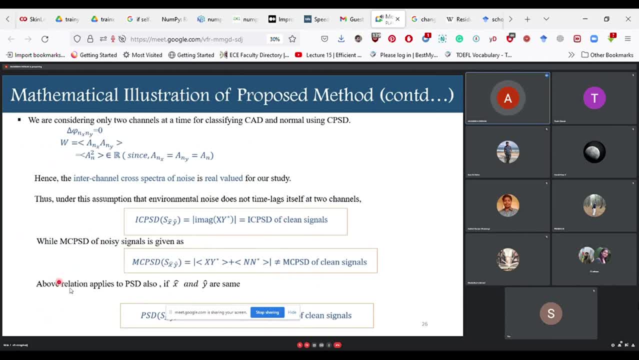 sondern we also take has no phase lag at multiple channels. so obviously the phase difference is zero. so when we are dealing with imaginary component of the spectrum, we automatically get rid of the noise spect not restricted to. this idea is not restricted only to heart zones. one can use it whenever. 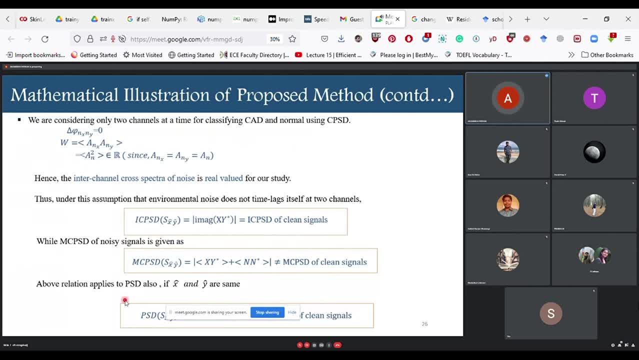 if he sees that, okay, there is sort of phase like condition and i can, i would like to use a imaginary component to get rid of the components which are automatically getting added with without some phase difference. so i must. i would like to mention that i inherited this idea from the 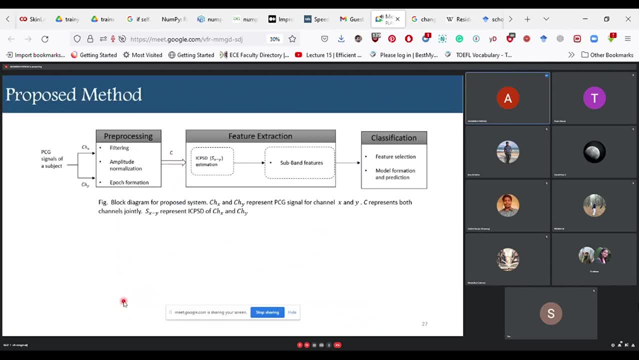 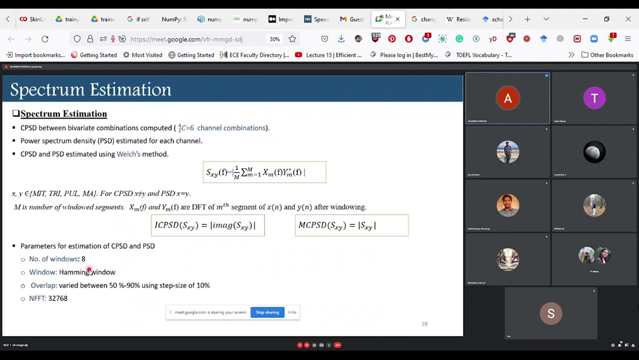 neuro domain itself. so, um, so, once we establish, okay, which spectrum we want to use, okay, now the question arises: what features so spectrum? i will just say it was associated, using welch method, and these are the basic configurations. now, this is the spectrum of all the four c2 six channel. 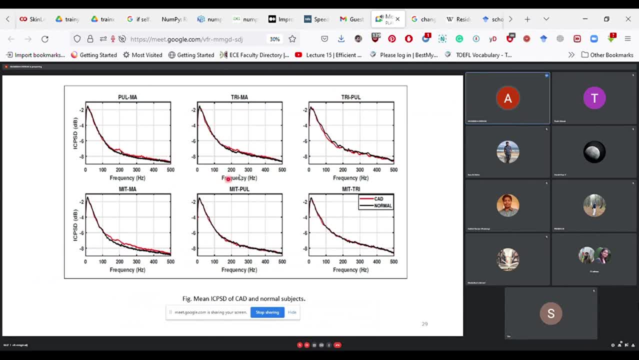 combinations we can say it is like highly overlapping. since it is highly overlapping, we can see that it is not very nicely differentiated. so the theory which we have that visually and audio it is not differentiated, we can see it in spectrum domain also. the cad and normal heart sounds are not 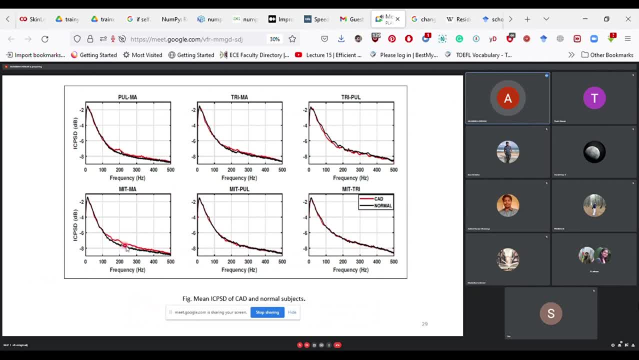 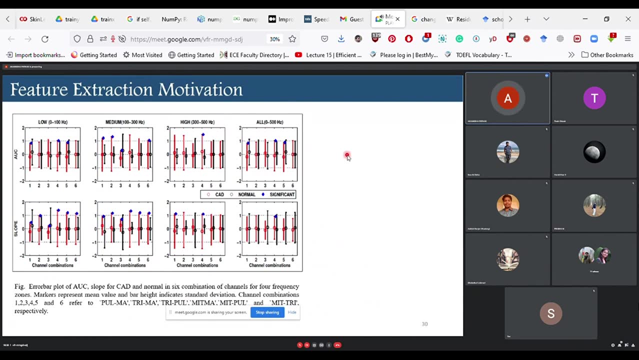 discriminative, so what we? but they are discriminated in some intermediate frequency zones. if we see in some cases, but not completely overall, you can say okay, this is highly discriminative uh patterns. so again, a statistical testing was done to to validate my intuition. i am saying that some, in some bands or some frequency regions, it is discriminative. but 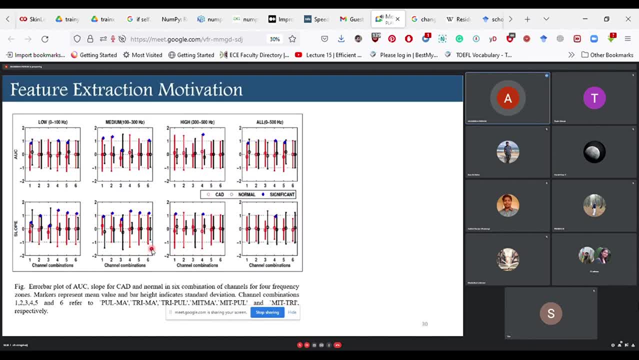 not overall. so a statistical stress not only gives you a confidence to proceed, but it also gives you a good quantitative proof. okay, that, yes, and it proves your intuition also, because, uh, research is not just based on intuition, it also. it is also based on facts and evidence and statistical tests. so one should obviously 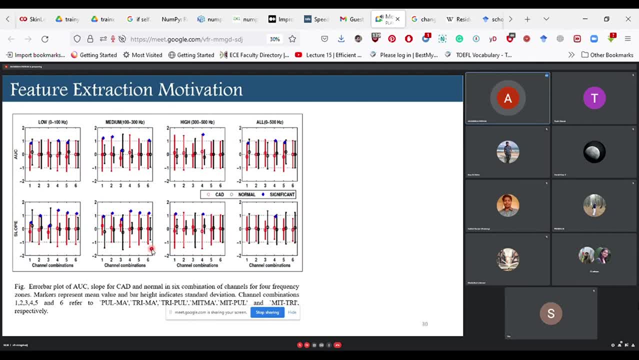 um, try to validate the intuition using some sort of statistical testing, but how to design that test is also based on your intuition. so what uh i did was i again took some intermediate frequency zones- low, medium, high- and the overall- and computed the uh slope and area under the curve of that cross. 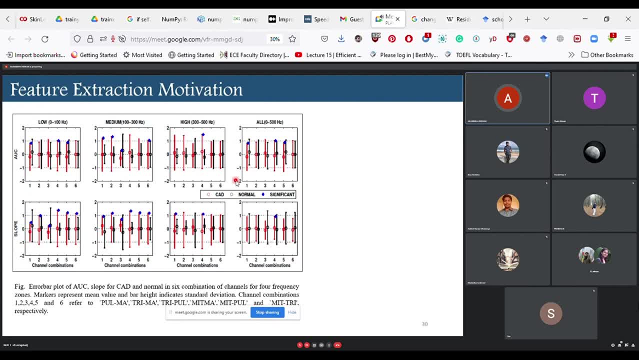 imaginary cross spectrum for all the six channel combinations. so again, this is the mean, imminese plot. so what we have been trying to do is that we have given someeto average innumerable batHAHAJ which will need to be skiing this Lift at end of your intuition during the study, and let mekelize out kind of the average intensity. 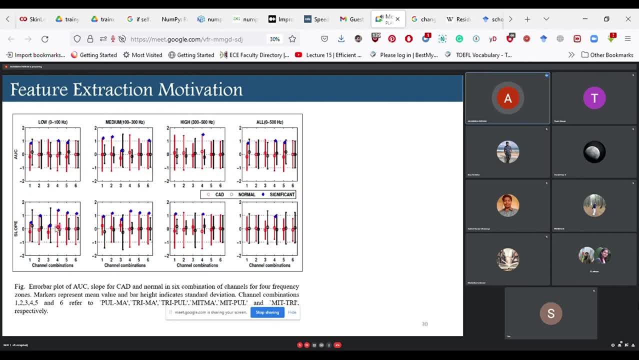 we see is that in the intermediate frequency zones you will see more significant portions compared to the overall frequency zone. so, okay, this gives you confidence that, yes, a band level approach will be more good to extract the features rather than using the overall spectrum as a single entity. 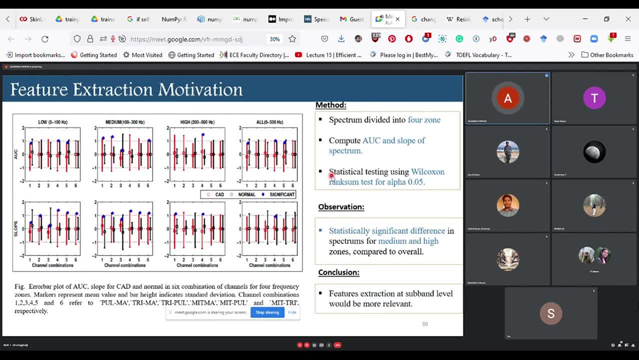 so usually you can go with any sort of test, uh, statistical testing. it depends on your data. if the data is normally distributed, you should go for t test, uh or the z test, whichever suits your data account. but if you your data is not normally distributed or you don't know which distribution it is following, we usually go with a non-parametric. 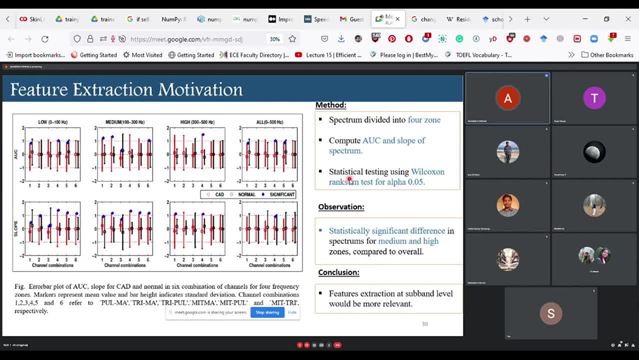 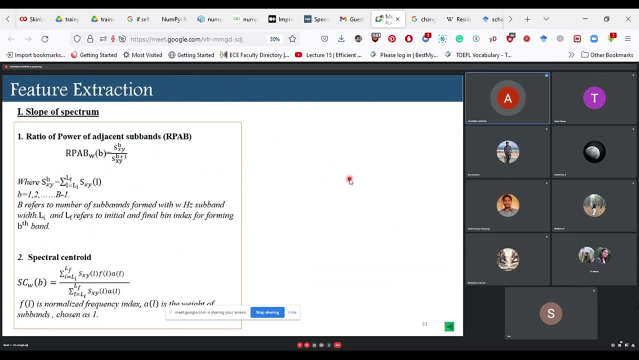 test, like wilcox, some rank, some test or others for features i just extracted. considering the intuition of slope, i took ratio of power of adjacent subbands and spectral centric. so these were extracted based on some bandwidth. but again the question come: what should be the proper? 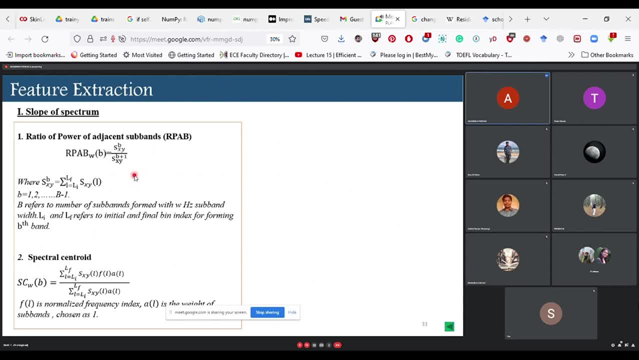 bandwidth. i don't have any proper intuition or the idea or a proof that what should be the prominent bandwidth. so sometimes we can use empirical based approaches also. so i just empirically experimented with narrow bandwidths of 5 hertz to broad bandwidths of 100 hertz. 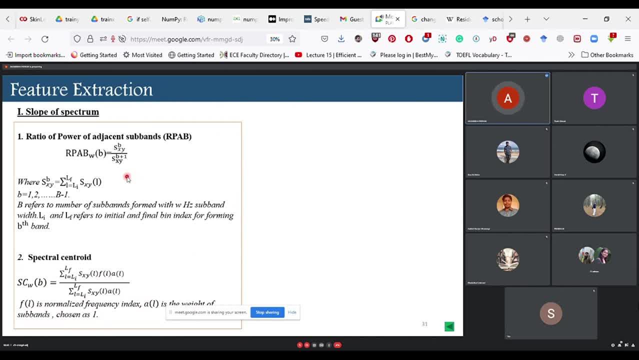 so 5 hertz bandwidth means i'm making the band in the range of 0 to 5, 5 to 10 and so on, and for 100 it's like 0 to 100, 100 to 200 and so on. so i'm computing like ratio of power of adjacent. 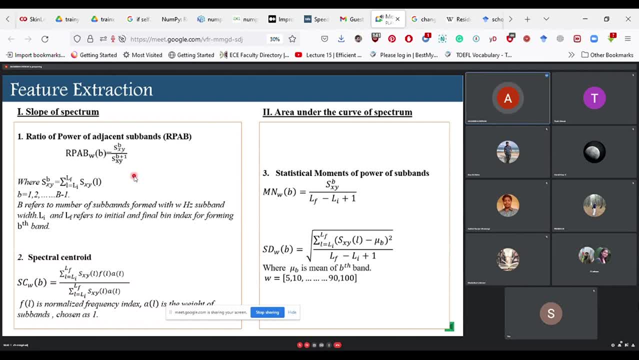 subbands, spectral, centroid- and statistical moments of the first two moments of the of this power in the bands. so in this way, i'm not going to deal with the show with the results, but since my aim is not to show the results but focus more on the signal processing, so we use these features and finally we build a model which i'll discuss. 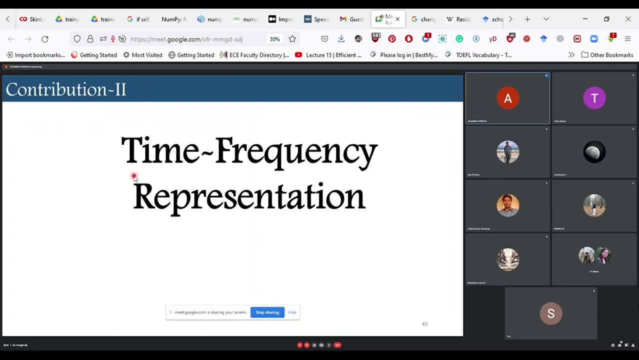 later. so this is like the first hierarchy. next is like the time frequency representation. now i am moving to a higher hierarchy. why i am moving to a hierarchy, see. first of all the bio signals are like highly non-stationary, so i'm moving to a higher hierarchy. so sometimes 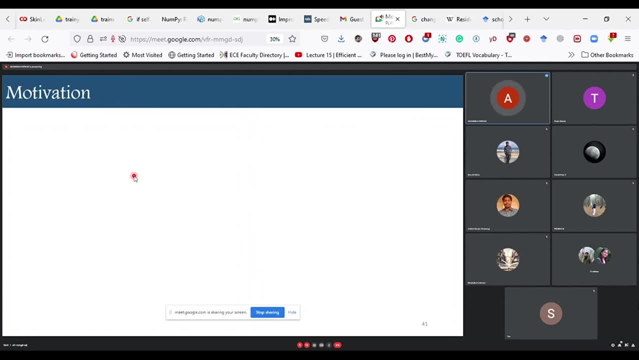 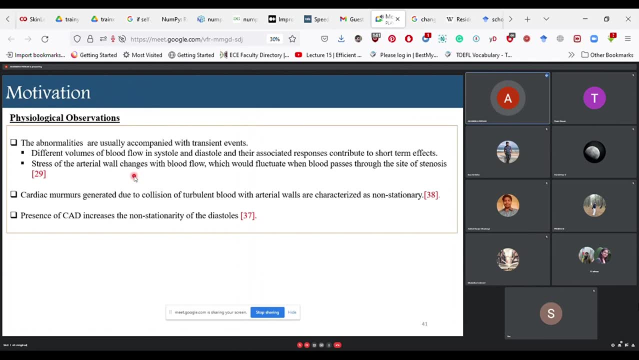 like my in this one time frequency representation, i'm moving to a higher hierarchy. why i am moving signals so, and using a spectrum based approaches like and dealing with a stationary signal. so there are a lot of transient events. transient events are like something which is very localized. 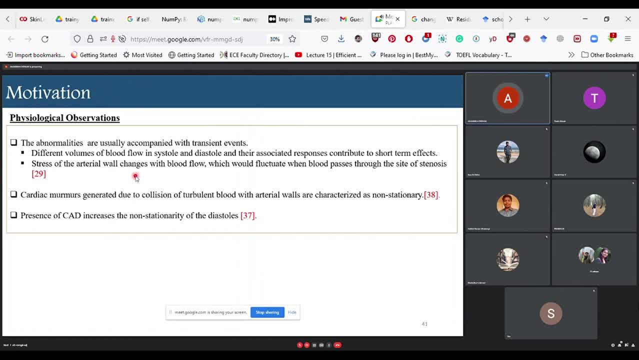 at some instant of time. so obviously something which is a very minute event, which is occurring for a smaller phase, will get overshadowed in your spectrum. you will never be able to localize it well that when this event took place, but a time frequency representation is like you are studying. 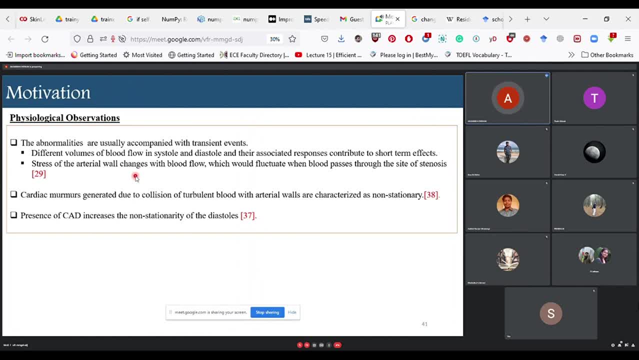 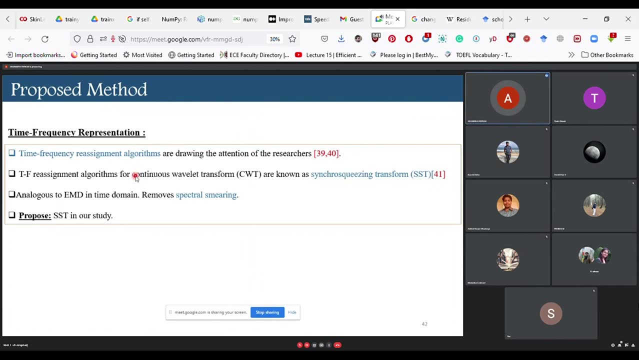 very precisely at which time, what was the frequency component of the signal, which frequency was high, which frequency was low, and so on. so obviously, a time frequency representation gives you a greater clarity. okay, now the next question arises: which time frequency representation should you go for? so it's not like that you should always go for the trending representations. 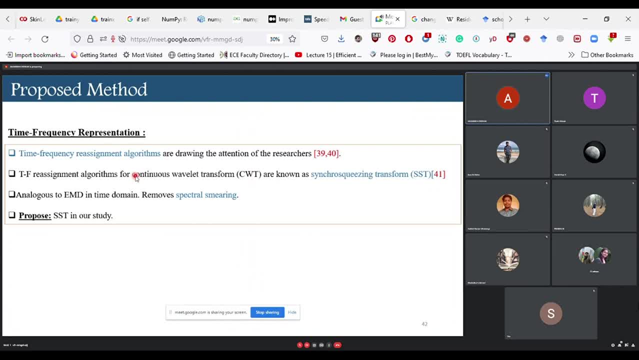 in the research a speech signals is still tried like the basic layout of the speech signal processing is short time period transform because they are suitable for it since they follow the norms for using the short time for a transfer. that the signal is stationary for short duration. if i am speaking in a in a tone, 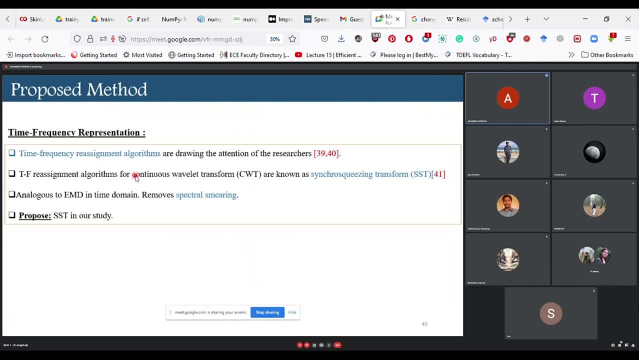 obviously some content of my speech will be stationary until unless i change the emotion or the content of my sick, of my speech. so a short time for your transform will be a short time period suitable for speech, even till now. but for the cw, but for the biosignals, other biosignals. 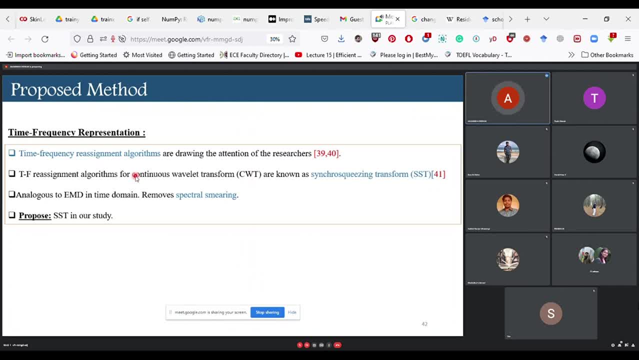 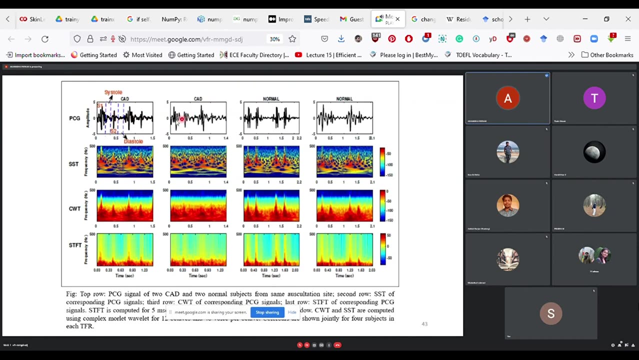 some advanced sec methods like wavelength transform or the reassignment algorithms are trying to be like more suitable compared to short time for your transform, the reason being in this figure. so these are like two uh. the signals for two cad into normal subjects from the same auscultation cells and we have the uh three time frequency representations. so first, 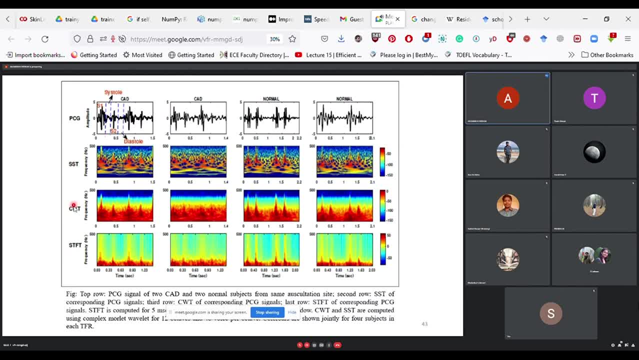 is short time for your transform. next is cwt, continuous wave layer transfer, and la la. and the last is single squeezing transform. this is a reassignment or we can say a post processing of the cwt. so in htft we can see that the s1 and s2 sounds are identified. you can see, but obviously 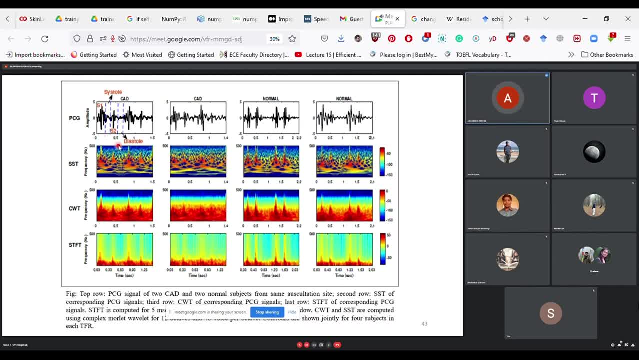 the localization and testing are basically the same, so the signal processing is very similar to the podcast. so in the case of the cwt, you can see that the signal processing is based on a short time period. time is not very good. uh, the see, the sound is spread. s1 sound is spread to a great extent, but 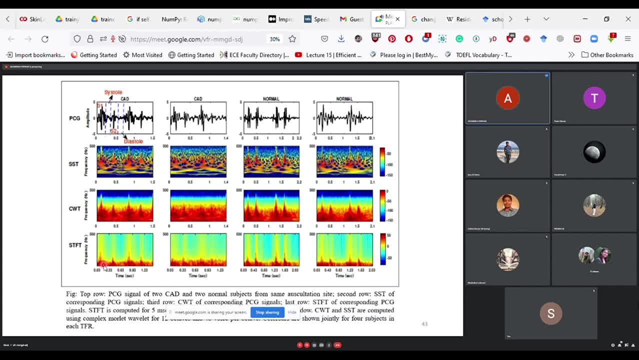 in, but herein we can see: okay, the that resolution. this is what resolution means. you are not able to localize it properly in time domain. next is cwt. okay, the sounds are localized well in time domain and frequency domain, but when you see that the power in the adjacent time bins is like not 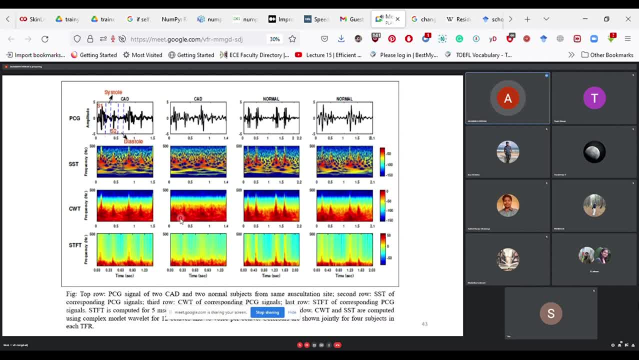 changing much, the reason being we perform convolution operation. so convolution operation is not just performing the convolution at a particular time instant, it is using adjacent bin also to perform that convolution operation. so even though there is there was least power in that particular time period, in that time instant, but still, since we were using adjacent bins, 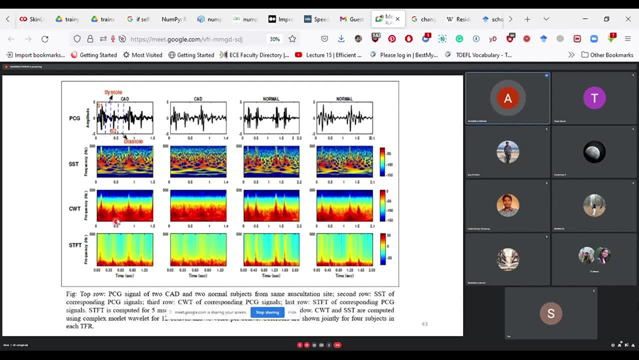 so their power gets added up to that, uh, that instant. so this is something like false information. it falls in the category of false information that, since they though, there was lesser power at a particular instant, but since we use the power of adjacent, which it get, it was represented here. so the change in the power content is less, but 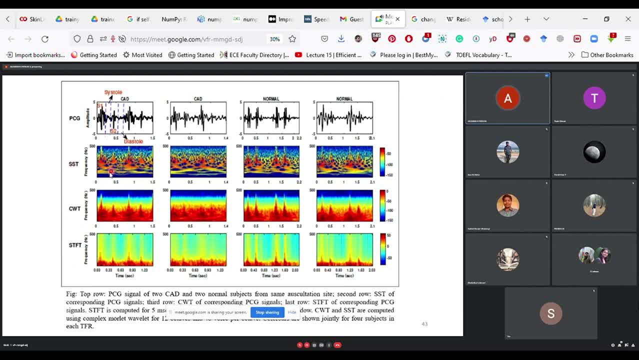 when we use synchro, squeezing transform of the ssd, we see that these changes are more evident. the representations are showing like more of a true content. okay, the power content changes as we move from s1 to s2, sound and so on. so this is like the reason. so one should not just go blindly but see like what suits the 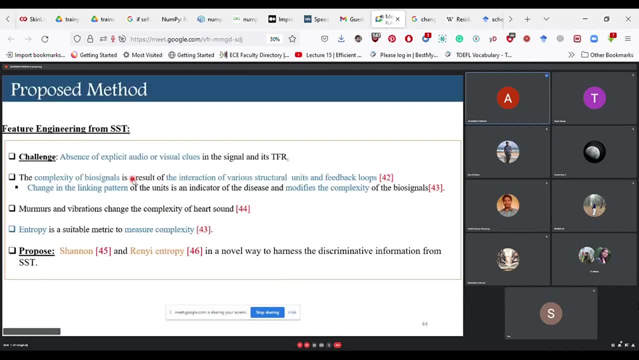 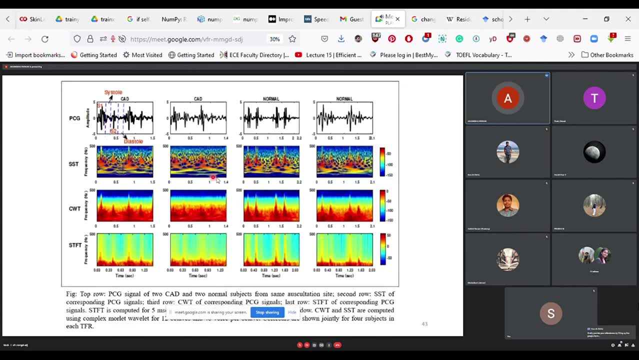 requirements better now. the next case is even so, see, even though we have this trying frequency representation, but our problem is yet not solved. can you say that which one is normal or which one is? can? no? so another level of feature mining is obviously saying that we have this time frequency. 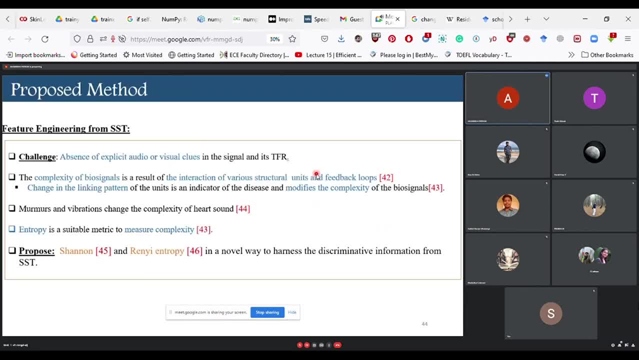 representation. but our problem is yet no. so another level of feature mining is obviously essential. now, uh, what to go for it? so in my uh here i tried to use the entropy. so entropy was not only the reason for taking the entropy was not only just based on what i wanted to use. 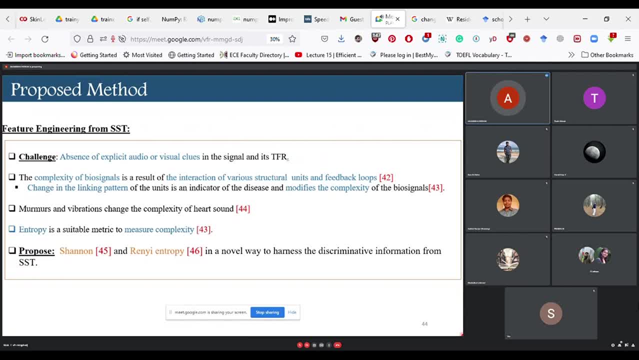 actually it was inspired more from literature. entropy is something which has been extensively used in all the biosignal processing. so what is entropy? entropy is something like: um, how surprised you are to for in with a certain processing of events. i will try to give a very simple example. if elections are going to happen and they're more ch and we know, okay, bjp is going. 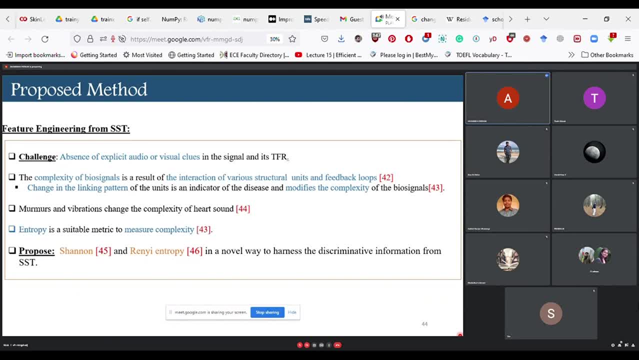 to win. the entropy of this event or this result is completely like very zero. okay, it is evident that bjp is going to win, but if apps all of a sudden comes up as a winner, this is how we are going to winner. this is a like a more informative. this is like a more surprising thing. oh my god. so there's. 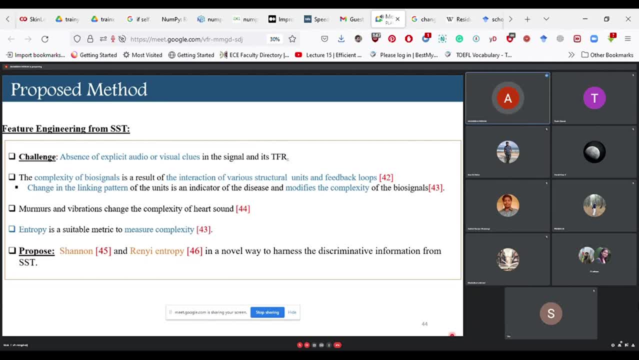 so much randomness, is it? so this event has a very high entropy app winning compared to bjp, isn't so the more surprise or more random behavior you see there, the higher is your entropy. so in what happened is that there was the usage of entropy in my literature, but entropy never. 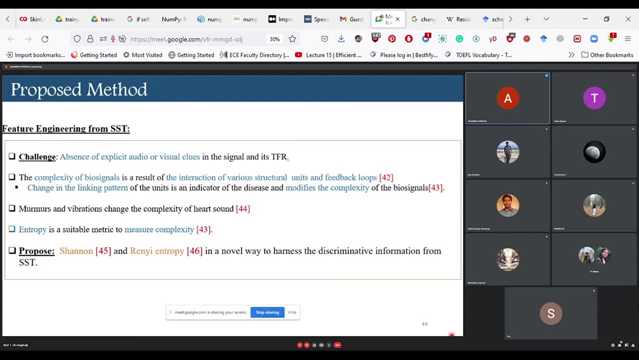 stood out as a winning feature ever people were using, but they were not coming with satisfactory results, which is like highly surprising. why is it not? entropy is like very a good feature to display the disease states compared to normal state, because disease in disease, you get like surprise. 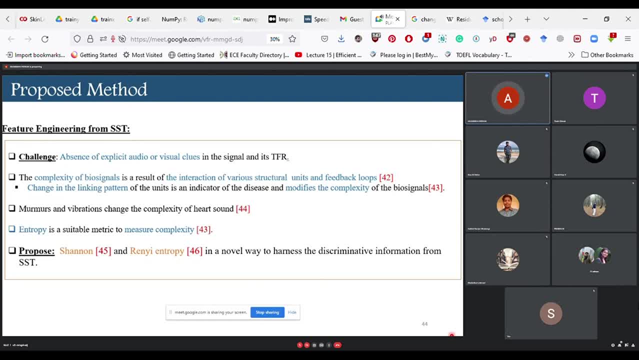 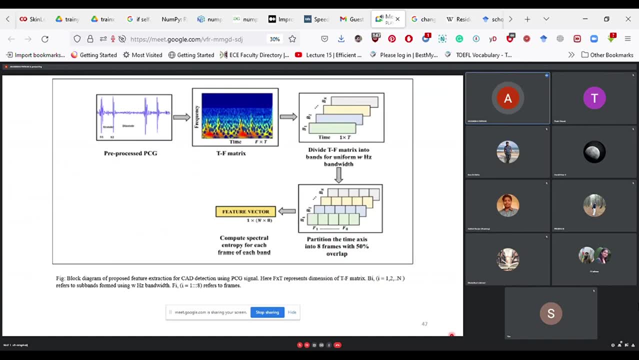 oh, this is like very rare occasion, so in top is high compared to a normal event. so what, uh? i decided was to go with us. what different approach to use? entropy? so? so this block diagram shows it. so instead of using the like um, what i did was: this is a time frequency matrix. i broke it into bands in the frequency domain. 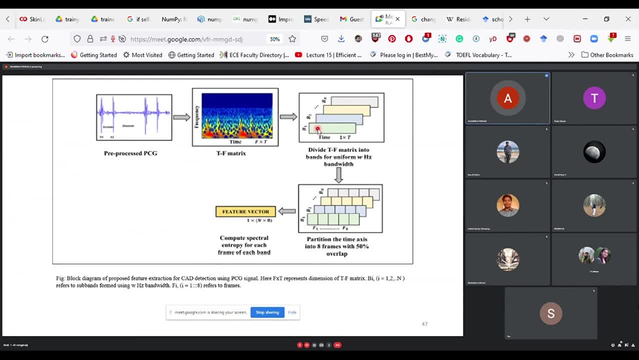 as done previously, and then divided along the time axis. also i divided into frames, so overlapping frames. i took just eight frames with fifty percent overlap. so entropy was computed for each frame in each sub band. so in band wise also i was trying to check out all the precise. 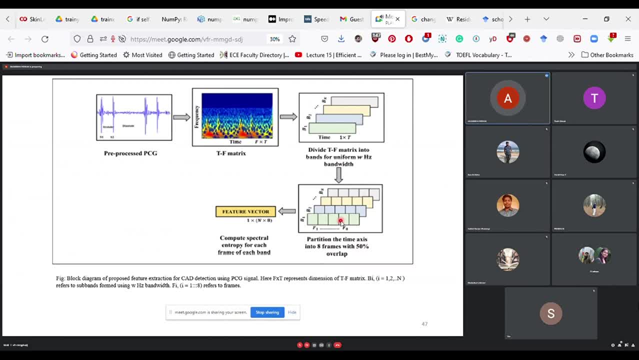 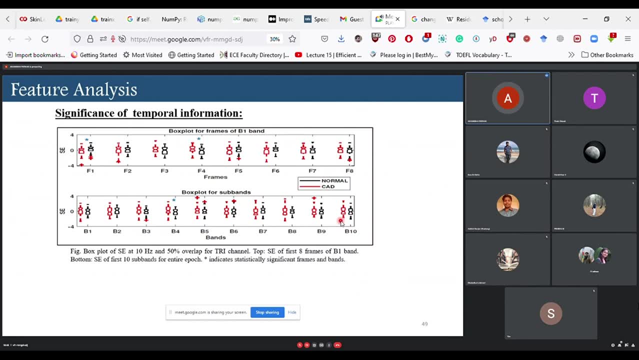 places where i could get signature as well as in time also. so this is like the one, the way which i tried to use. i did some statistical test again by as to convince myself and the readers like why it should be like a frame wise approach rather than just computing the entropy for the entire. 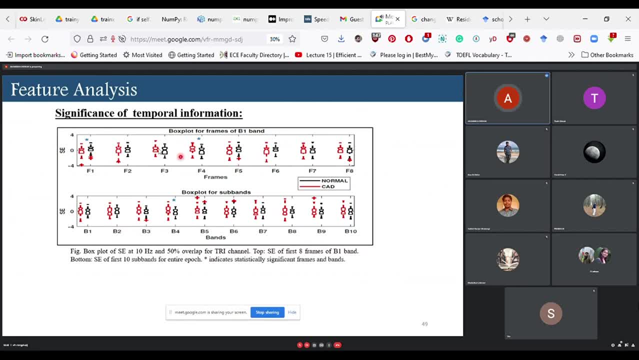 epoch at once. so for example, this a statistical test. so upper box plot is showing the the entropy for eight frames of the b1 band, but the lower box plot is showing the entire entropy computed from b1 band, like, irrespective of any frame, for the current complete epoch. so what we see, even though the frame f1 and f4 of the b1 band are like 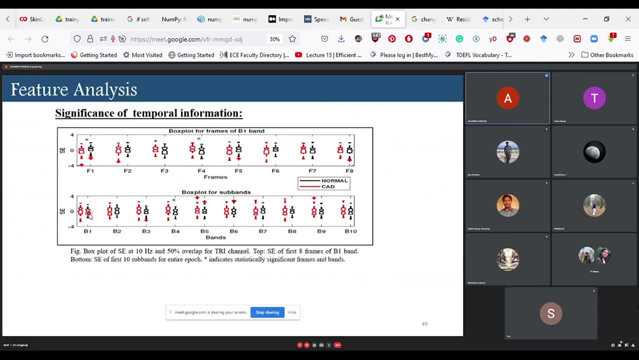 discriminative or statistically significant. the entire band as a whole is not statistically significant. so this is like the main point. okay, so the information or the entropy is discriminative only at certain phases and not throughout the cardiac cycle. so these are like i'll say one should go for: uh, identify like which phases are discriminative. 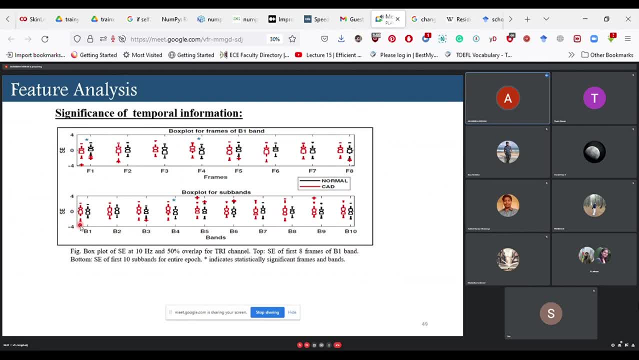 for example, because in our case the signals are so weak that you cannot just go through the entire signal and use it as a discriminative pattern. you need to magnify and zoom your use cases where you should use in either time or be in frequency. um, i will not go through it. 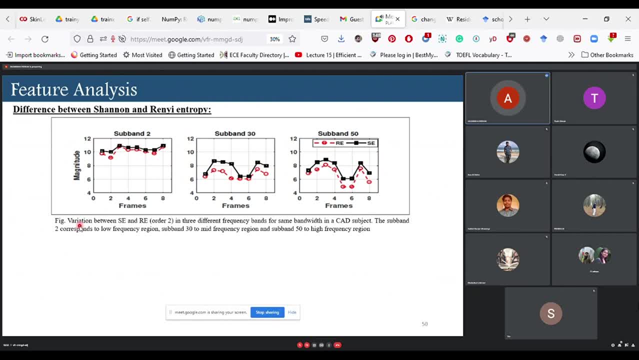 okay, so this is just like showing why i am using two different entropies, shannon and rengi. so these are like very interesting. um, so what happens is in these two entropies are redundant, but they are also, uh, complementary, but they are redundant in like lower frequency. 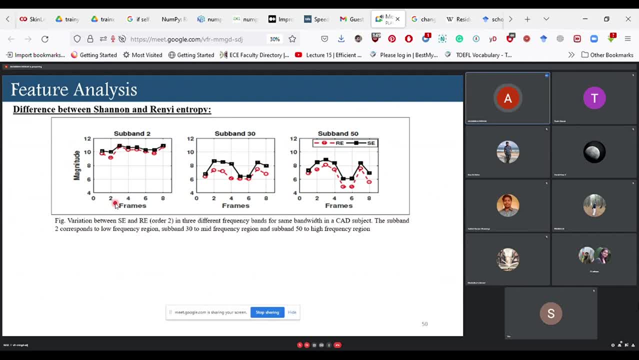 zones and they are complementary in higher frequency zones. so this is basically based on the formula which we use for them. so one should try to explore more specifically so more options. we should obviously try for more um complementary aspects, but sometimes little bit of redundancy can also be used or adjusted to like you can go for this trade-off y2, which 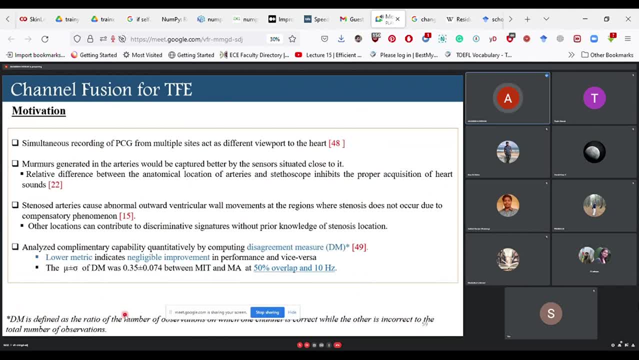 one to use. and last and the next thing in this time, frequency representation- was that i was always hoping to use my multi-channel informations collectively. so in the spectrum representation, obviously i went with the cross spectrum based approach, which was automatically using multiple channels in each phase. but here, since we are dealing with feature extraction of, 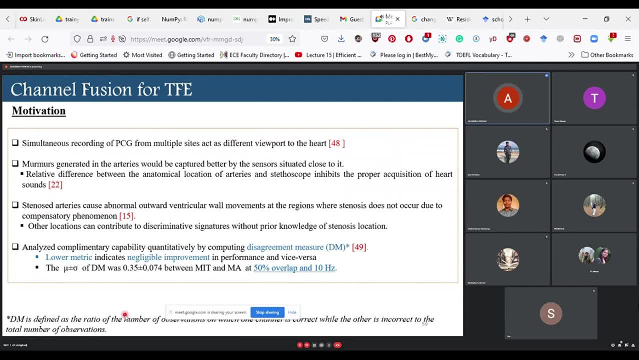 each channel using time, frequency representation and the entropy. so i went with, like, fusing the channel information at score level. so whatever scores we get from the classifier, or the probabilities, were fused to obtain, uh, a more strong decision, whether the signal is scared or normal. so again, this is like more of a 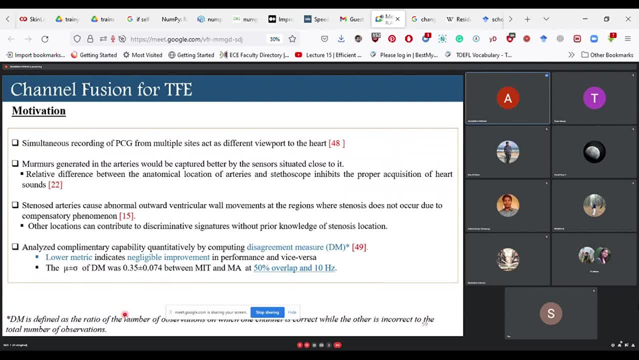 physiological based, uh, intuition. so what is happening is like different sites are capturing different signals and the database is also like vast, so you don't have a homogeneous data. some patients are like uh, very, very fatal stage of the disease. some patients are like very initial stage. for some patients it might be that all the three arteries are stenosed or blocked. 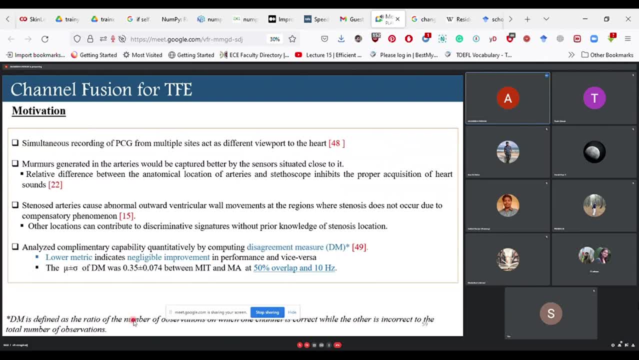 for some patients, only one or two arteries are blocked, so my data is not at all homogeneous. so this is like first, so i should use information from all the sites collectively and basically, and moreover, since i'm, if, for example, for testing, making a testing pattern of this system. 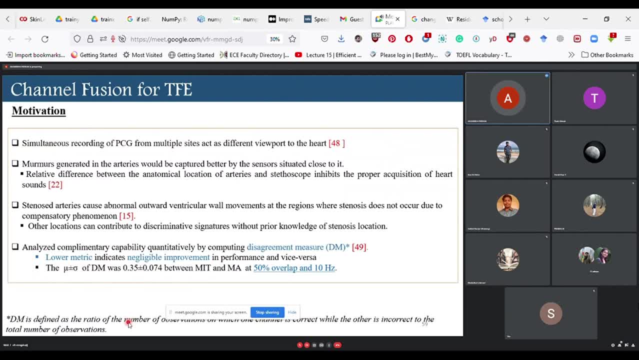 i don't know which site or which arteries also blood, so i want to use information from all the sites because i don't have any prior information. if i'm not going through angiography or a standard test, how do i know that which site is more prone or will be more favorable to identify the disease? 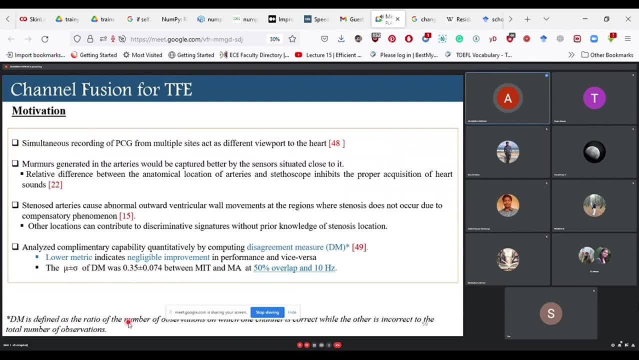 so that is a multi-channel approach. was user here. instead of just relying on a single channel vote, i will go for a combined vote. so fusion is obviously a very a good approach, but depends the type of fusion you are going with. so when you are going with fusion, you can always go from beta level to 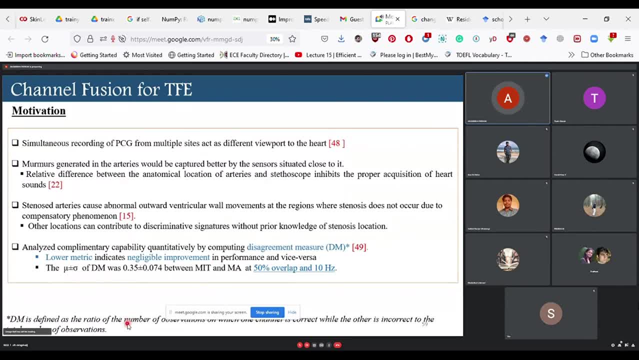 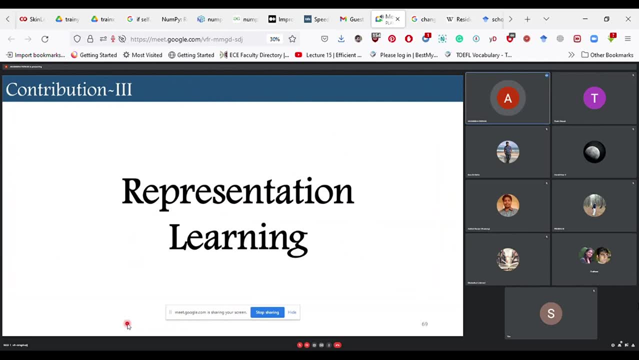 out to score level or output level fusion, whichever suits their purpose. last but not least is the representation. i hope we have some time left. yes, ma'am, yes, efficient time left. so next is the representation. so my first two approaches were based on handcrafted feature based, of course. obviously, a handcrafted 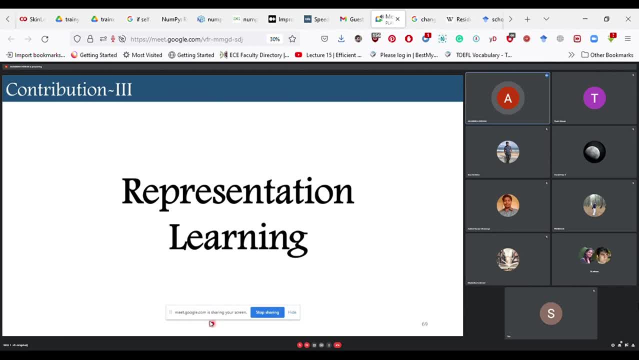 feature-based approach requires a lot of clinical understanding, which needs a time and effort to go through the literature, understand the bio. being from engineering domain, you need to study the bio and relate it with your general know-how of signal processing and the physics, like how to understand it. so and related, for example, if i am using entropy, i need a intuition of physiological 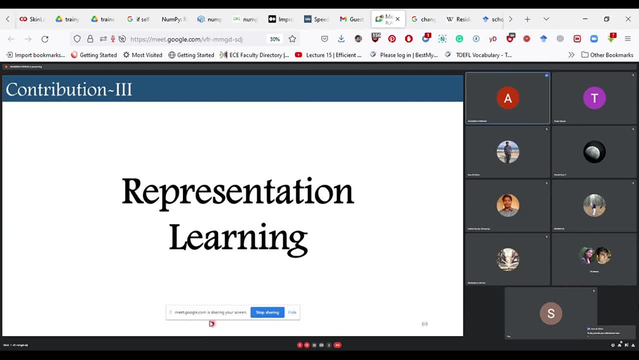 understanding that, why i should use the intro. it is not like using a black box and i am just using the entropy randomly. or why am i using the cross power spectrum density? i have a understanding that, okay, the heart sounds are transmitted, but in order to use these concepts, i had to go through a lot of 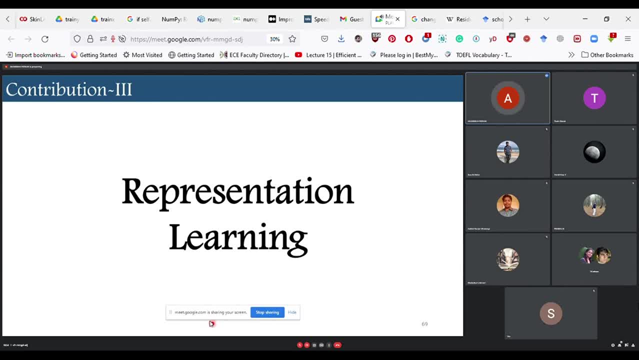 thorough detail of the system or the heart sounds at the cell before diagnosing the disease. so obviously these demands are fresh. a lot of effort. in this context. if we go for representation learning, at least you will be getting rid, though it is not very good because it is a like a sort of black box via which features are being used, but still. 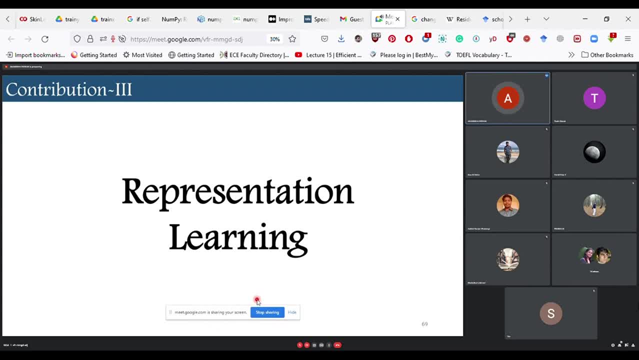 representation learning is something which can help you in this context, wherein you will automatically be learning the features. so, um, as already so, but another advantage of the representation learning is it is not always like going to happen that, whatever physiological understanding you have, you can relate it with some technical domain information in order to use it. 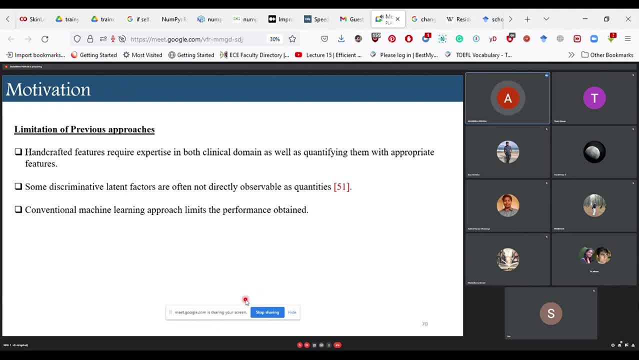 so, for example, if i am using the uh, the entropy, i know, okay, the complexity or the signal changes, so i will, i can use entropy. but there might be other factors also with which i cannot come up to a quantitative quantity that, okay, i should use this metric or quantity for analyzing my signals. so 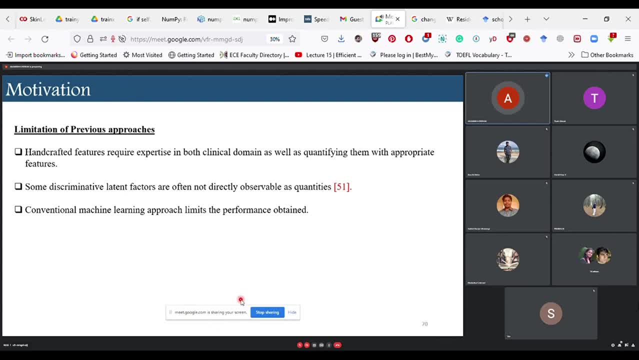 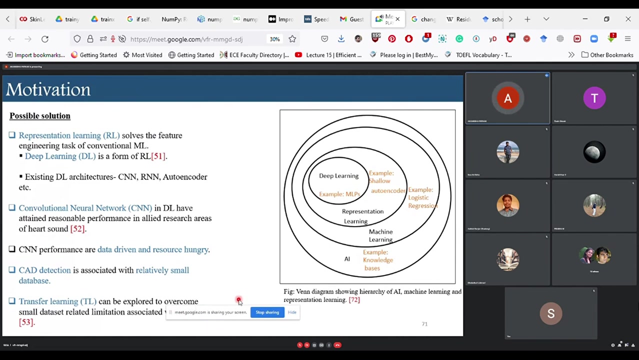 this. bridging the gap between the clinical information and the engineering domain is also essential. with somehow in handcrafted, feature-based approach, we are not exporting completely. so in this context also, i think representation learnings is beneficial to use. so as we all know, i think, what is like deep learning. so deep learning is just an example. 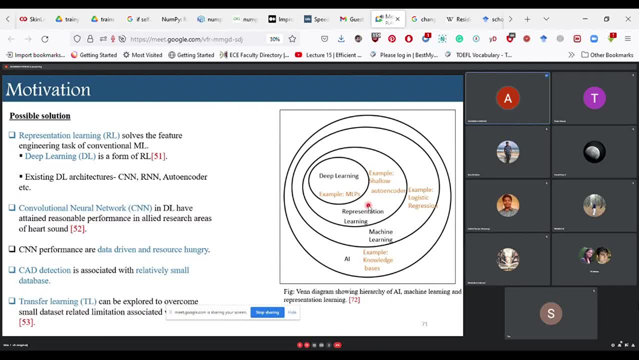 uh in a subset of representation learning where we are not only learning how to map the features to the class level but we are also learning the features from the input also. so cns we have, uh, we all know that they are very data driven and resource hungry and so and medical and i 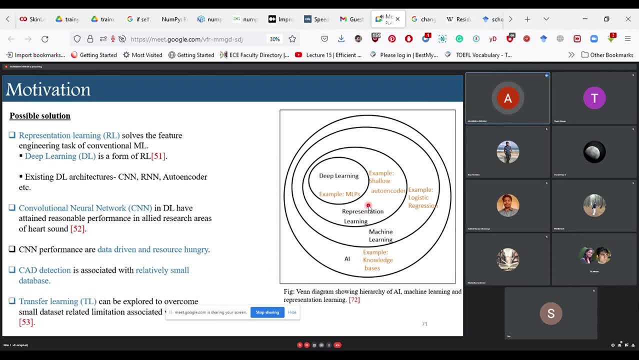 know. in our case especially, we see that we have a very small amount of data, like not even 10 000 samples, it's just in 960 samples. so obviously our cnn making your own cnn training- it will be a like very difficult task. so we have tried to come up with using the concept of transfer learning. 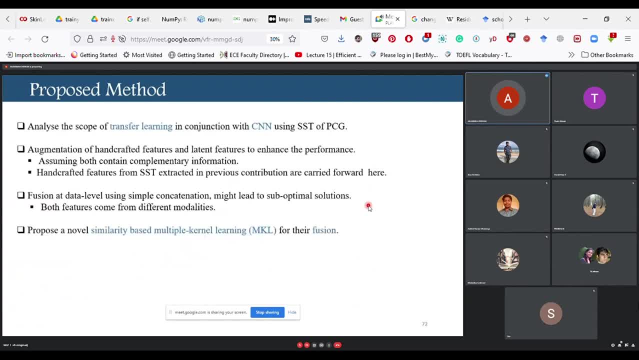 okay, so transfer learning, but before going with it, i would like to tell that, uh, another experiments experiment which i wanted to use it on my own was: i wanted to see how the augmentation of handcrafted features and these trans and these representation learning features help us to and deal with this diagnosis. so the source of input was same, that is, i wanted. 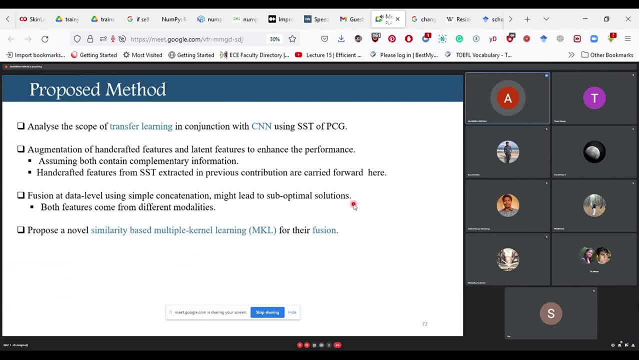 to use same input, uh, for the handcrafted feature, that is, the time frequency representation for the and the same representation or the input for the cns, and we wanted to see, like, what both of these systems are extracting, how different is it and whether they are redundant or complementary. 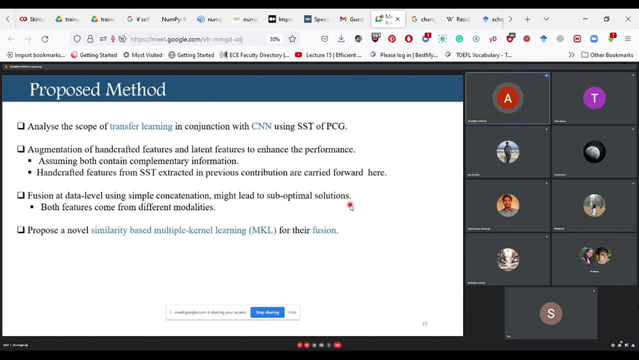 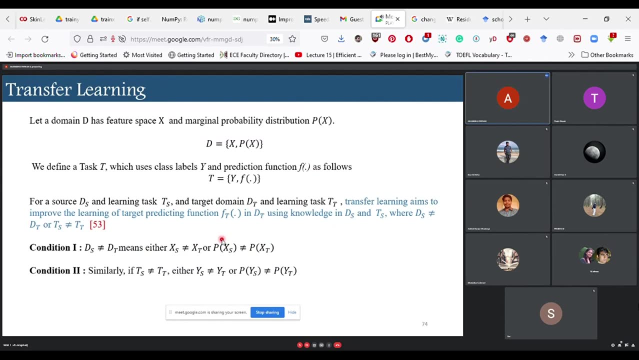 so the few. for fusion, i am basically using a kernel based approach, which is known as, like, multiple kernel learning. now this will be a little bit interesting, okay, so a quick go through for the transfer learning. transfer learning, basically, it is not. first of all, it is not only confined to your cns, i would like to say, it is a general topic. so transfer learning is. 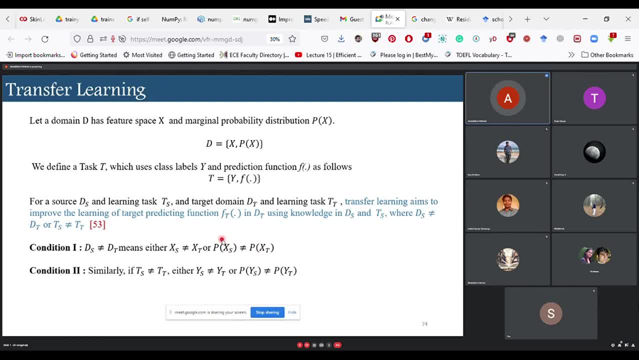 basically, you have a some problem or domain which has some feature, space and some probability distribution of the classes- okay for. and then you have another task or another domain which is defined also, uh, using the same set of things. so transfer learning basically aims to use the knowledge in 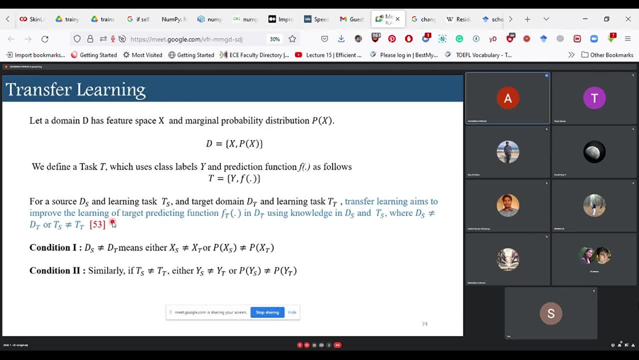 one domain and and to use it in some way in the other domain, but on the condition that either the samples are not the same or the probabilities are not the same. similarly, another condition would be, maybe, that the task or the class classes are not the same in both the source and domain source and. 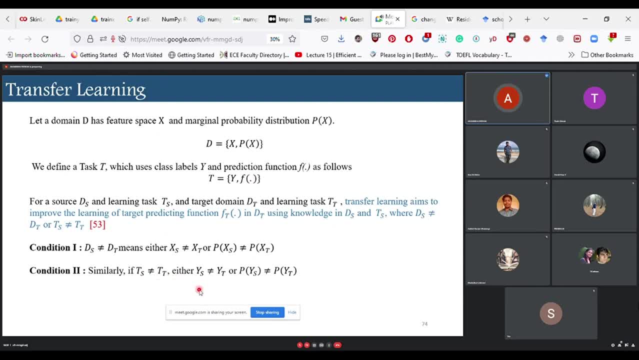 class. remember that the class is not the same. both the domain, source and domain is different. so, first of all, the same sort of things are that um transfer learning is not the same and other of the other, and the task domain, all the probabilities are not same, so something would be matching or something. 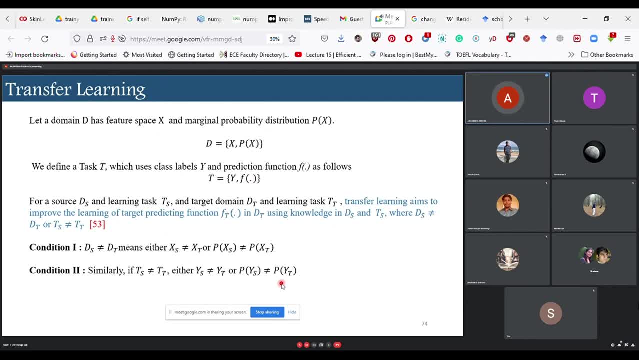 would not be matching. so this is like the concept of translation. you will not be using directly cad and normal as source, one source and then cad and normal from another channel. this is not transferring. you need to expect information from another domain to use it somewhere in the same another, one more domain. another question arises: what to transfer and how should we transfer? 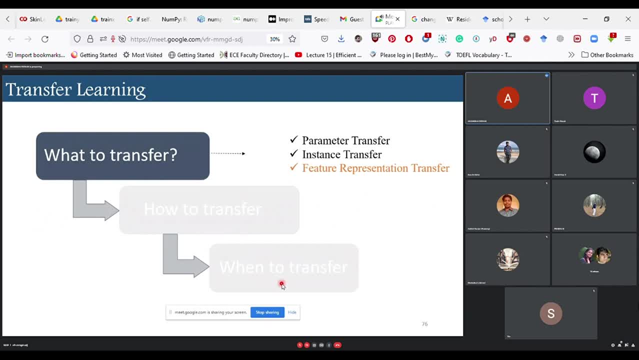 when should we transfer? so what to transfer is like: you can transfer the parameters of the system, or your, your train models, or you can transfer the instances of your data, if you think so, or you can transfer the features. so in our case, we are transferring the feature. 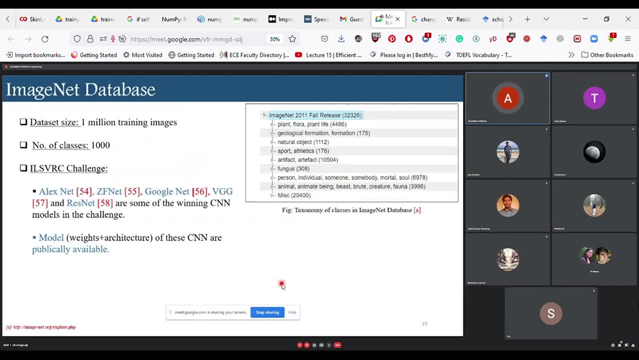 representations and what is my source domain? my source domain is an image net database. so image net database is a very big, one million image based database with approximately thousand classes. the classes also varies from, like plants, it is like numerous thousand classes a lot from. i have listed, like some of the classes here: animals, persons, fungus. 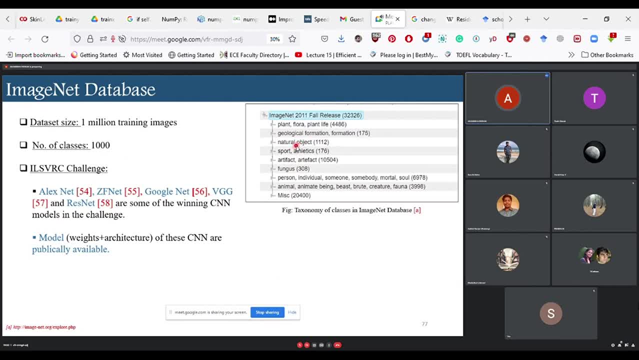 artifacts, sports, natural objects, like. it is multi, highly like multi-class you cannot. there is not even a one um hierarchy that such set of classes are there. there's multiple. so and we have some of these classes which have already learned how to classify the data into these thousand classes. 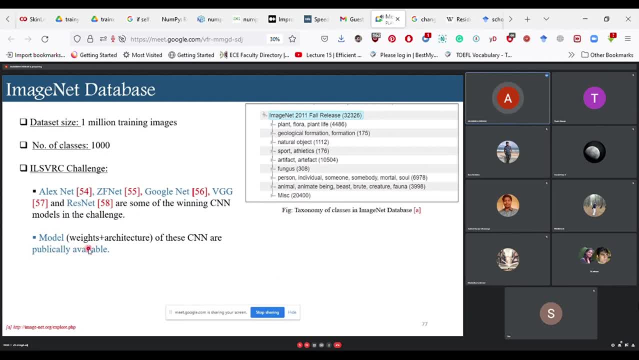 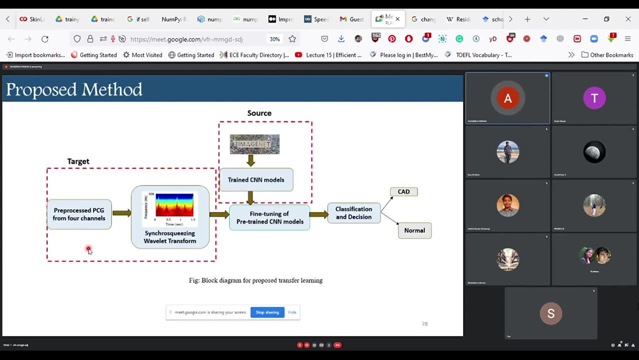 so we have the model, that is, the weight and the architectures of these cns publicly available. so what we do is like: this is like the basic block diagram. we have the target, which is the my pre-processed pcg signals of phonocardiogram signal from four channels and i 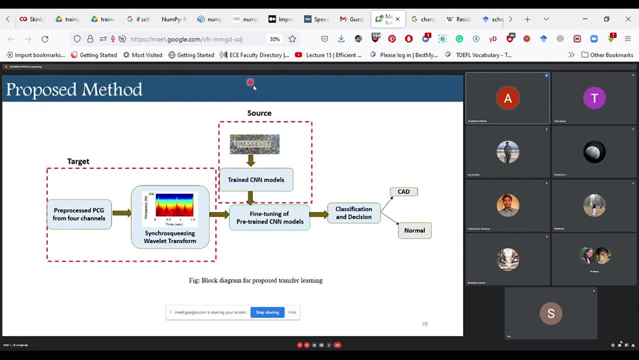 have computed that this includes squeezing wavelength transform and the source is the same. so this is the pre-trained cnn data and the trained cnn model. now i will use this model weights and architectures to fine-tune those pre-trained cnn models and then use them for classifying cad and normal- just two classes, which is my target or task function. 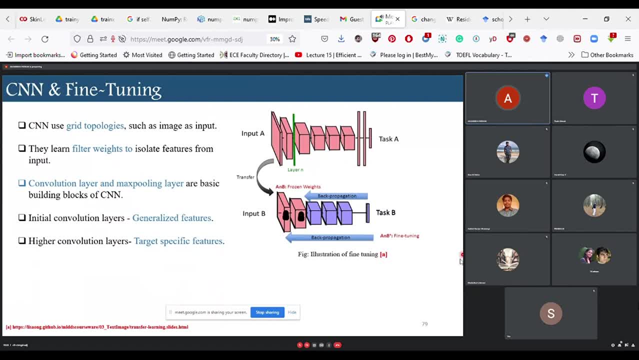 so a quick go through. how does this fine tuning takes place? so suppose this is a cnn for task a or an input a. so what i do is for transferring. i retain some of the initial layers of this cnn. so cnn's are basically neural networks which work on. 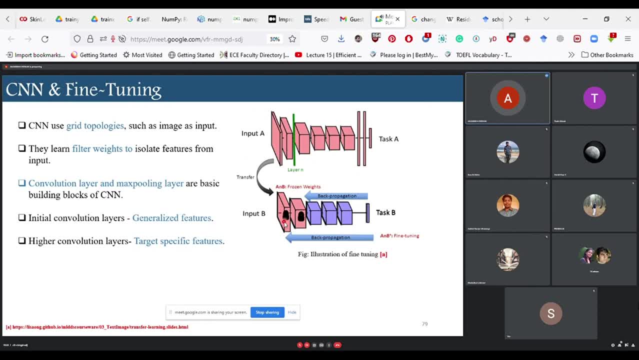 grid-based input. grid-based input could be a image, 2d image or a three-dimensional or multi-dimensional matrix- grid-based, which has some like rows and columns. it works and basically its motive is to extract the features from this grid-based input using the concept of image processing. that is it. 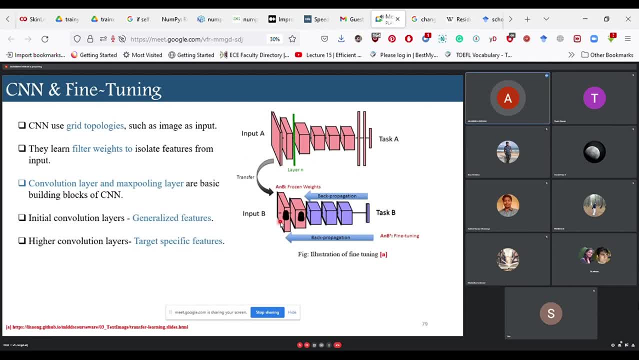 identifies the field it identifies or learns the filters which are used to extract features from this image type of input. so the general theory is that initial layers learn the generic features. generic features are like identifying where are the edges, where is their contrast, or like what main outline of the image, main building blocks, and then task specific feature is like 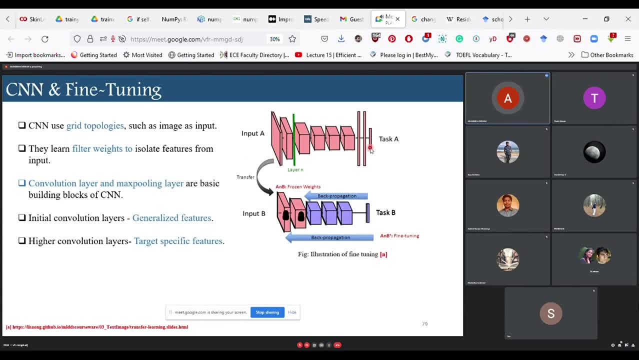 identifying where the tree is, where the house is, localizing it more prominently. so this is the case. so how do we transfer it? we transfer some initial layers so we always want some edges okay to identify. i want to demarcate where is my s1 sound, where is my s2 sound? little bit some boundary, where is the noise or like. 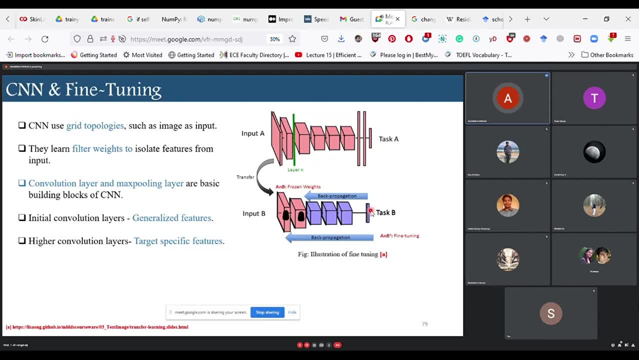 and then finally leading to water, like: where is? how do you know where is cad and where is normal? so we retain some of the initial layers so that we don't need to train our system again, and we obviously we don't have data that much to train. 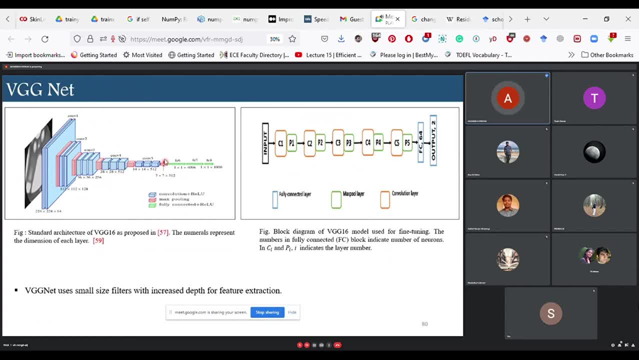 so we have used bgg net. so i retained all the convolution layers, five condition, and just replace these last uh fully connected layers fully connected layers with the last two with one single fully connected layer and the output layer with a single output, a layer with two neurons. 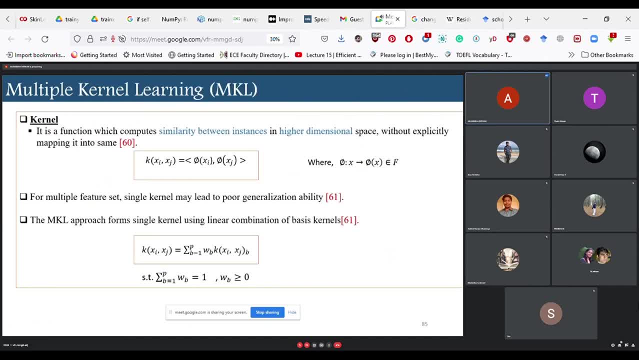 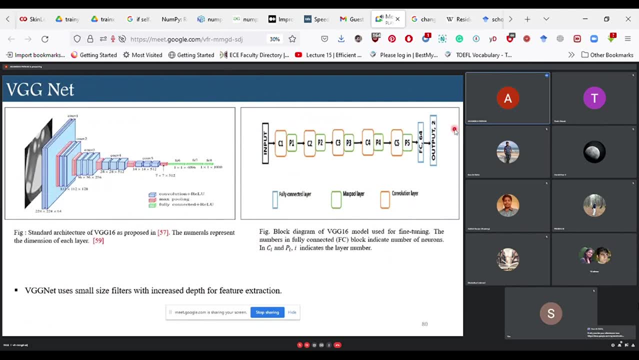 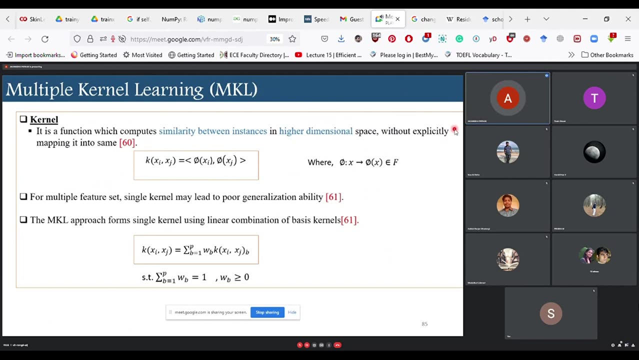 so this is the process of fine tuning. okay, so once we do this fine tuning, we get, we restrain our system and get the results. okay, now comes like this concept of multiple kernel learning. since already stated i wanted to, this is my curiosity to see what the system is learning using cnn and how much is it different from my. 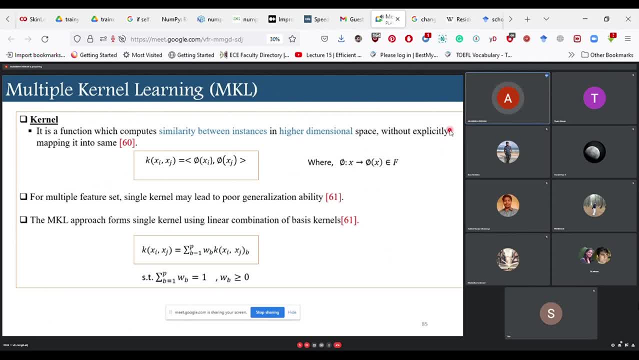 handcrafted entropy based features which i have used in the previous contribution. so um kernel is a very- uh, i will say a very- simple, yet advanced function. basically, it is computing a similarity between two instances, but in a higher dimensional space, and it is not explicitly mapping it into the 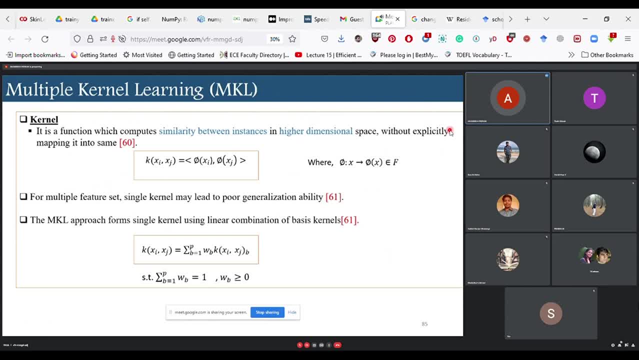 higher dimensional space. but the kernel function, which is it? it itself gives you an intuition that it is mapping into a higher dimensional space. so, for example, in rbf kernel the formula is like: e raised to the power, x minus y. so x minus y is basically taking the similarity. okay, x and y. how? 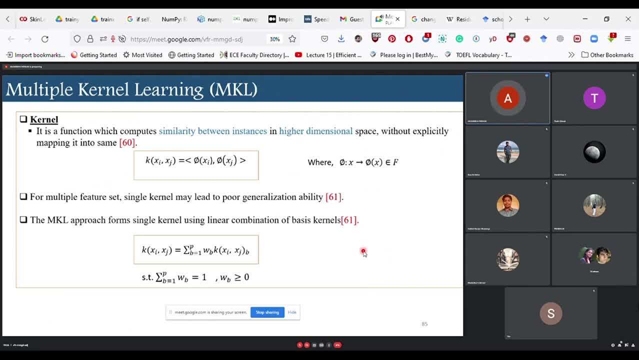 much similar or dissimilar they are and e, raised to the power of that similarity or this similarity, is basically mapping that similarity to that thing to some different way in an exponential space. i'm not watching the similarity in the linear domain, i'm watching the similarity in exponential domain. 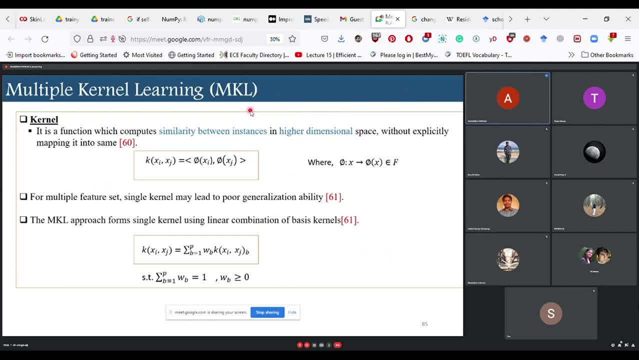 but instead something is being found in that kernel to be able to map the data to a higher dimensional space, which is the same as the correlation between the two instances of kernel. so when we don't want explicitly or manually to map the data to higher dimensional space, 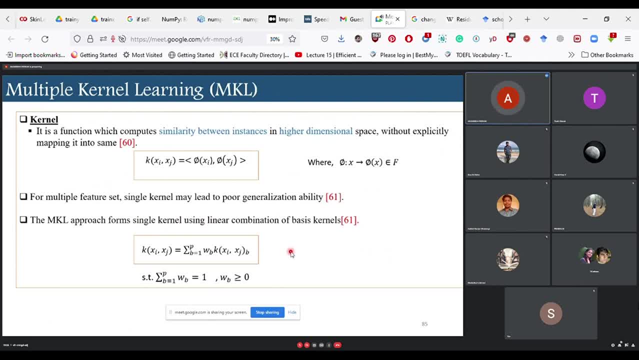 we use kernels to do it. sorry, now, what is multiple kernel learning? the main reason actually behind going through a kernel based approach was that, uh, since i used svm in my machine learning based went for the kernel. so what happens is, if i think, each and everyone, if they are anyone, 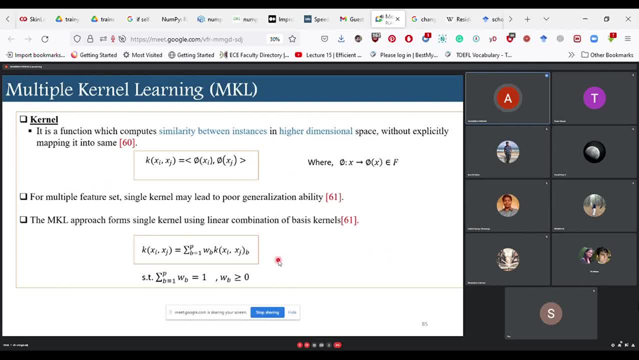 who is who has used the machine learning will surely have used the svm. so in svm we use this kernels for classification. so usually we don't. for example, we have two features. if we have heard about the iris data set, we have sepal length and petal width, for example. 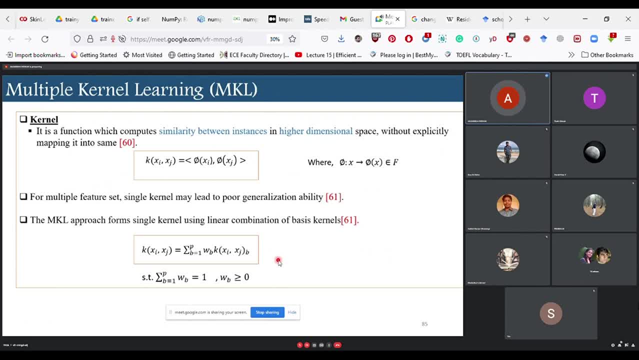 and we are just using all these features and using one single kernel. so it might be that the value range of petal width are different from the length by sepal length features. so what is this? we should use individual kernel for each different types of features so that 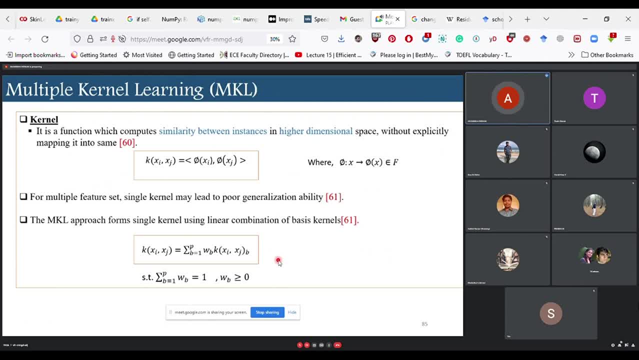 you can see the similarity properly, like how much similarity is there between the instances using the sepal length compared to petal width. so it is like map watching the similarity more in a homogeneous data rather than in a heterogeneous data. so in this context, multiple kernel learning is. 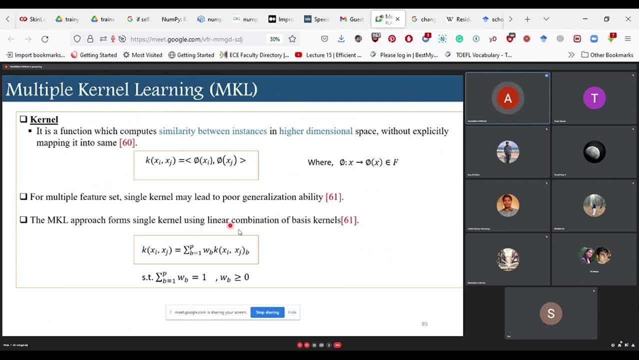 a good thing because it makes a single kernel using linear combination of other basis kernels. so what is it like? you make kernel for petal length explicitly, you make the kernel of petal width explicitly, sepal length explicitly, sepal length explicitly and with the. What is the best way to do this process? also, question is: is there any security rule of kind? so 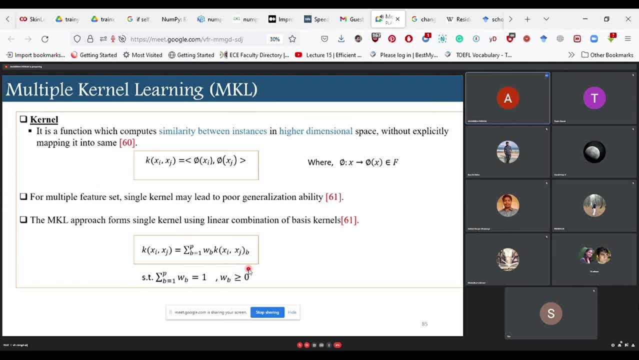 explicitly. You have all these four types of features. You make one kernel for each and you just add those kernels with some linear combination of weight to make one final single kernel, on the condition that the weights of these kernels will sum up to 1 and all the 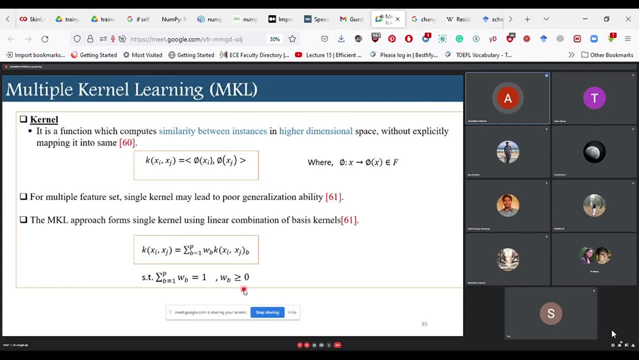 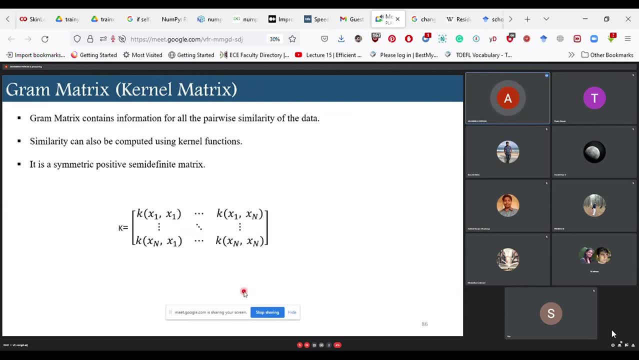 weights should be more than or equal to 0.. So this is the idea of multiple kernel learning. Then this is a prerequisite. So gram matrix, or we can say a kernel matrix, is basically a matrix which contains the similarity of all the pairwise similarity for the data. 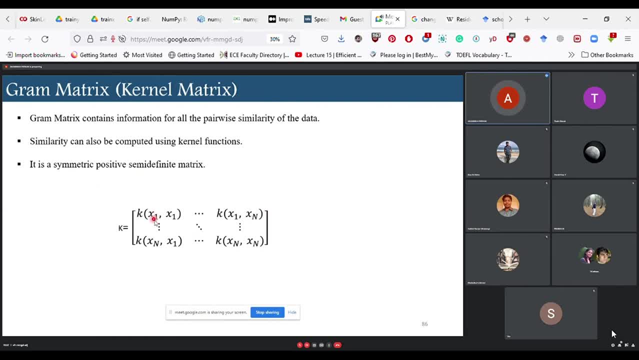 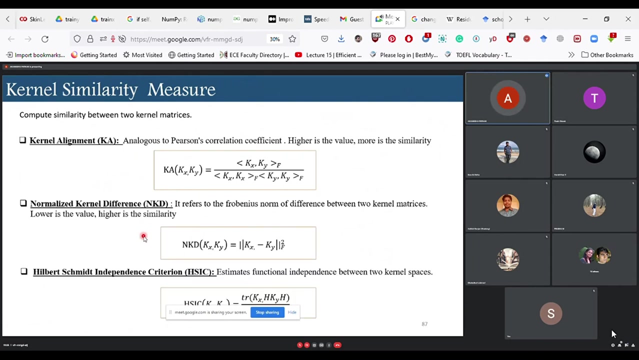 So since if we are using some kernel function, so it becomes a kernel matrix and it is like a positive, symmetric, positive, semi definite matrix. Now the comes the question like what kernel similarity measures we need? So the idea of kernel similarity measures basically is like I want to compute similarity. 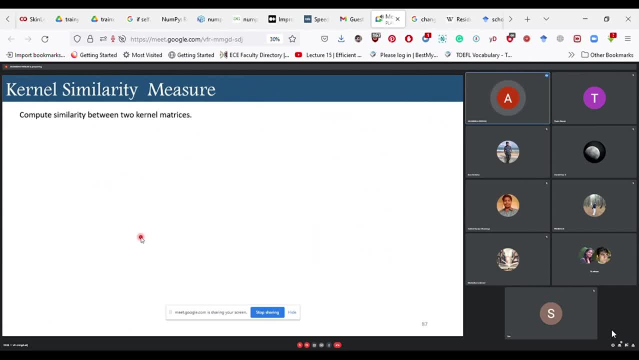 between two kernel matrices. now I have one kernel matrix, suppose like this, and another kernel matrix also. Now I want to see the similarity between these two kernel matrices. So till now we were dealing with instances. For instances, we have the kernel, but for matrix. 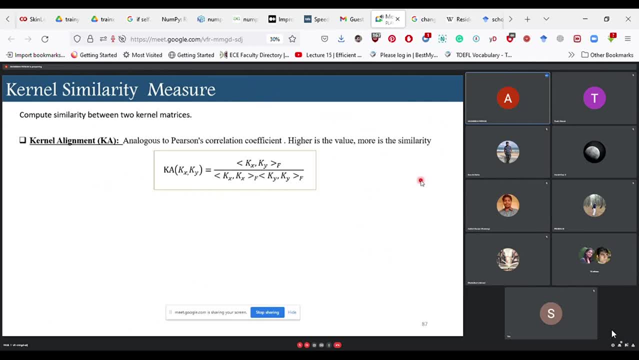 we have the kernel similarity measures explicitly. So these are some three kernel similarity measures. It might appear very complex, but it is very simple and it is analogous to correlation coefficient. So you are just performing correlation between two matrices. So when we deal with matrices, we use Frobenius norm, For example. 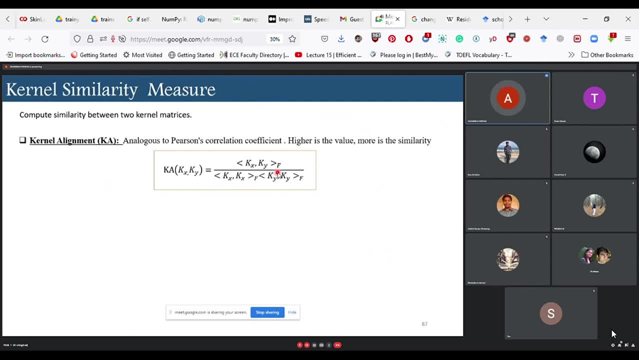 for a vector, we use L2 norm or the Euclidean norm for getting its absolute value. For matrices, we use Frobenius norm. Next is normalized kernel difference. It is just like taking the difference of the matrices and using their Frobenius norm. And next is like Hilbert-Schmidt. 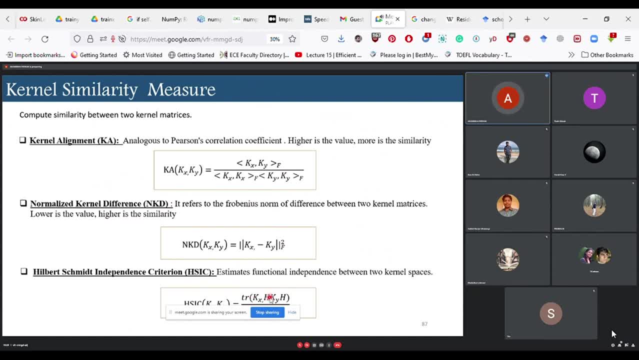 independence criteria. So this is like computing the cross covariance of the two matrices. I will not say that these are the only ones, but these are the ones which I have undertaken for computing the similarity. So this is the difference between the two matrices. So I will not say that these are. 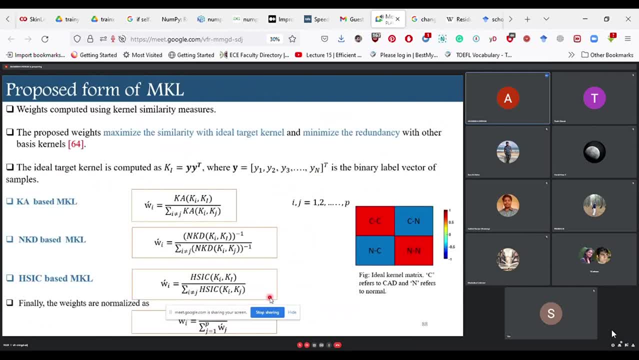 the only ones, but these are the ones which I have undertaken for computing the similarity. Now it is like: what is the idea of? how am I going to use this kernel similarity measure or this multiple kernel learning? So consider, you have listed your, you have made an output. 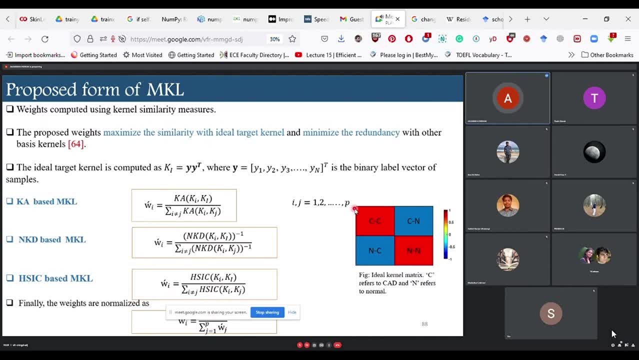 ideal kernel matrix which have cad instance first of all lined up in this quadrant, and next quadrant you have the normal instances. Similarly, here, also in the row wise, you have the column wise, you have listed all the cad instances and then again the normal instances. So, ideally, what should happen when you compute the similarity of cad instances with cad instances? 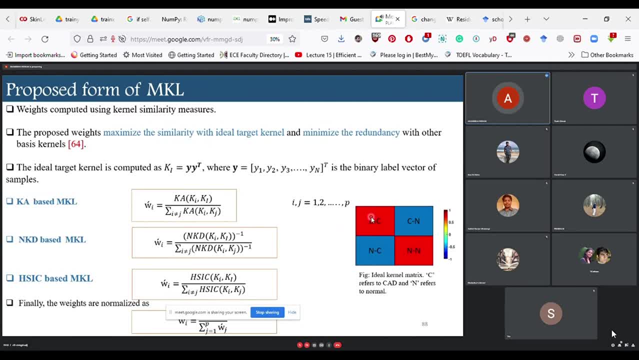 they should appear as like high. The similarity of instances from same class level should be high compared to similarity of instances from different class levels. So this is an ideal kernel matrix. This kernel matrix is simply composed. So I am using- currently I am using just the output levels. So, for example, you have 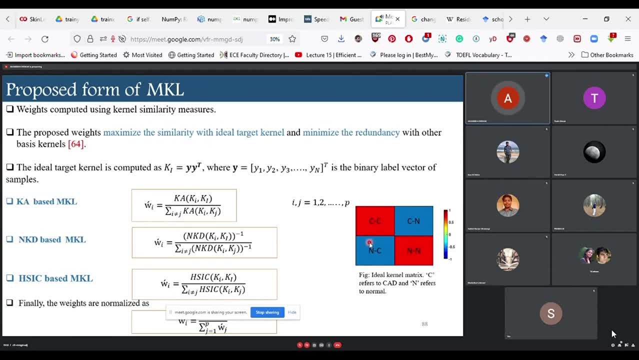 used 1s for cad and 0s for normal, or minus 1 for normal and 1 for cad. So first hand this quadrant and this quadrant should be 1 and the diagonally opposite should be 0s. So this is an ideal kernel matrix. Now what am I doing is so? for example, I use how, how, 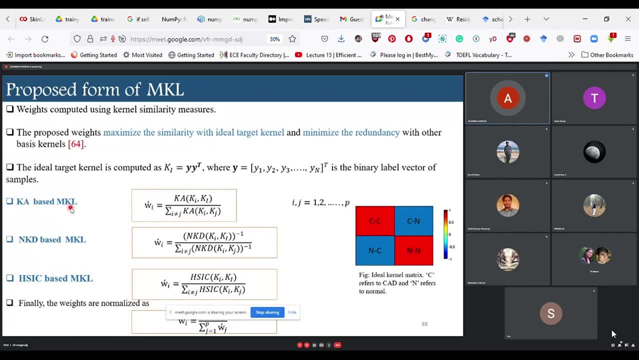 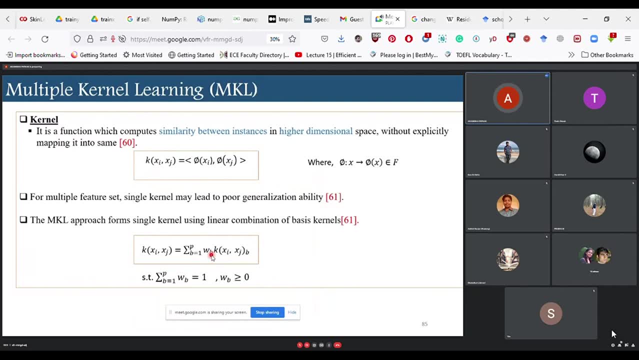 can I use this as my matrix? So the basic task here is to estimate these weights for using the multiple-kernel learning. I want to know what should be the weight. I have the information that what should be the kernel matrix, so in my case I will be using the kernel. 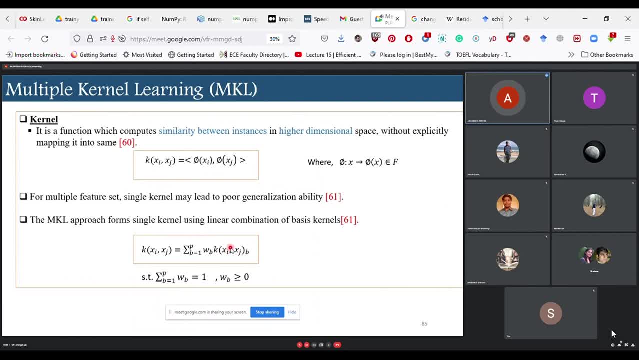 matrix of the entropy Shannon entropy. one kernel matrix should be for the Renyi entropy and another kernel matrix would be for the embedding which I will be using. the kernel have learned from the cnn's so i have three types of features and i have computed three. 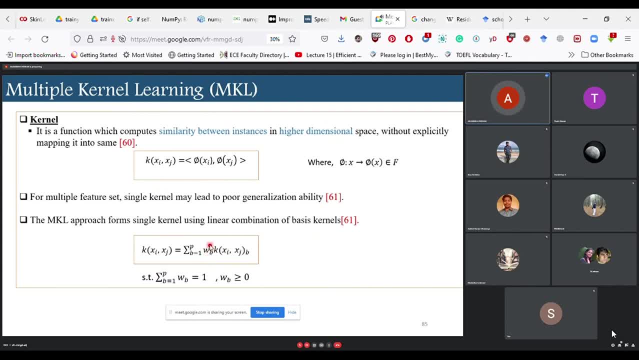 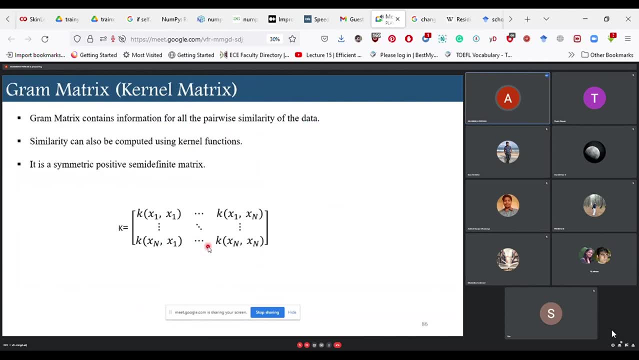 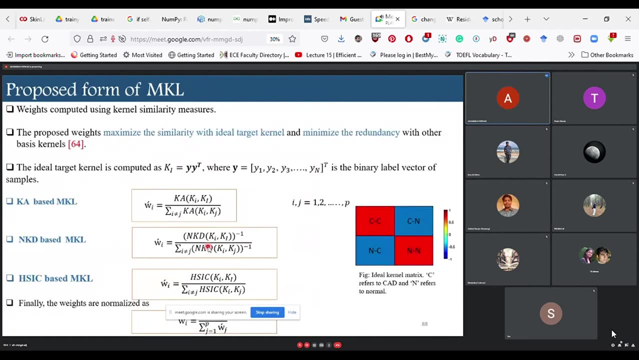 kernel matrices for them. but now i want to find out what should be the suitable weights. so for finding these weights, i am using these similarity measures: kernel assignment, alignment and denormalized kernel difference. so the so my basic approach is that the each and every kernel which i am using should maximize the similarity with the ideal target. 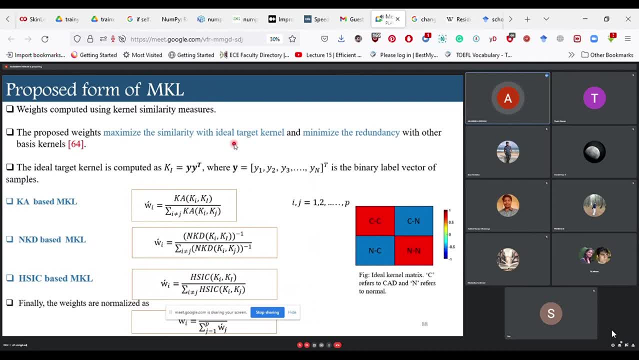 kernel, but it should minimize the redundancy with other basis kernels. so the feature which is more contributive towards classifying should get higher weightage, but it should also accompany the fact that if it is redundant with the existing features it should accommodate that factor too. so in any sort of machine learning 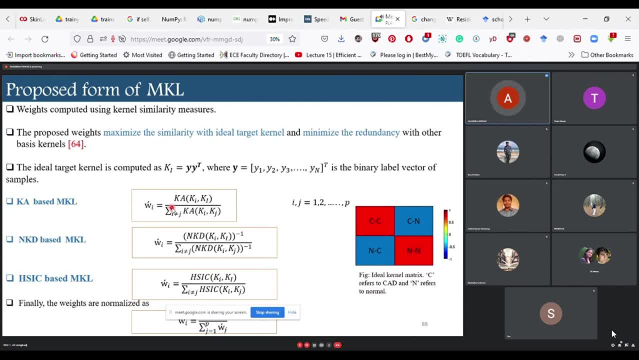 based approach wherein you are trying to find some features or any sort of other. i will save like method. redundancy and the relevance are like two terms which go hand in hand. everyone wants to be relevant with respect to the target problem, but redundancy is also one of the criteria so that you 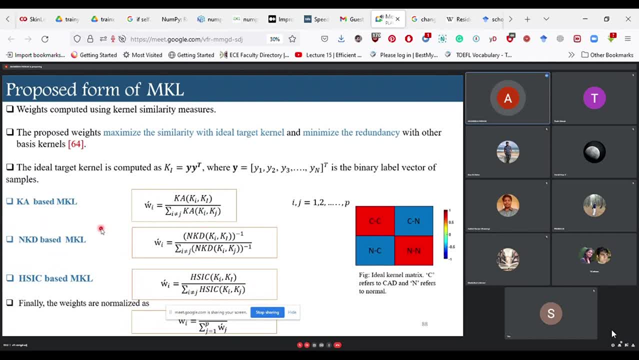 understand what the instability is being passed up and not to deceive theedelta j letter distinct LC h function: uh, so detract that form of type description. young J learned Class every year and that got into register data is be always bear manifested as a policy in class assignment program only if it is done with. 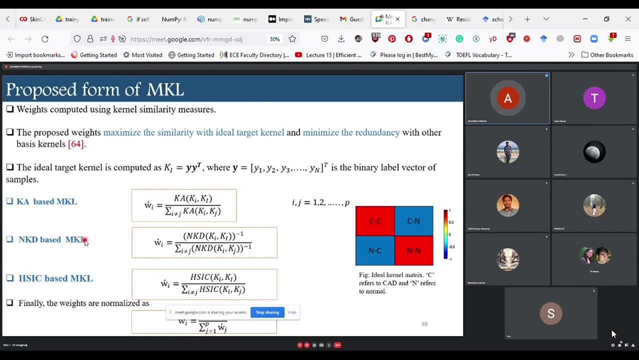 writer, depending on whether vendors use random variable or method, apartment kind of kind of i'm trying to, since i don't know whether embeddings are more in discriminative or my handcrafted features are more discriminative, so i'm trying to estimate the weights automatically. okay, the system. 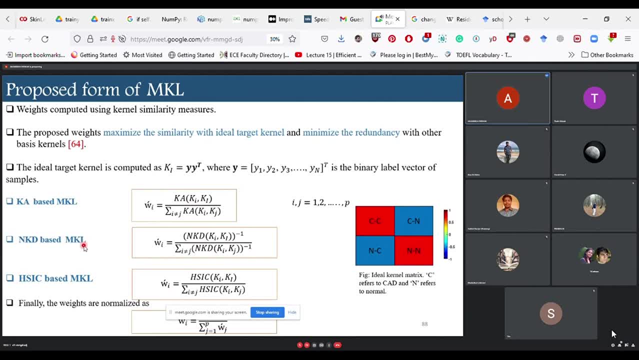 should learn and identify which should be weighted more. should they be weighted equally or with different weight metrics? so this is like main idea to maximize the similarity with ideal target kernel. so the feature or the, the kernel matrix formed with any feature should resemble more like this. but if it is redundant with other matrices it should accommodate that fact. so how to compute? 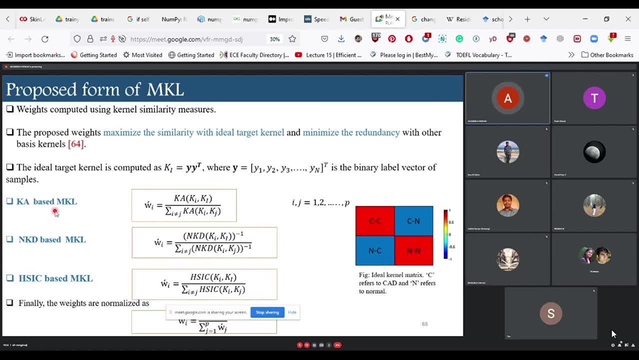 the weight. for example, i'm using kernel alignment for estimating the waves. so what i do is i compute the similarity of that kernel with an ideal kernel and divide the denominator with the rest of the kernel. so i want more inf. so numerator is accommodating for relevance and 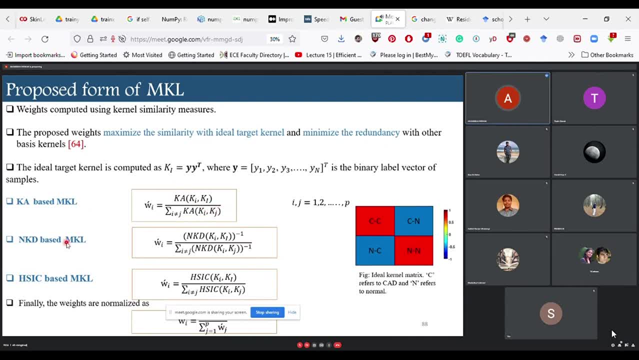 denominator is accommodating the redundancy, similarly with normalized kernel difference. also numerator is accommodating the relevance. but i have put inverse here. so if x and y is similar, so x minus y is zero. but uh, zero means more similarity. so i'm taking like the inverse of it to accommodate for the higher weightage. 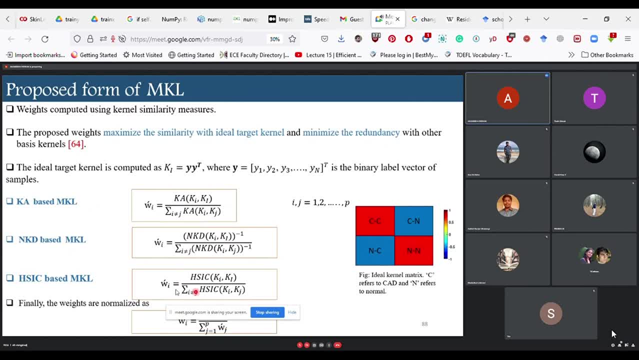 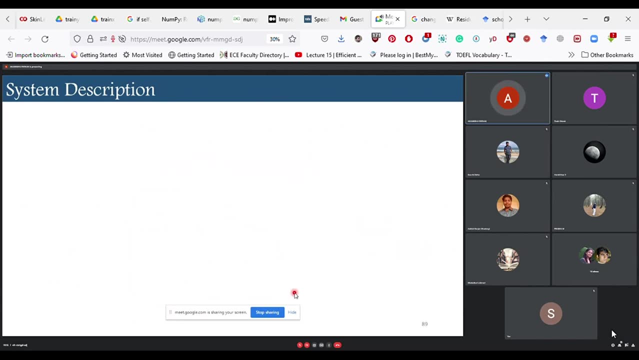 numerator and lesser weightage at the denominator, similarly hsic. so in this way i'm computing the weight for each of the kernels or the features which i am using for the fusion. so that's some of the mkl approach, not just a little like some prerequisites of using the 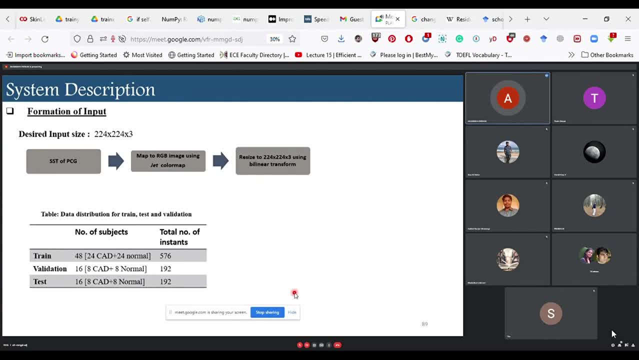 uh time frequency matrix as an input in your cnn, since you had a two dimension matrix and these pre-trained cnn is basically this they were. they are using a three dimensional input, so in such cases you can simply map the values of the time frequency representation to some rgb image using any color map of your choice. so i preferred a jet color map and then 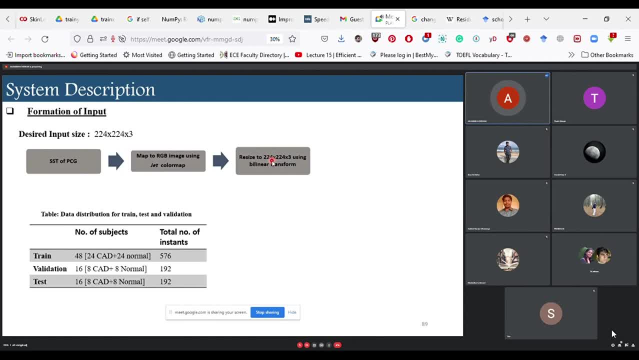 i resize it into a proper size which the cnn accept or the network accepts, using a bilinear transformation. and now, since this is like a training, a neural network, so i'm just going to. we needed some training data, testing data and relation data, and these are the parameters of 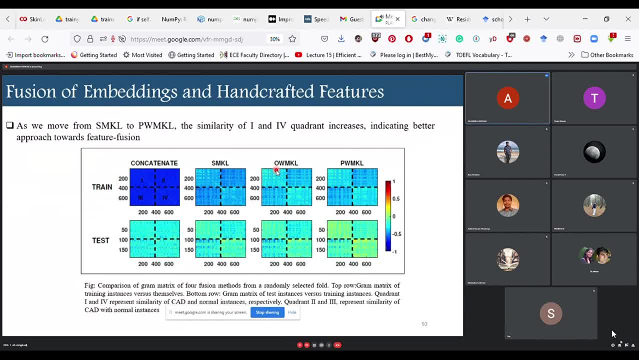 graph preparation. okay, so this is just a visual illustration of the of the kernel matrices. so concatenation is for four different cases and showing the relevance of mkf. so first case is concatenate, that is, i just concatenate all the features- shine and entropy, rainy entropy- as well as the embedding, and just use one single kernel to for uh or the kernel. 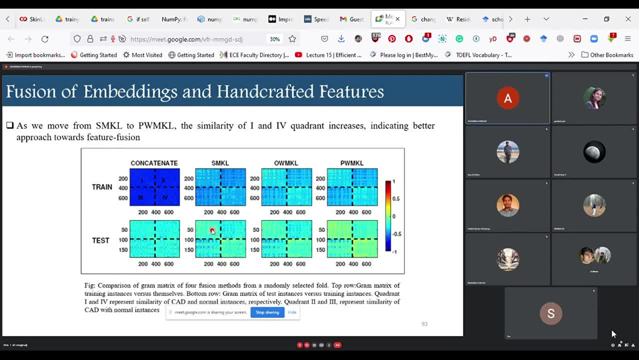 matrix to perform the classification. next is simple multiple kernel learning, that is, i'm using unit weight or the same weight for all the three matrix. next is owmkl. so this is like an approach where only relevance was accommodated in the weights, that is, they were only focusing. 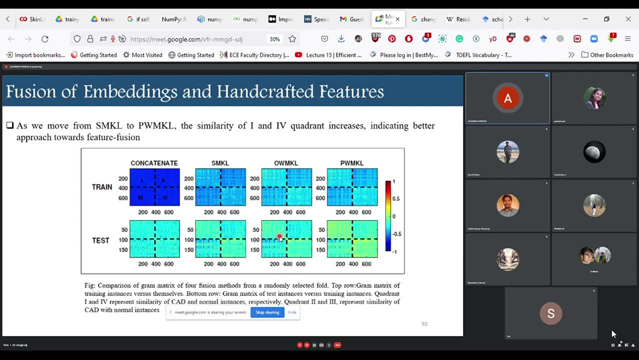 on the similarity with the ideal kernel and this is the pwmkl, which is the proposed one, where i am also using similarity as well as redundancy. so what we see is like if we see the first and fourth quadrant, so they are like going towards more prominent, like the. they are getting more. 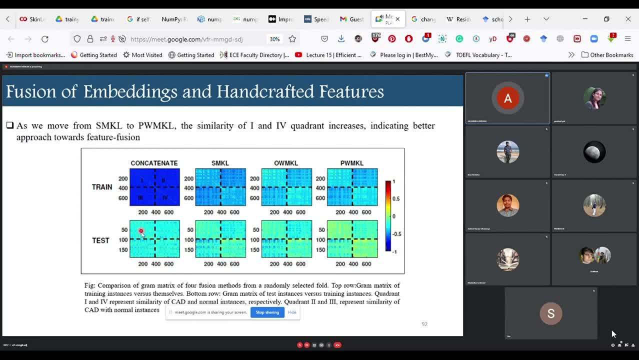 maximized, getting maximized more compared to simple concatenation case. so this is like the intuition behind. okay, why is it like that you should go for? uh? why mkl approach is better than simple concatenating the data and using a single kernel for classification? this figure is basically just the weight assignment, which 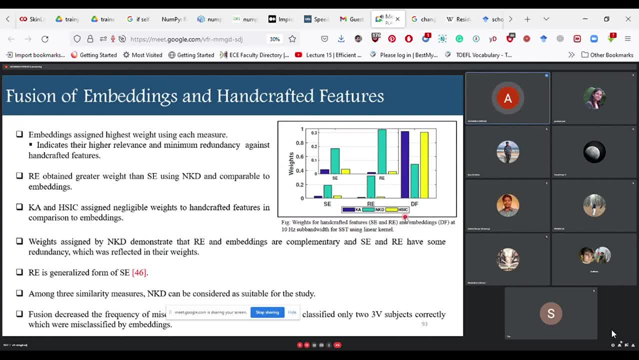 shows that. okay, how the weights were assigned using each similarity measure. so sc is shannon entropy, re is reny entropy and dm is the embeddings which are learned from the cnn. so we see all the three similarity measures assign higher weight to the embeddings, that is, they are more relevant for the classification. okay, 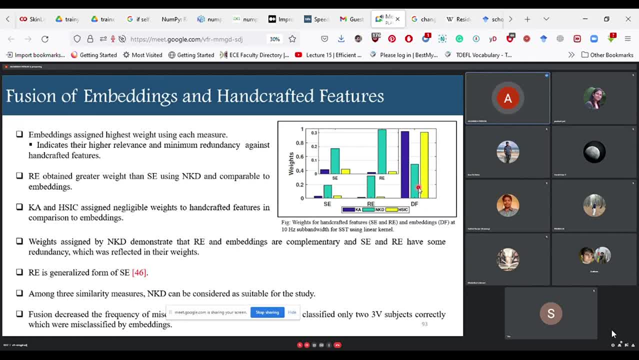 that is pretty much good, that cnn's have learned much more than the embeddings. then we see: how is the weight distribution for shannon entropy and reny entropy explicitly so? what we see is that see, as i discussed before, that these entropies are also redundant among. 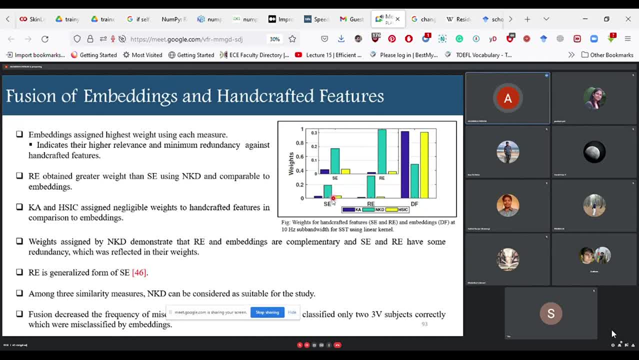 themselves, but they are also complementary. so the weight assignment shows that, okay, more weightage was assigned to reny and less weight is compared to shannon entropy. so this shows, okay, the method which i have used is accommodating these facts also, which i have learned before now. come see um. so this was like summing up all the signal processing. 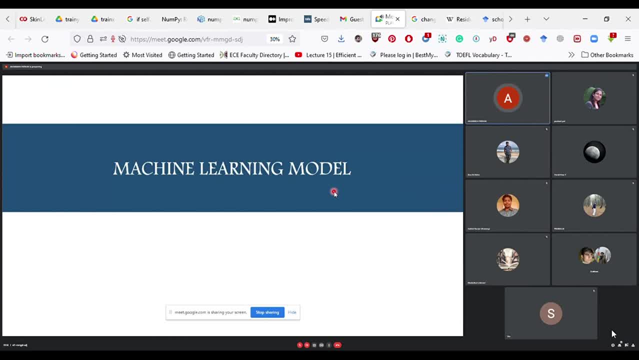 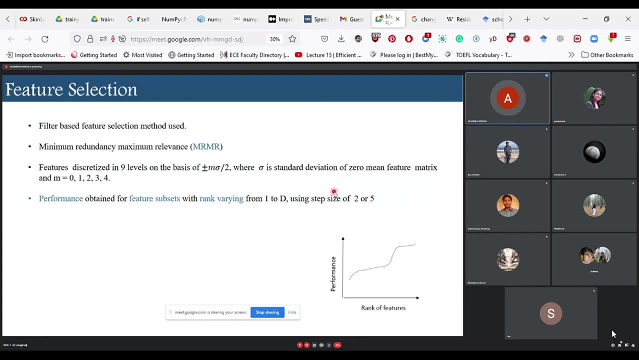 or the aspect and the feature extraction process, either hand drafted or representation for for framing the machine learning model. basically, we are left only with few main building blocks. if you are going with obviously a handcrafted approach, you might need feature selection, may or may not, but if you go it is better. so in the case, basically, 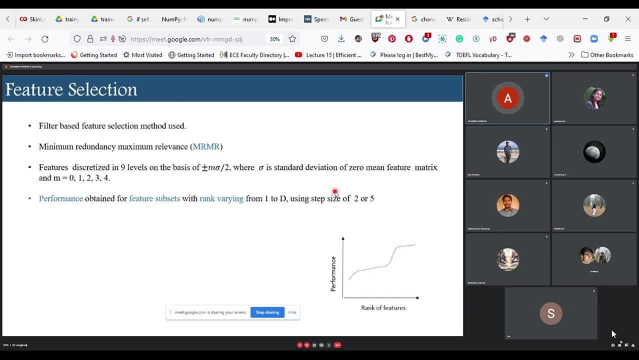 so there are multiple feature extraction methods and i would not like to focus more on them, so we have used, like filter based feature selection method. filter based feature selection method is like you just filter whatever is good for you and then just train your model so that feature selection is not a part during the classification stages, like you already filter. 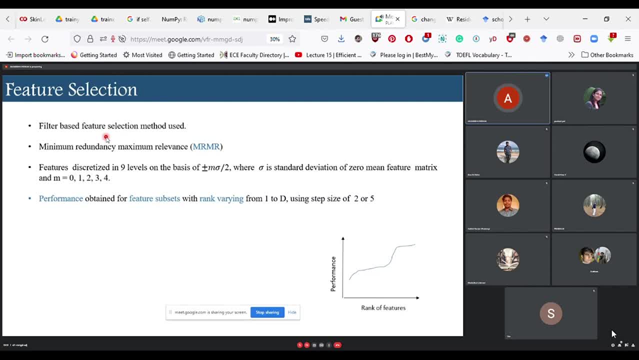 your good features, using your training data, and just use those good features in the classification. there are other methods also, like the wrapper method and the embedded methods, wherein you during the course of classification identify which features are good or bad for your performance. so here i have like used minimum redundancy and maximum relevance as a. 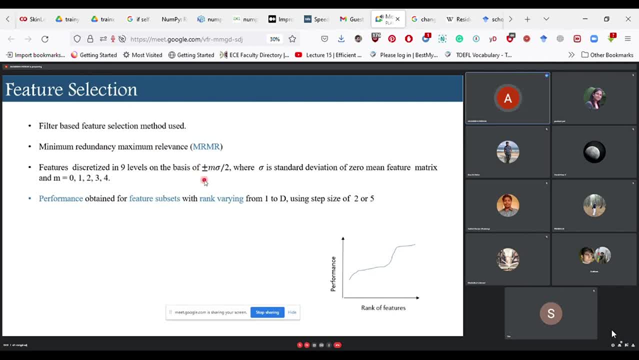 feature and these are like some prerequisites for using it. so whenever you are dealing with mutual information or these types of terms you show your data should be like more of a discrete form. discrete form is like levels. for example, if you are dealing with 0.1 to 0.2. 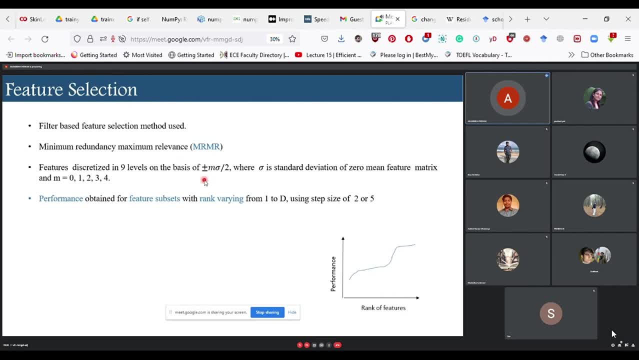 so these values would not be like good to be used in a entropy based on mutual information based metrics. so it is better that you discretize your data and divide it into some forms of levels. okay, the values in the range of 0 to 5 will be labeled as one, and so on. so the feature 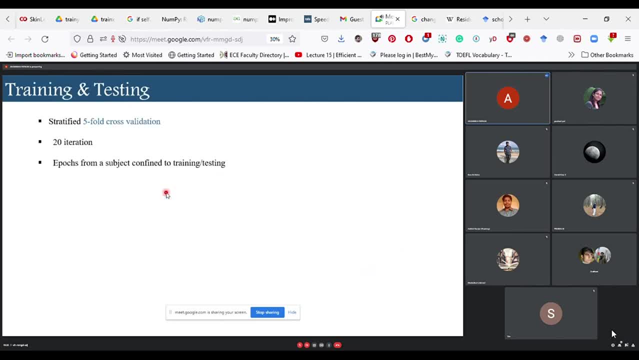 discretization needs to be done and then you get the tank. next is training and testing. so this is very essential if you are dealing with small data set. in case of large data set, one randomly takes a data as training and then testing and validation etc. but we don't have this luxury given with. 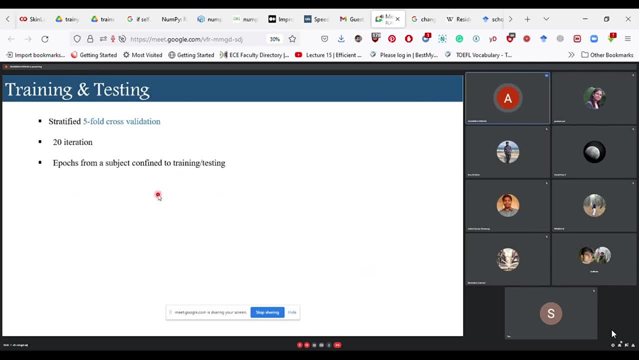 960 instances. there is no luxury that i will use 800 for training and rest 200.. moreover, this would be like a more of a biased approach like: how can you use just those fixed 800 sets? it might happen that different combinations of subjects might change your result, since 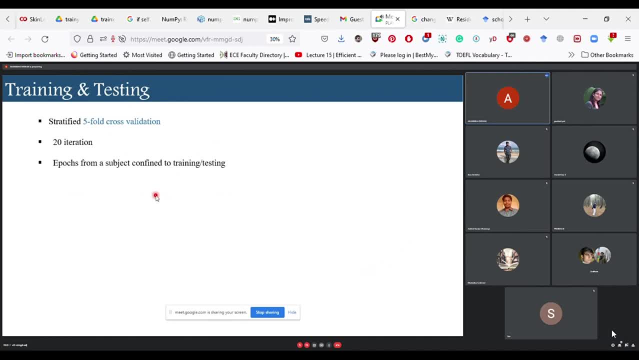 a low amount of data comes with its own biases, so you need to be, like, very impartial towards the training subsets you are forming as well as the testing subsets you are using. okay, so what we? what a good approach is to use a cross validation approach and even like 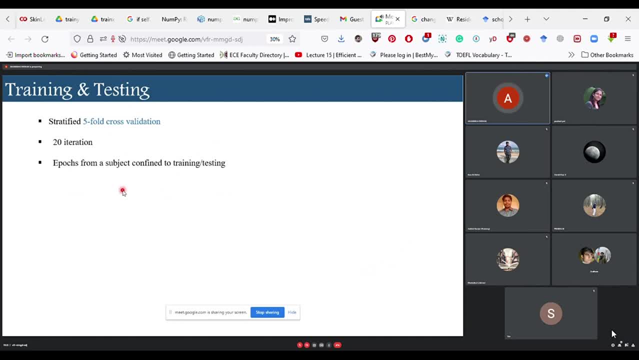 i trade it for different iterations. so, for example, i have divided my data into five folds, but i have done it like 20 times and in each iteration i have divided my data into five folds, and in each iteration i have divided my data into five folds and in each iteration 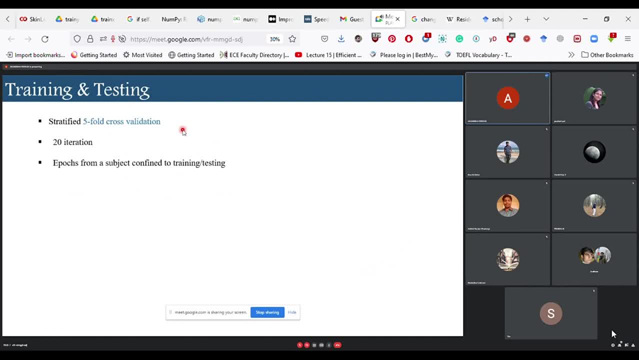 i'm taking different divisions of the five fold. so this is like i'm expanding the number of iterations of my test, training and testing. so it is like i'm testing 100 times with different combinations of subjects or epochs so that i don't get any sort of bias results. but however, 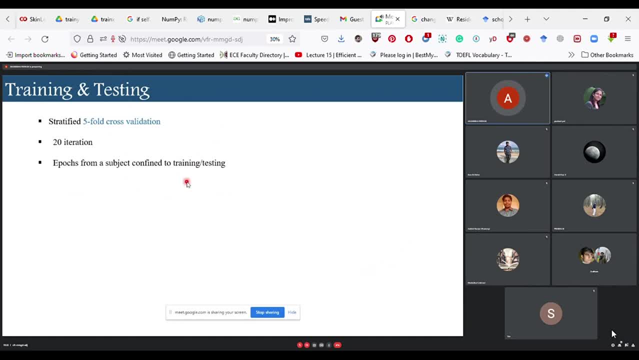 punch it with in medical domain processing, which should be kept in mind is that if you are using epochs, so you are using a different combination of subjects or epochs. so that you are using epochs so you are using a different combination of subjects or epochs. so that you are using a different combination of subjects or epochs, so that you are using a different. 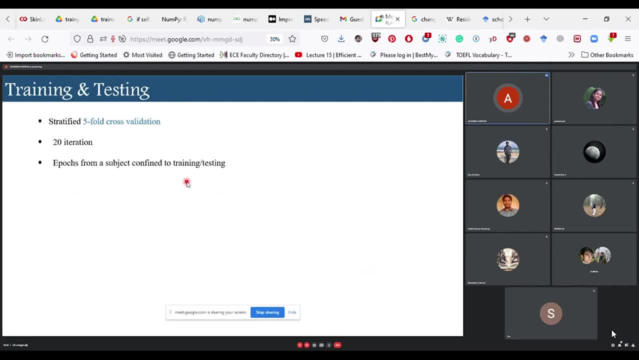 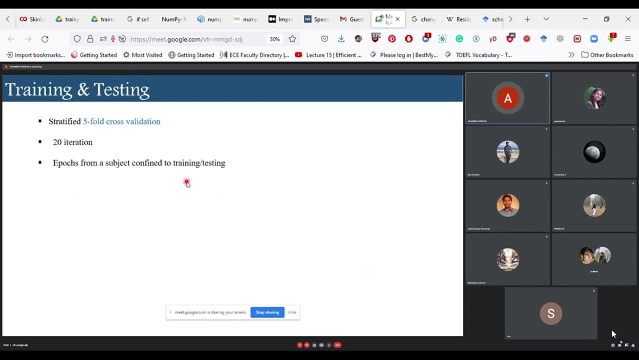 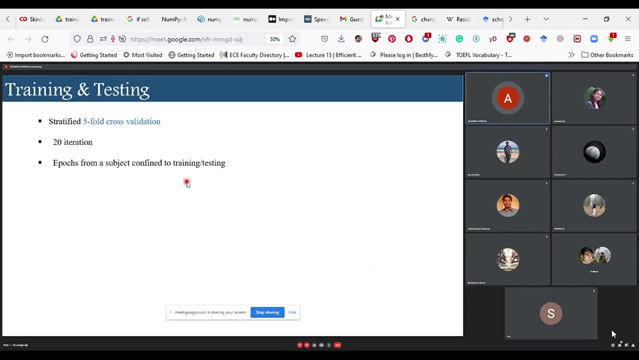 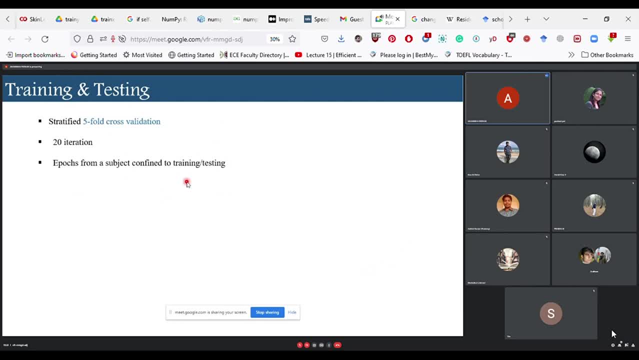 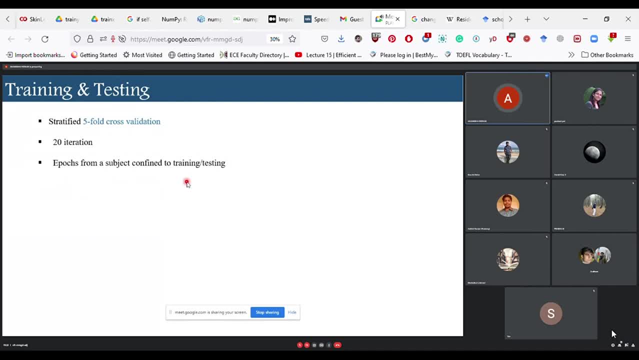 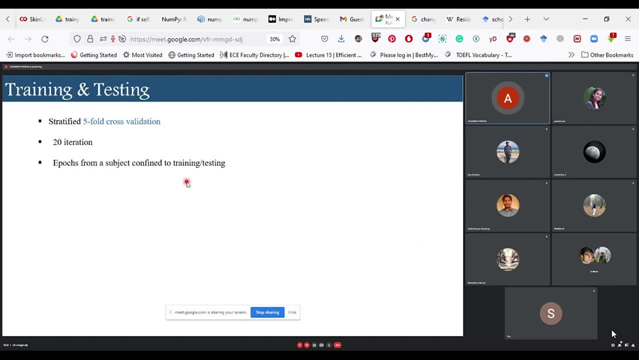 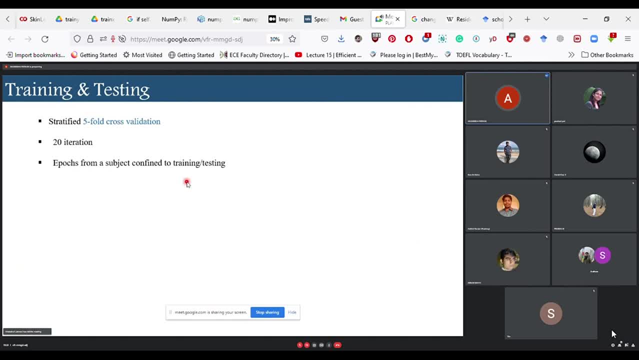 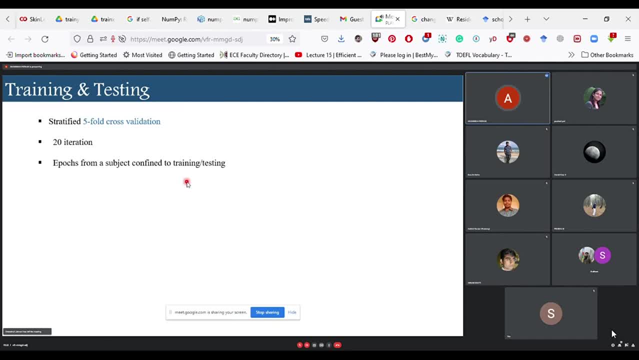 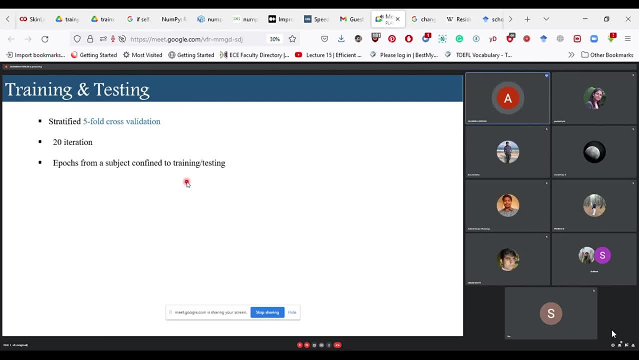 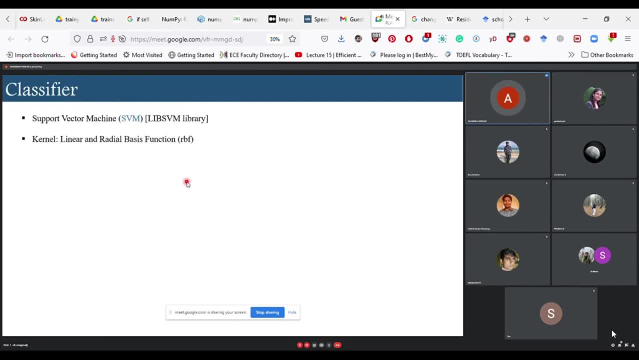 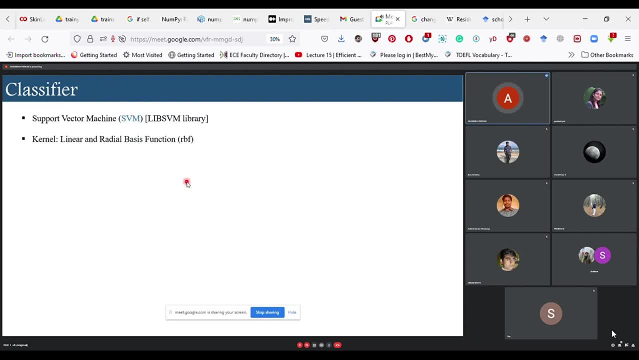 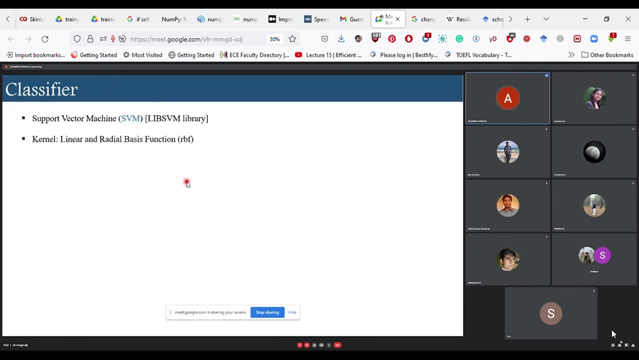 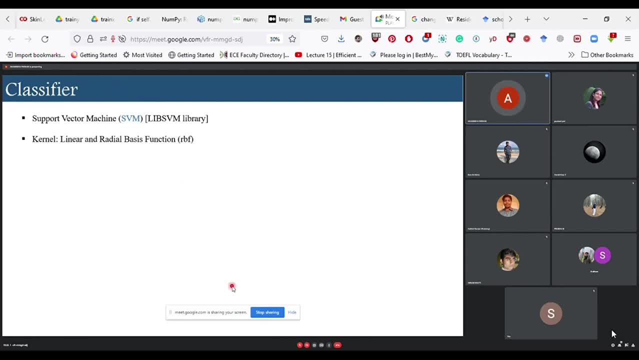 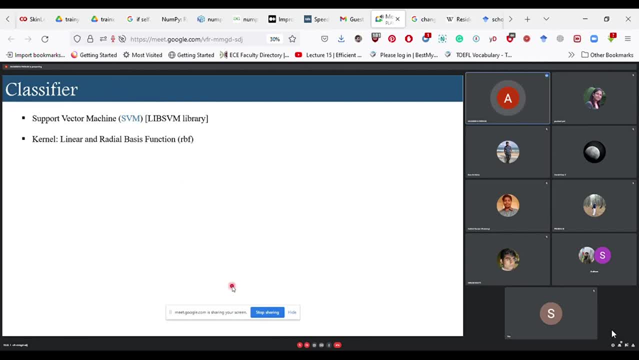 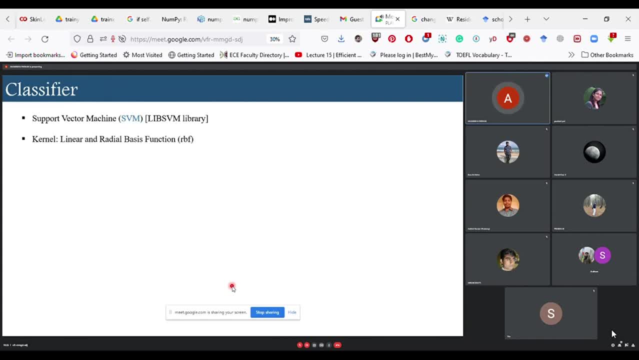 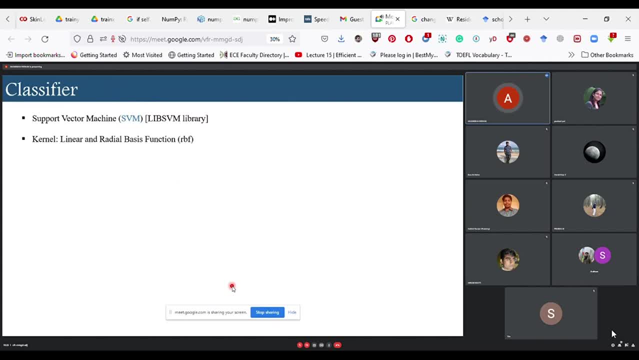 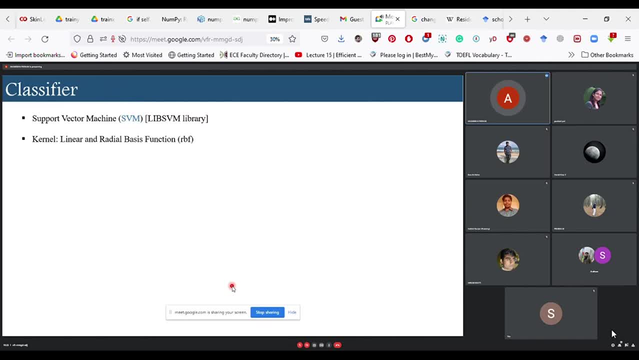 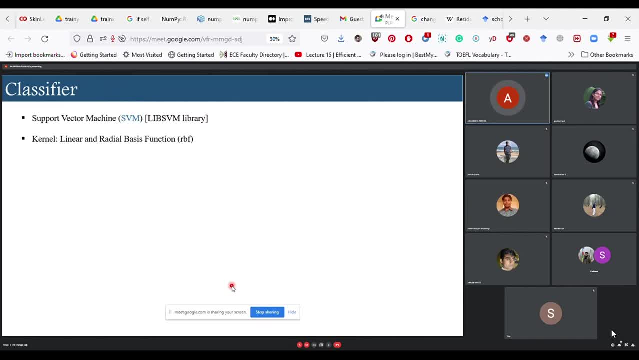 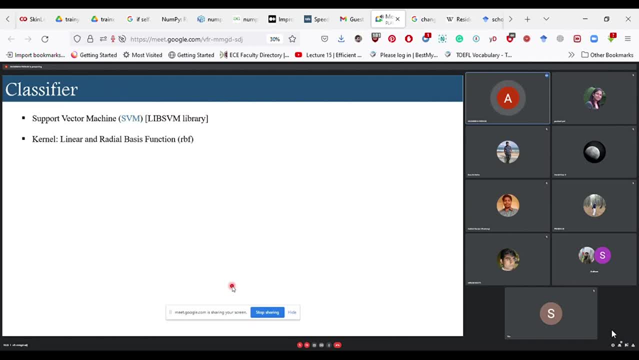 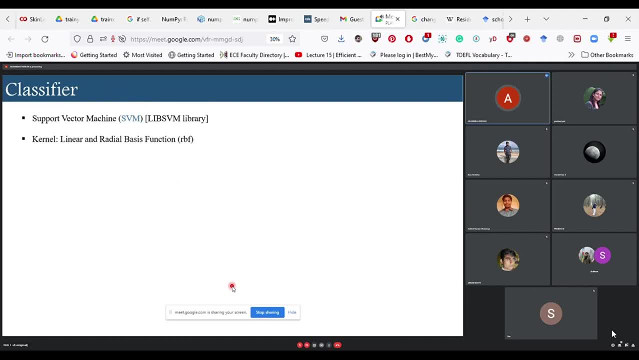 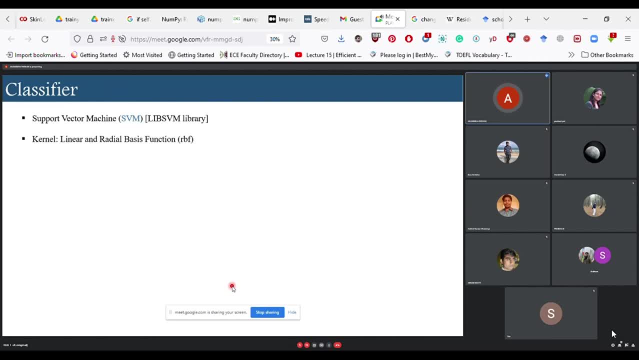 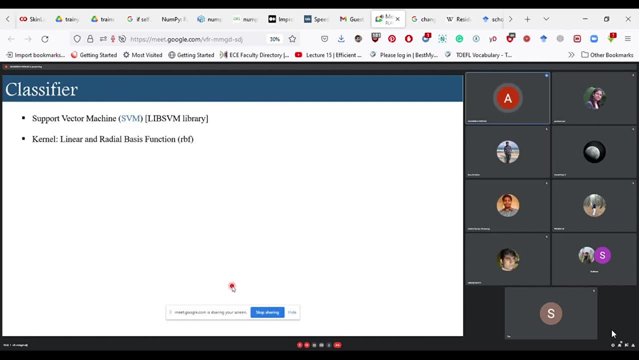 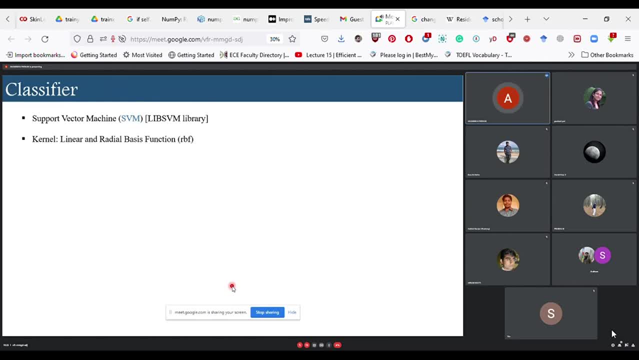 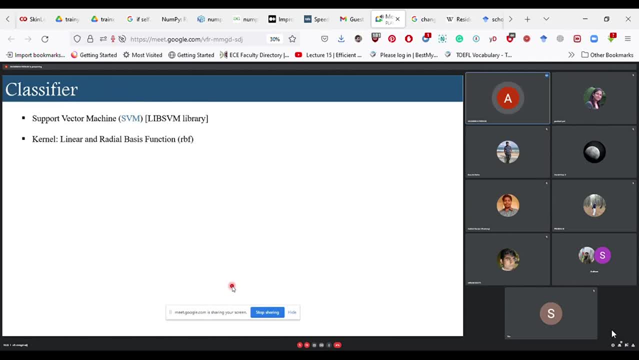 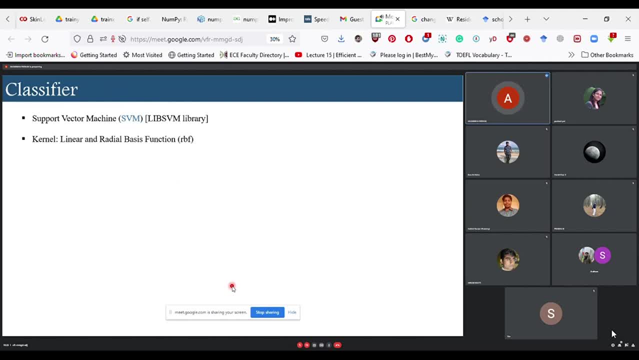 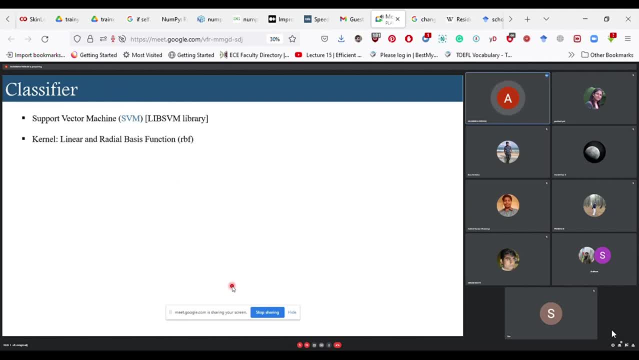 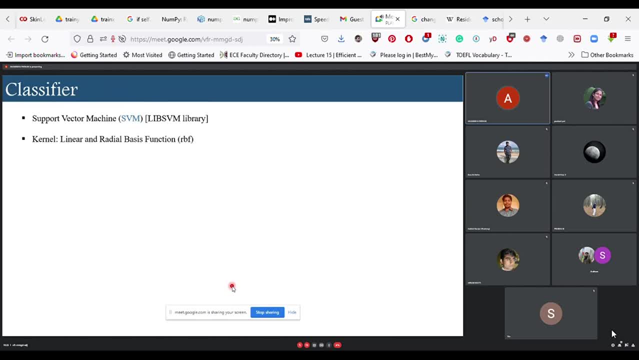 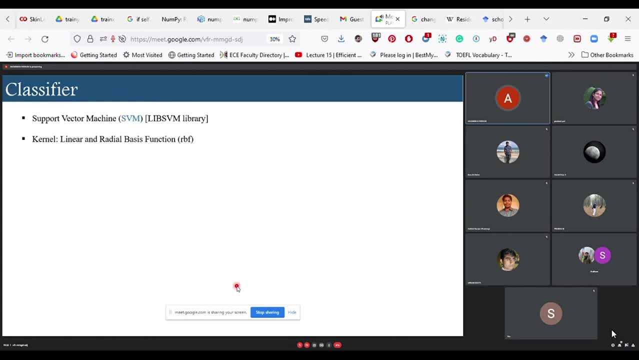 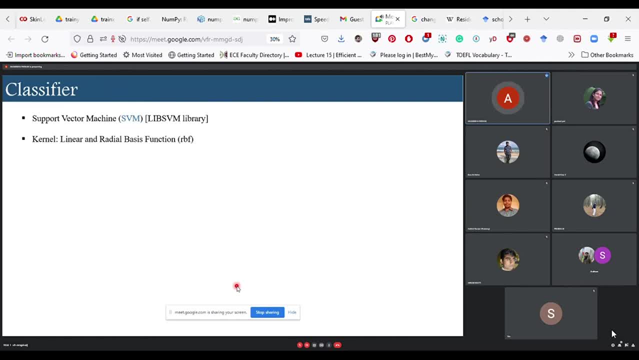 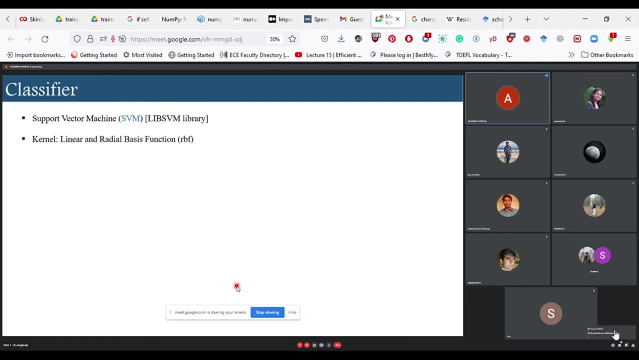 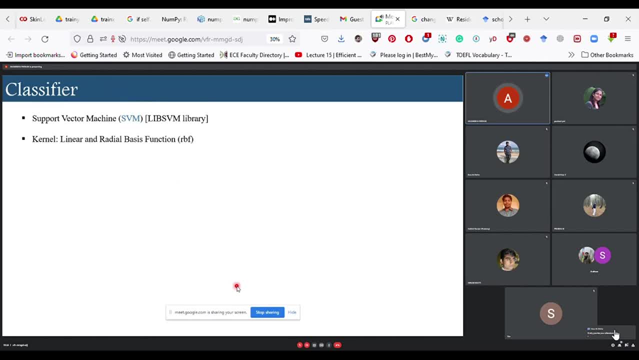 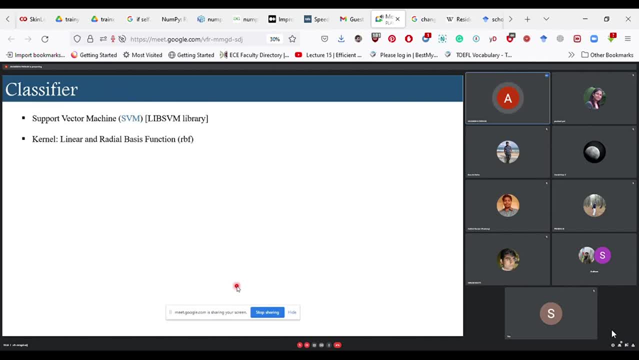 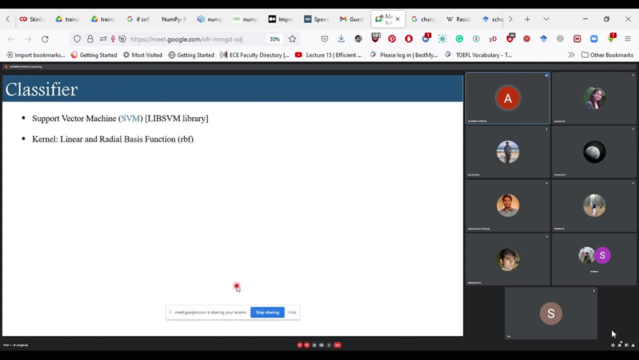 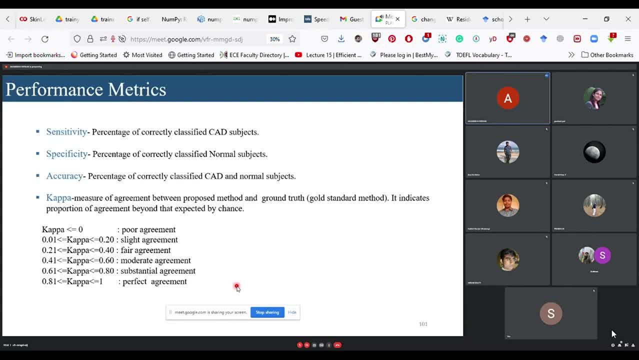 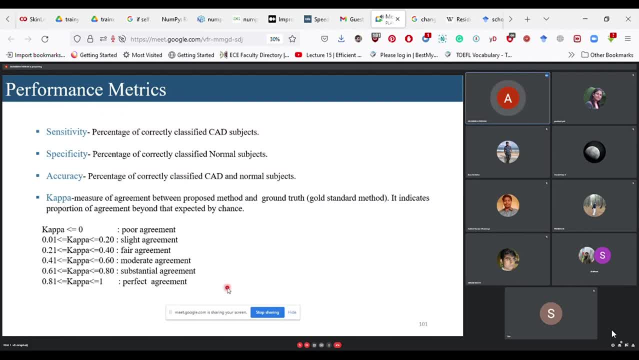 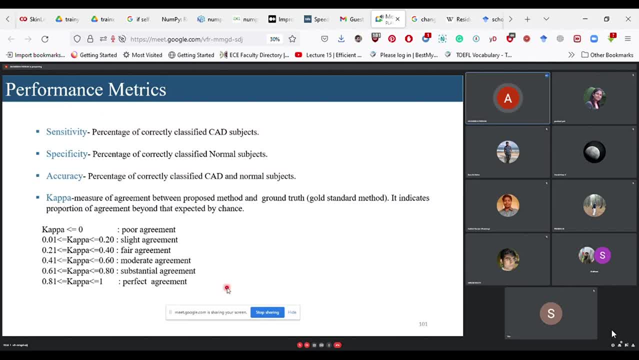 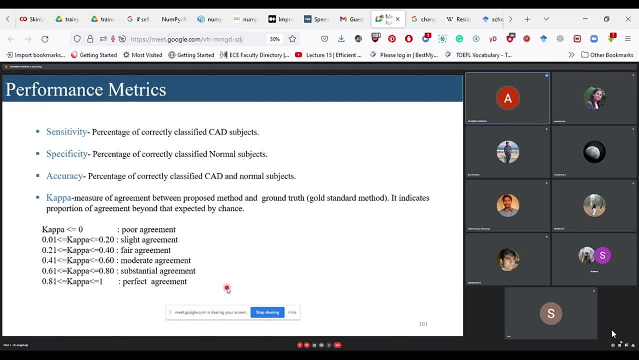 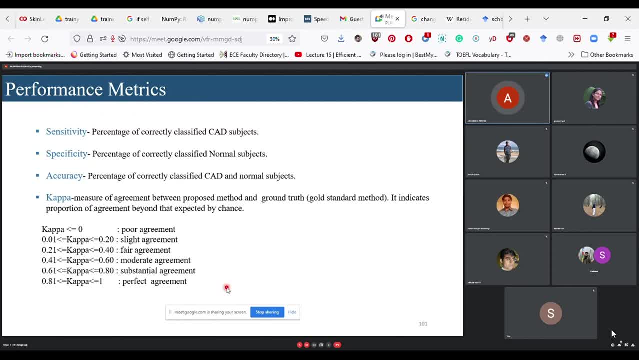 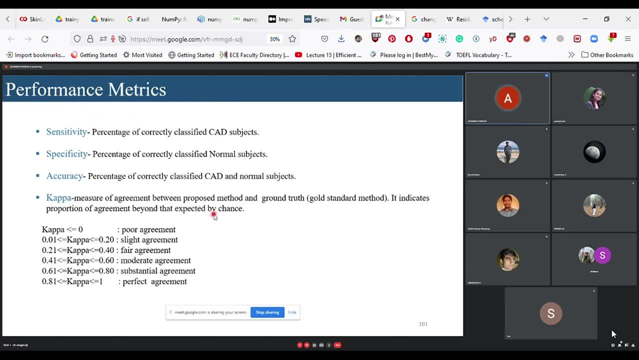 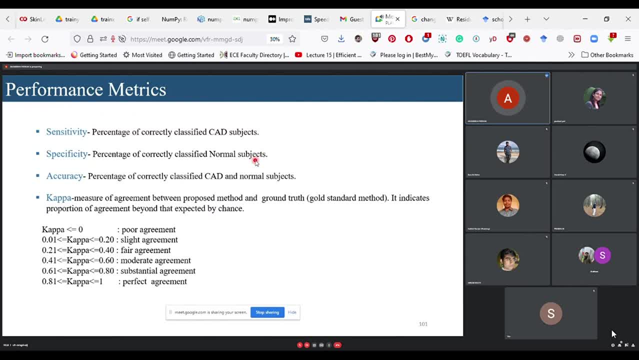 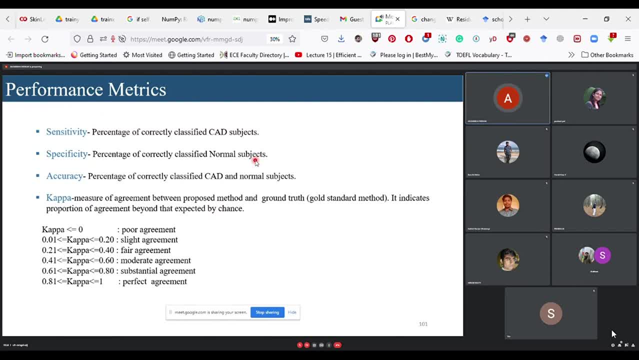 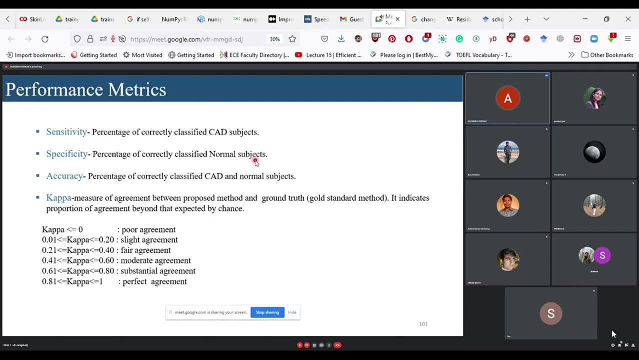 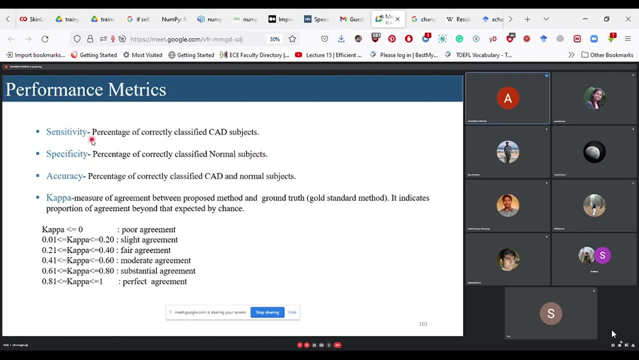 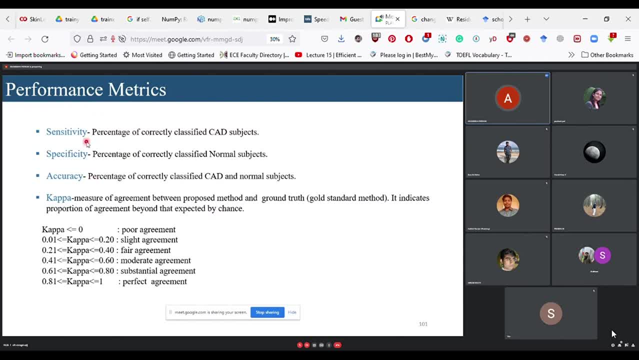 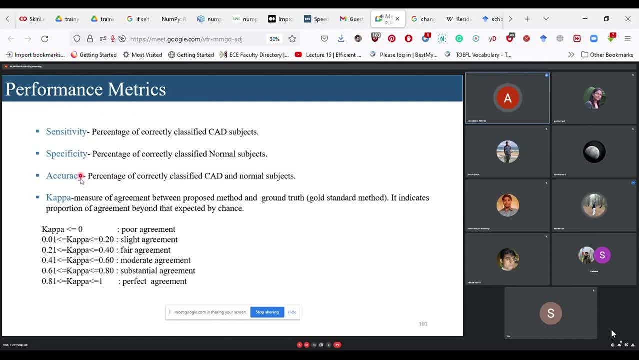 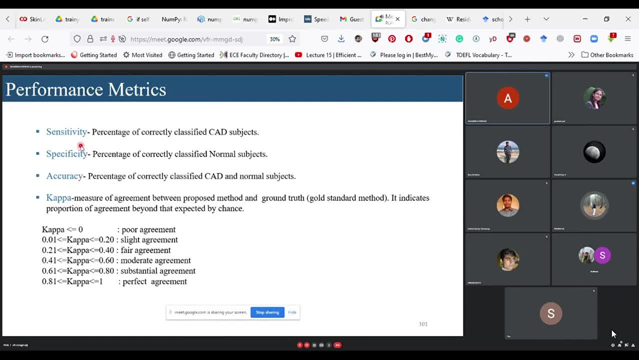 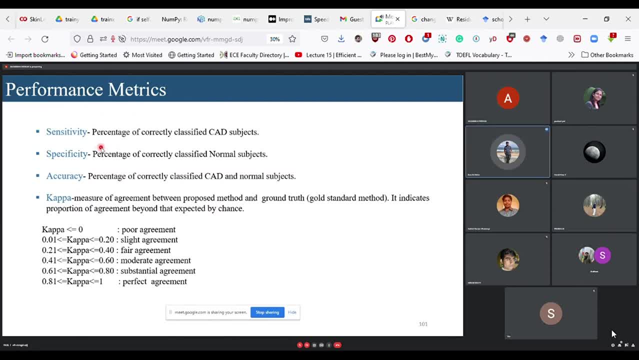 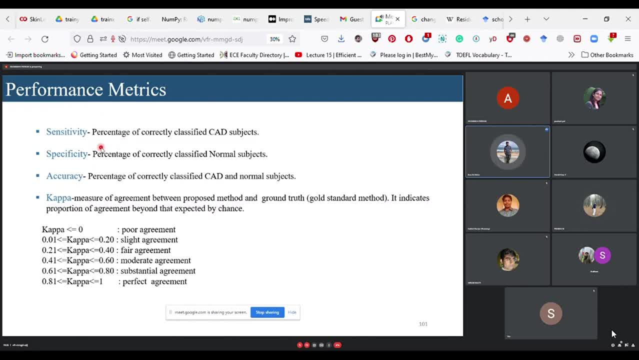 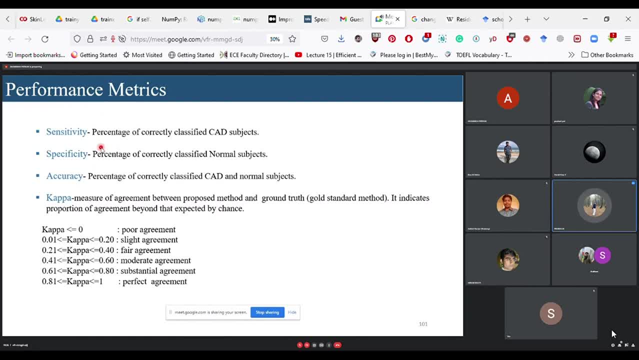 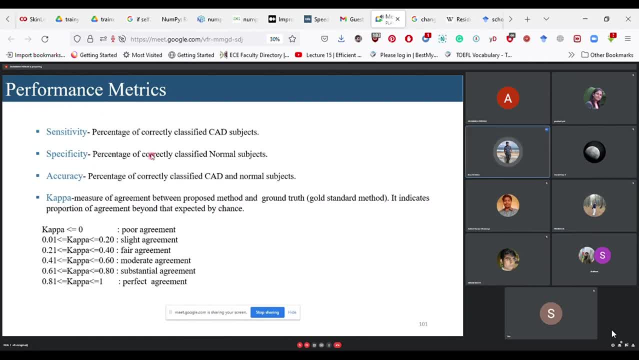 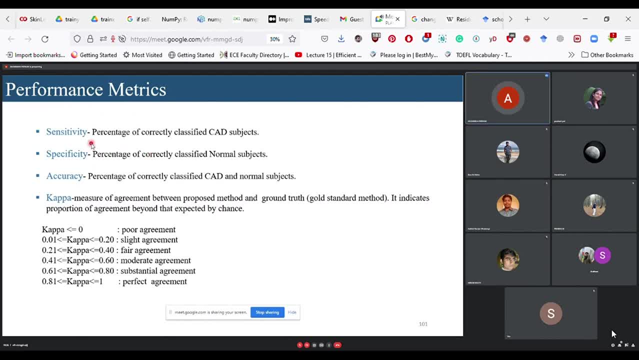 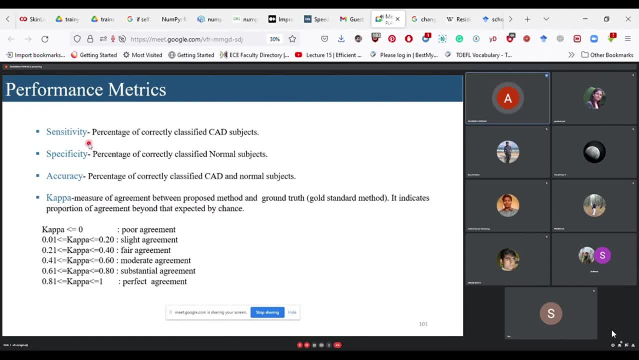 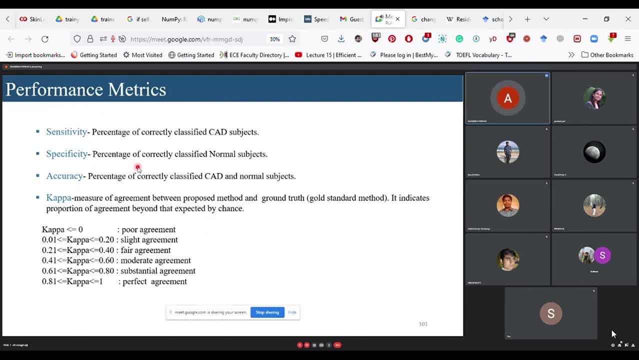 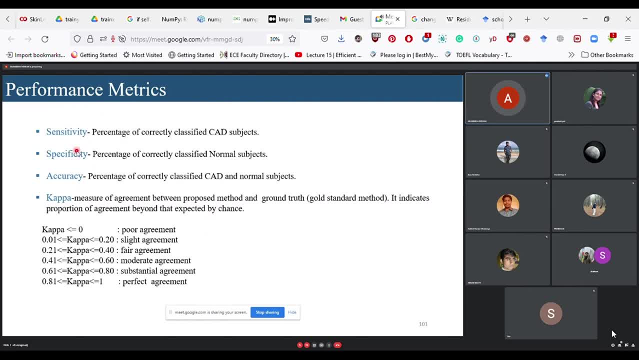 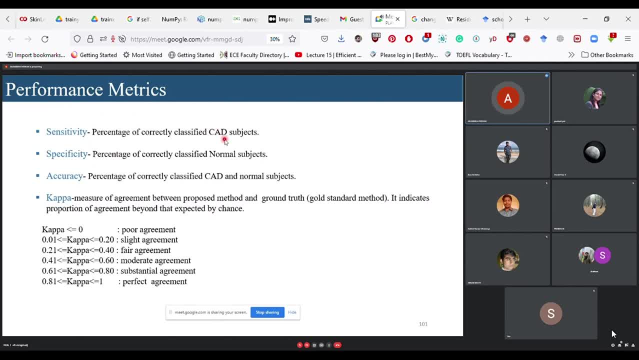 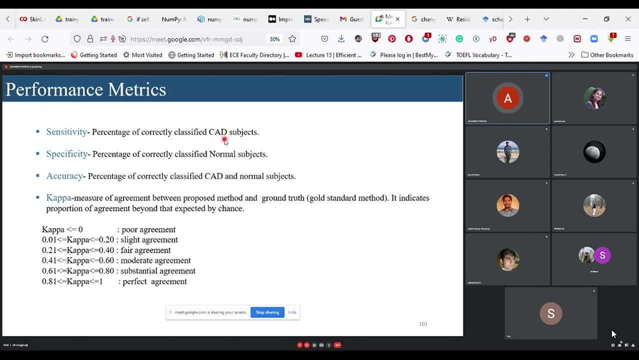 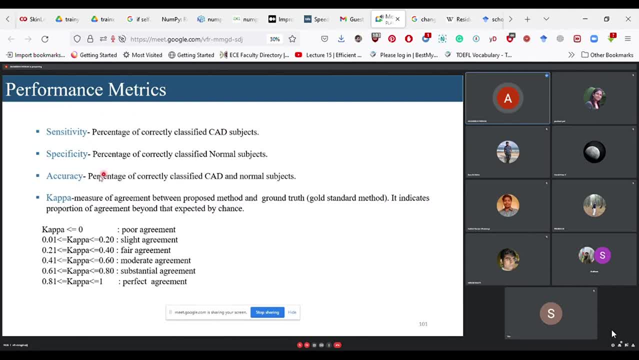 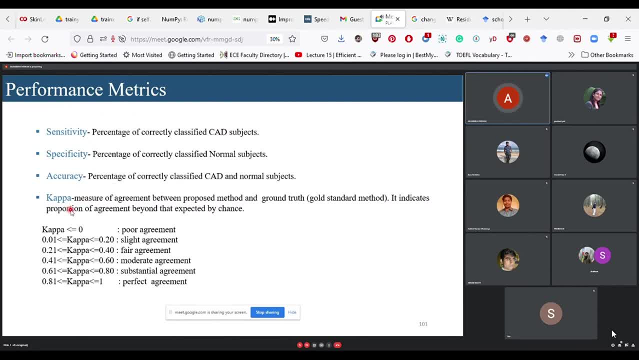 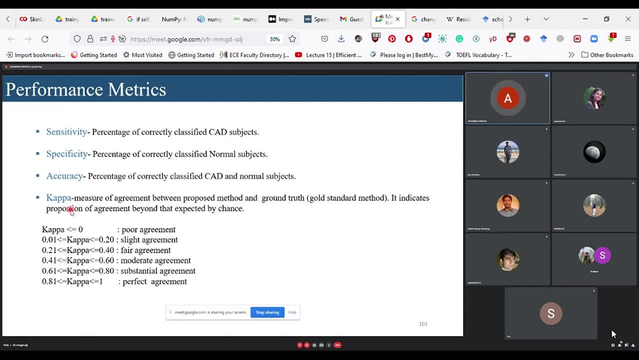 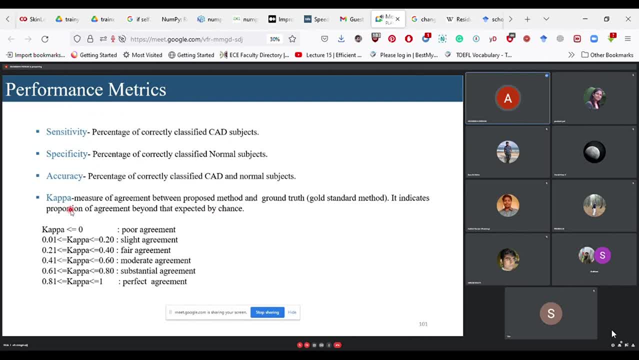 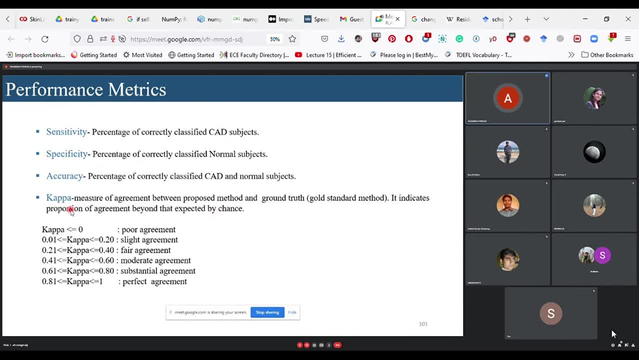 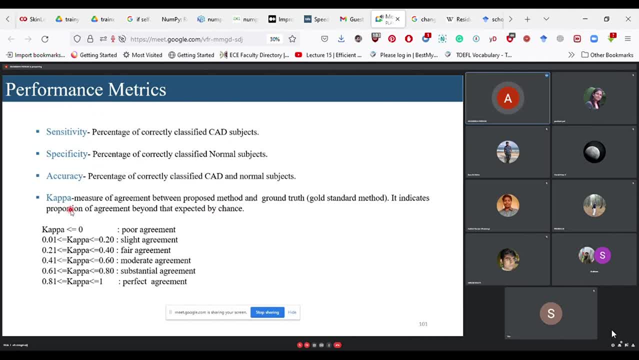 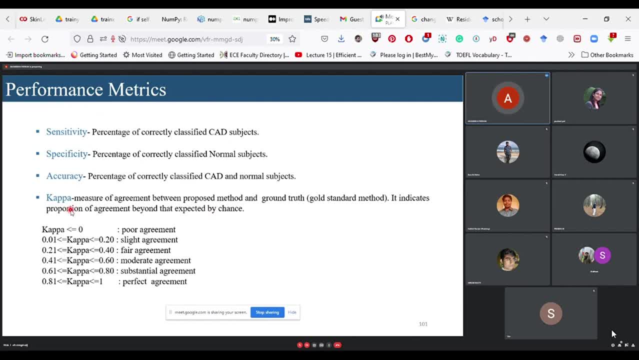 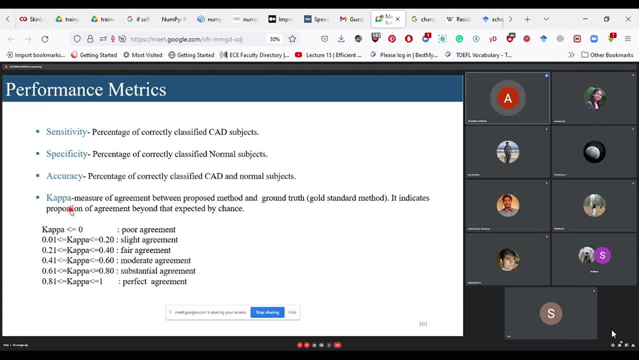 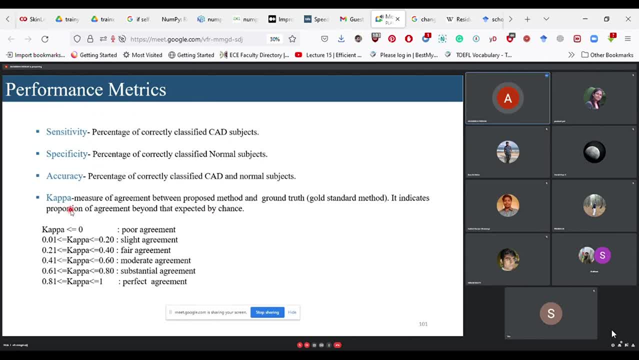 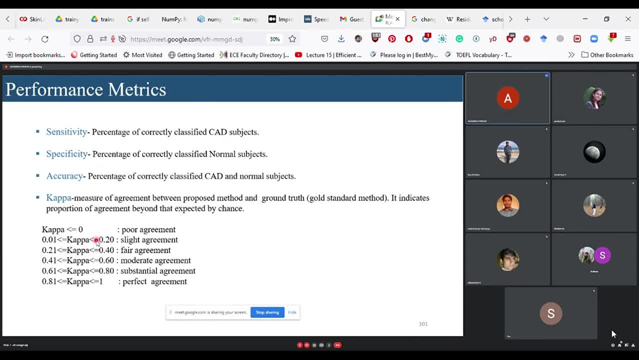 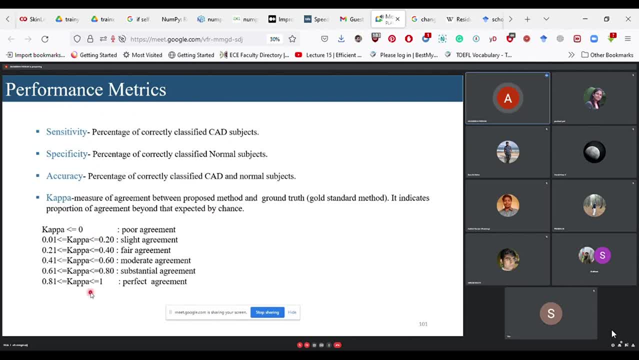 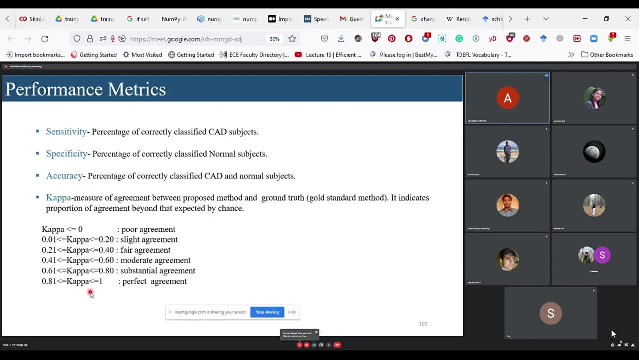 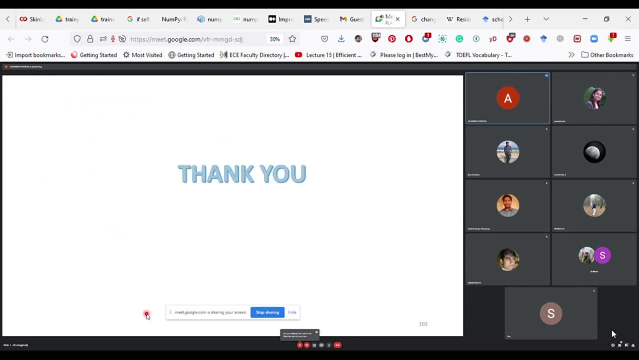 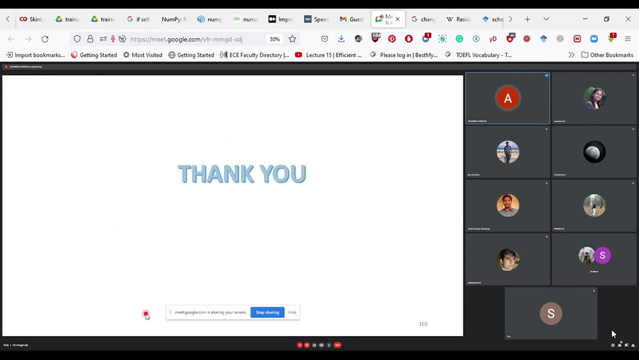 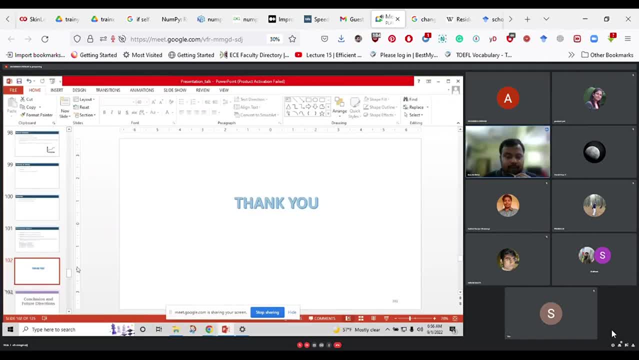 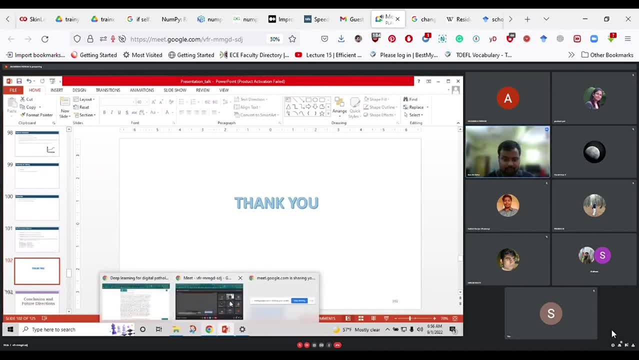 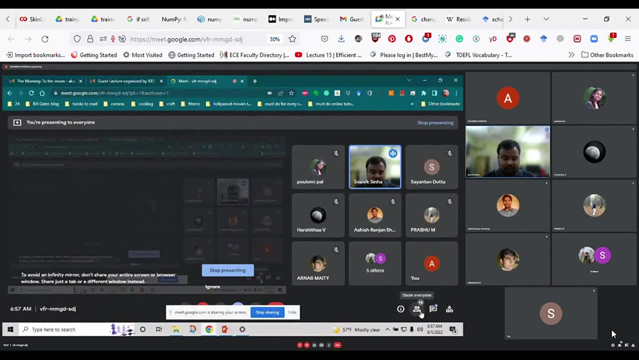 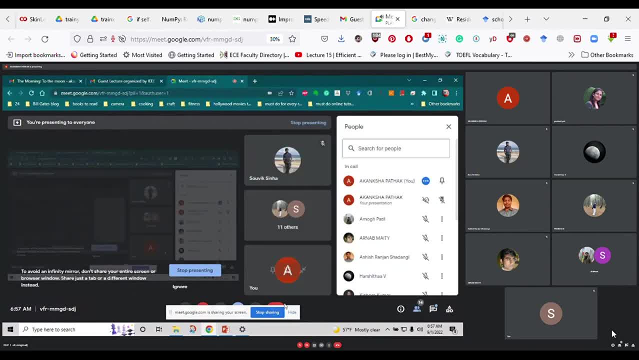 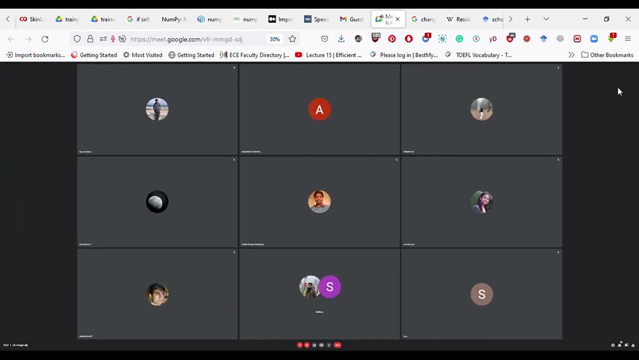 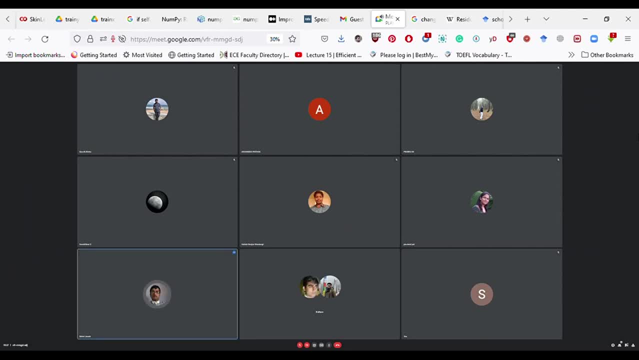 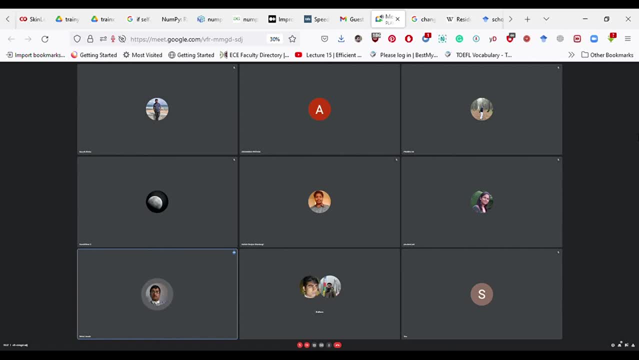 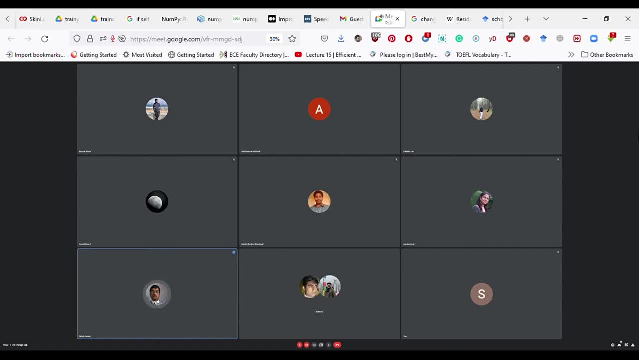 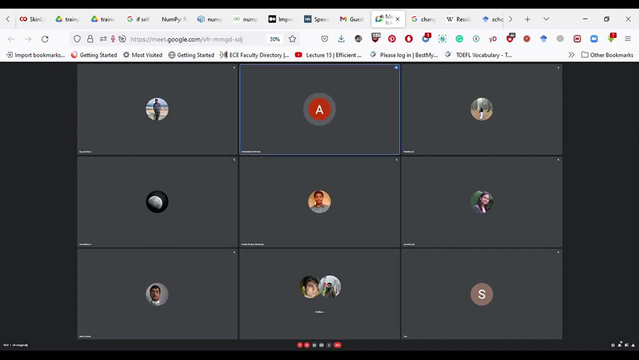 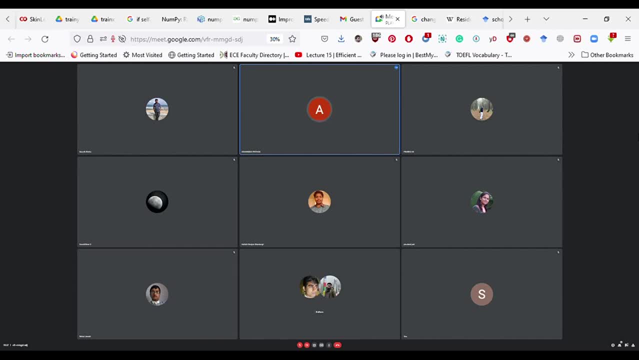 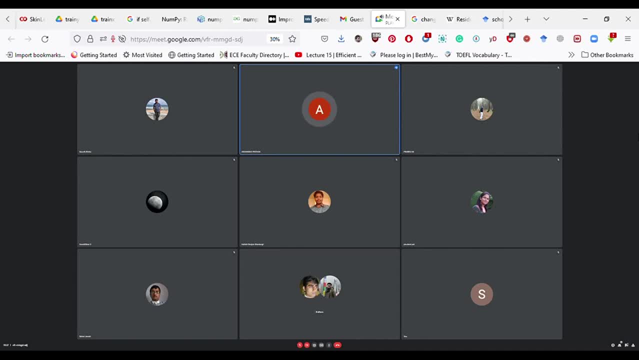 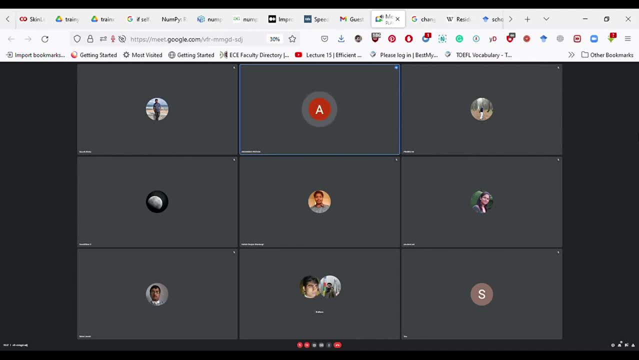 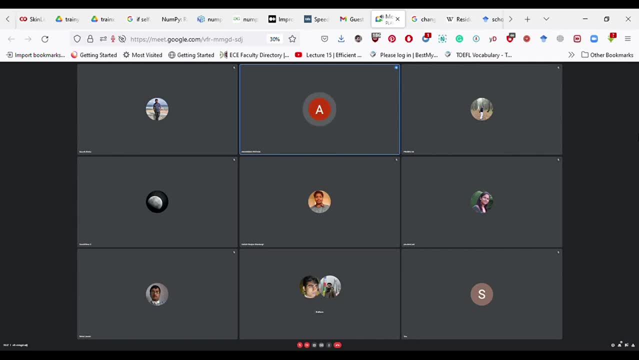 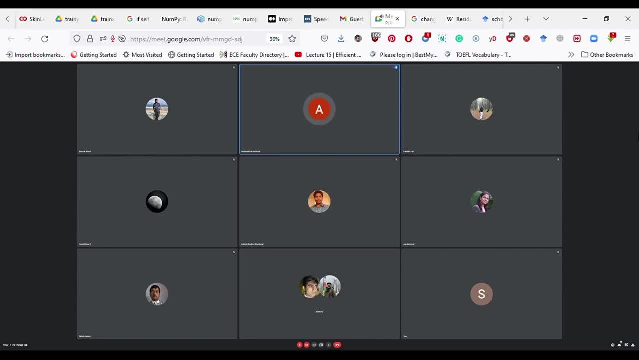 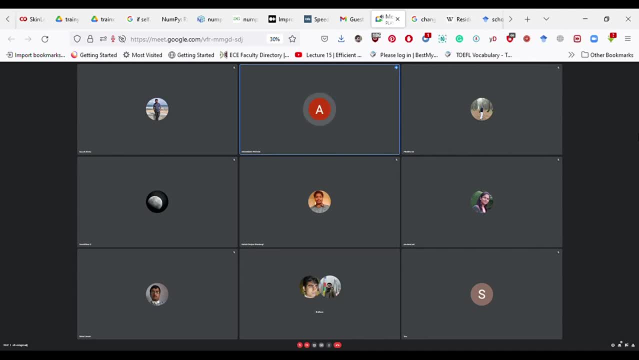 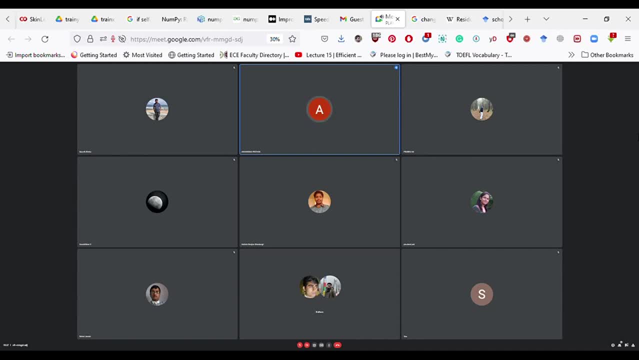 we are using less sort of color range. so this is like an intuition that you should go for a color map which has more color gradients. so it helps. the extractor, or the general know-how, is also the based on the same. you will look more for color gradients if you are working on such problems. so better to have more. 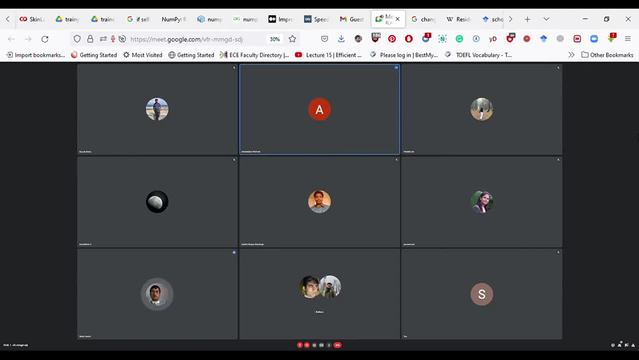 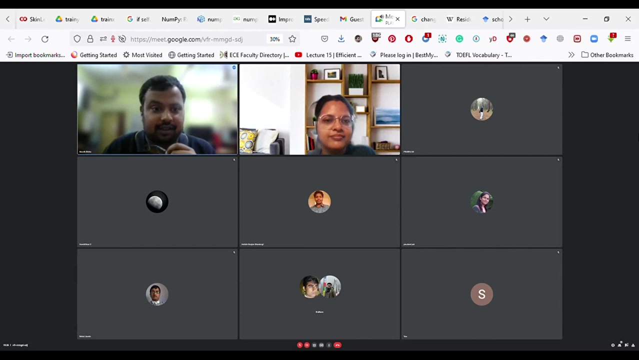 ranges. okay, thank you very much. now, any more questions from anyone else? please go ahead. okay, seeing that there are no more questions, I would like to provide the concluding note. so firstly, I would like to extend my heartfelt thanks to Akanksha ma'am for taking out time from her busy schedule. 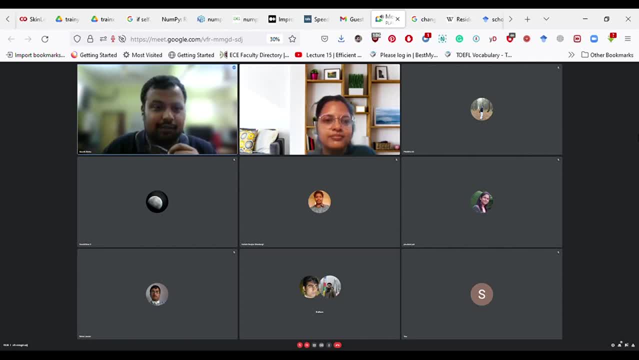 and preparing this fantastic presentation for us. it was very detailed, and not only did we come to know about her research expertise, but we also came to know about the workflow that needed to need to be carried on in order to make a very established research. so thank you, ma'am, for that and also for 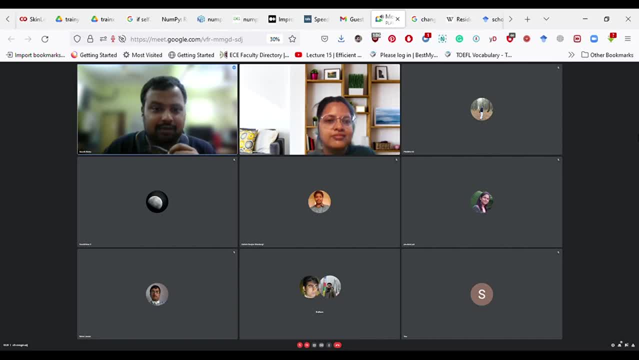 delivering your speech at a time which is very early in the morning at your place. thank you for inviting me and having me here. it was a good experience, like though we have given presentations before, but giving the same topic presentation to a crowd which who is not, that was expertise.